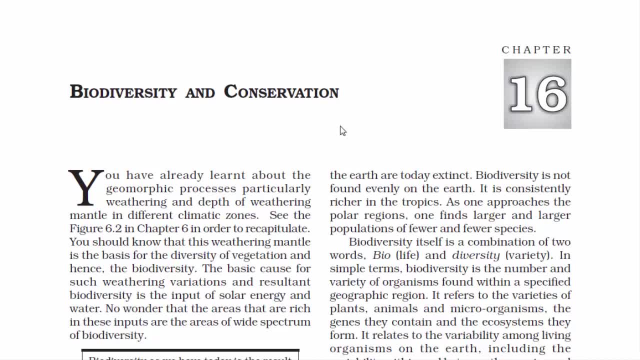 For those of you interested in watching specific parts of this video, check the description for timestamp links. You can click on a specific time and fast forward to the part that you want to watch. For others, let's begin with the chapter Chapter 16, Class 11, Biodiversity and Conservation. 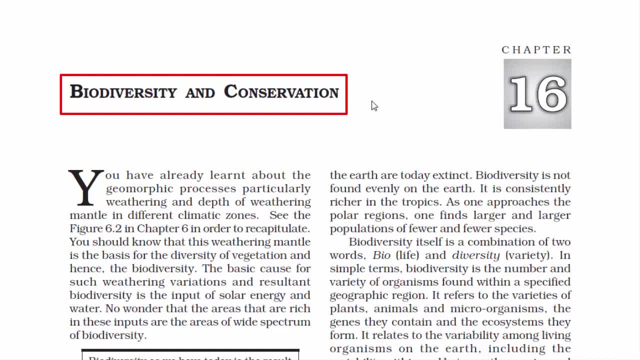 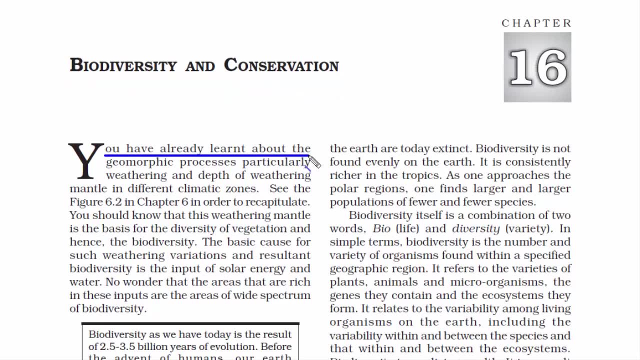 This marks the last chapter of this book: Fundamentals of Physical Geography. Alright, then let's begin with the chapter Now. here it says you have already learned about the geomorphic processes, particularly weathering and depth of the weathering mantle in different 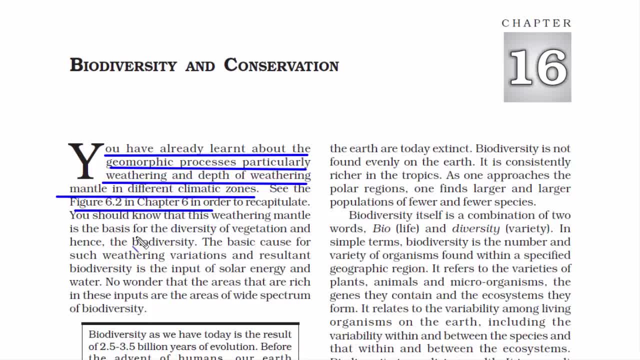 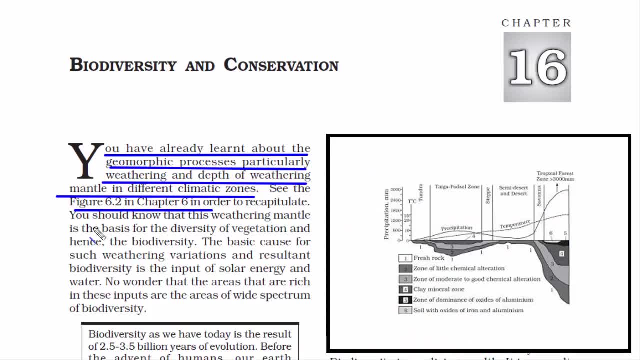 climatic zones: See figure 6.2 in chapter 6.. So chapter 6 is geomorphic processes and we need to look at this picture. It's fairly easy to understand this picture. Let me quickly describe it. From left to right, it's showing the gradual pattern of the earth's crust, If you remember. 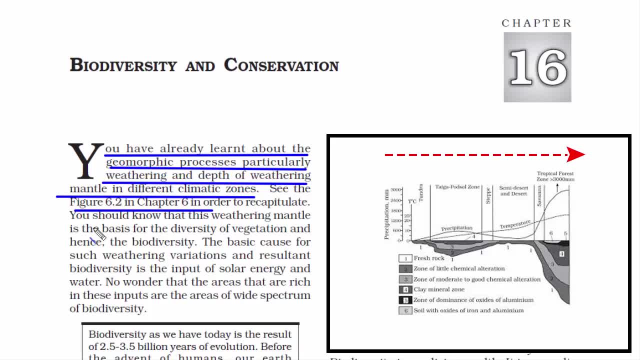 this picture different zones of earth. we have frigid zone, torrid zone, torrid zone. Even this picture is the same as this one. I just need to turn it 90 degrees and it's the same picture. The left side represents the landmasses of cold tundra polar. 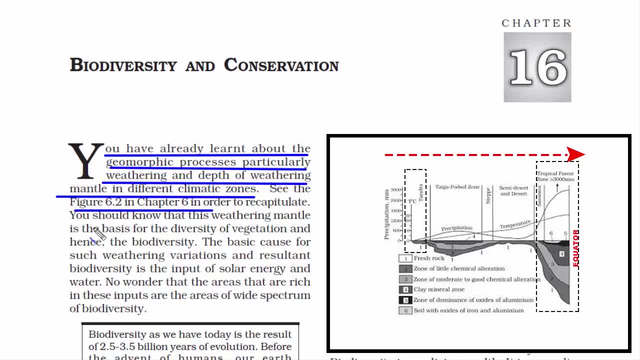 region and the right side represents the landmasses of warm tropical equatorial region. You can also see the temperature and the precipitation graph going low to high from left to right. The alternative explanation is that as we go away from the earth, the temperature and the precipitation 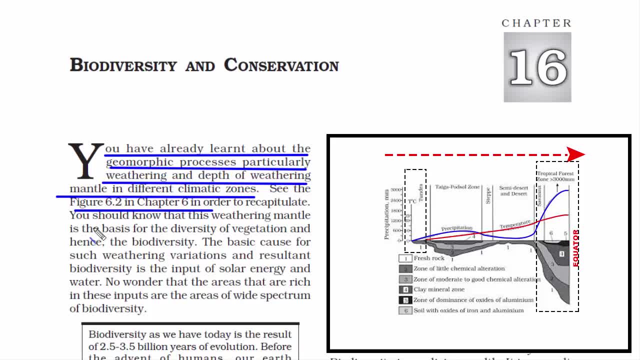 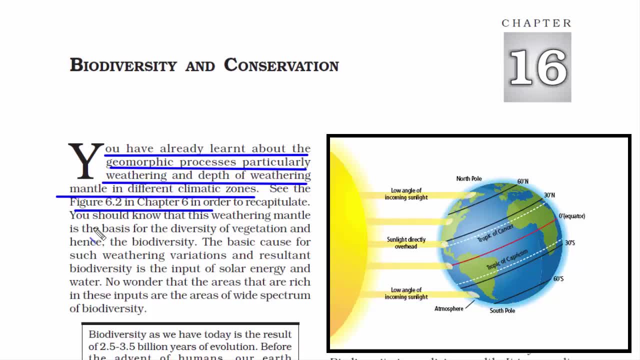 in the equator towards the pole area, temperature as well as precipitation decreases, And the most important reason behind this phenomena is the input of solar energy and water. At the equator, the sun's rays are the most direct on earth. As you move towards the poles, the sun's angle in the 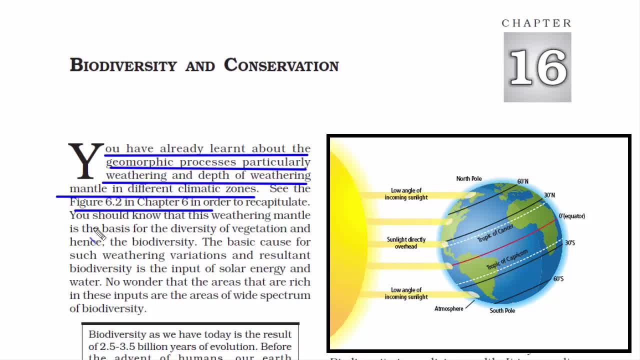 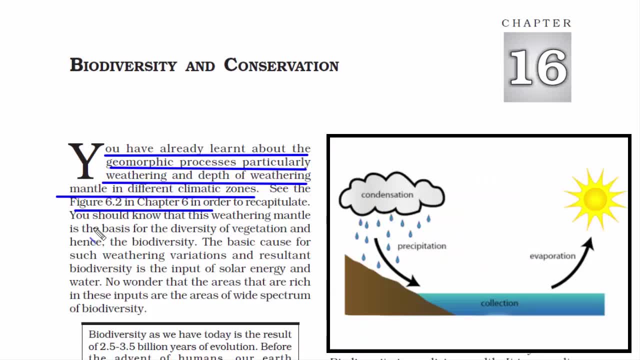 sky decreases and that affects the incoming solar intensity. Now the thing about precipitation is that it takes place only if there is evaporation. So if you move towards the equator, the sun's rays don't would not be considered as evaporation. An evaporation relies on warm temperature. 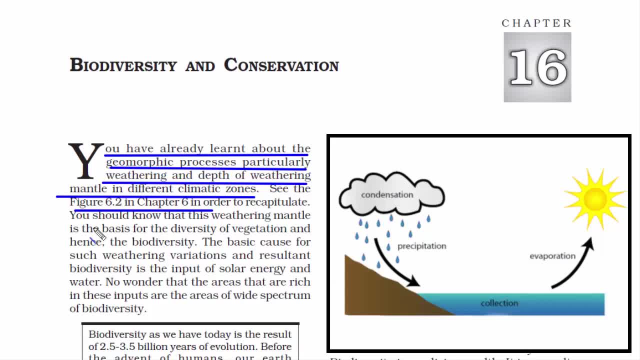 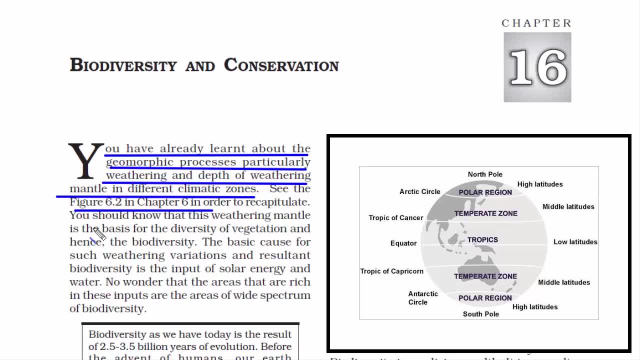 in other words, solar energy. That means tropical equatorial region is a perfect place that is both warm and wet, Which is perfect for the existence of wide variety of biodiversity. If you look at the biodiversity hot spots in the world, everything exists in the tropical region. 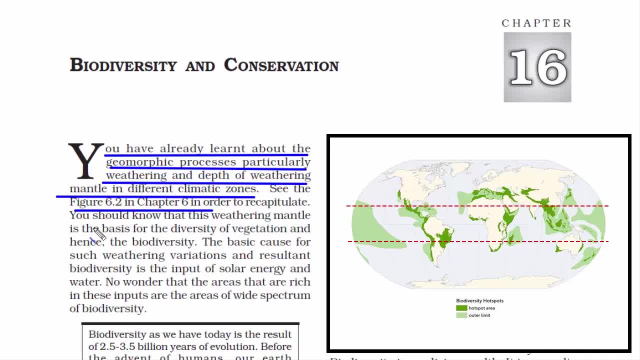 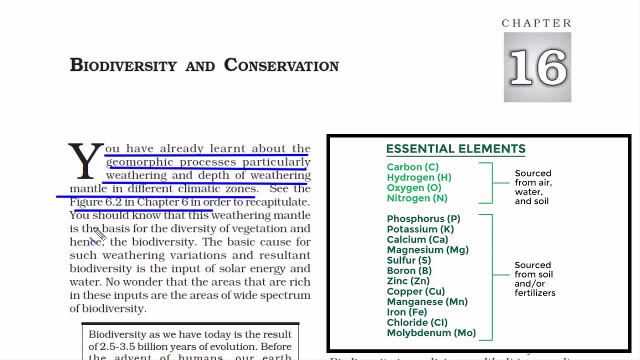 That means temperature. wise tropical region is ideal for the existence of a wide variety of vegetation, But don't forget that trees and plants need some essential nutrients, which they only get it from the soil. Some nutrients that plants need are nitrogen, phosphorus. 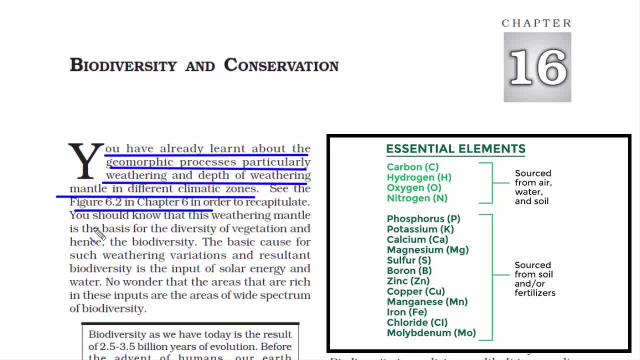 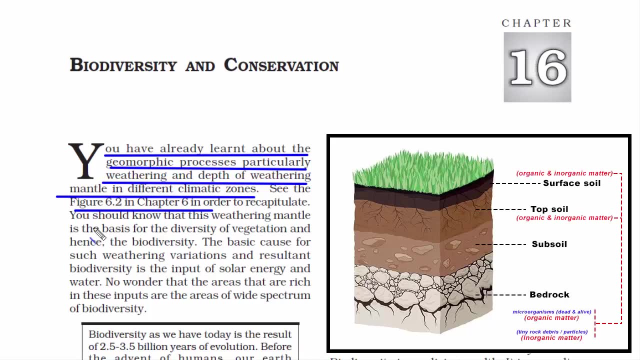 potassium, calcium, magnesium and sulfur. All these nutrients are available only through the soil. So now the question comes: what is soil? Well, soil is the material found on the surface of the earth that is composed of organic and inorganic material. And how is soil formed? Soil is formed by weathering of 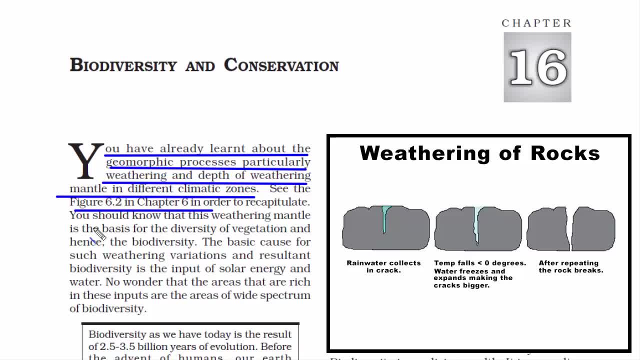 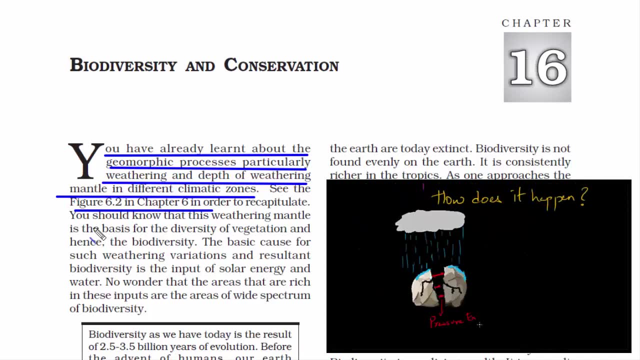 rocks into fine particles. Basically, soils are formed from rocks. When rain water gets collected in pores, they crack the rocks in a number of pieces. I have a video on how soil is formed from rocks. I'll put the link of the video in the description. just have a look at it. In that I have explained what are the. 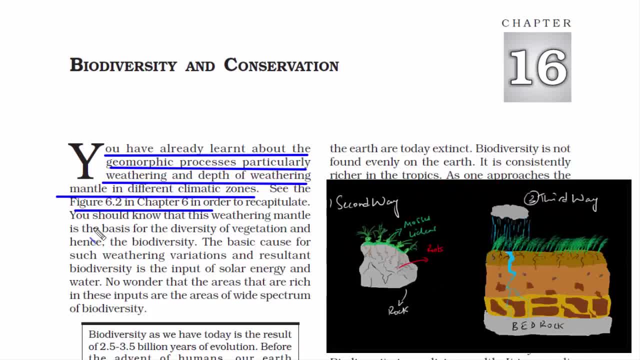 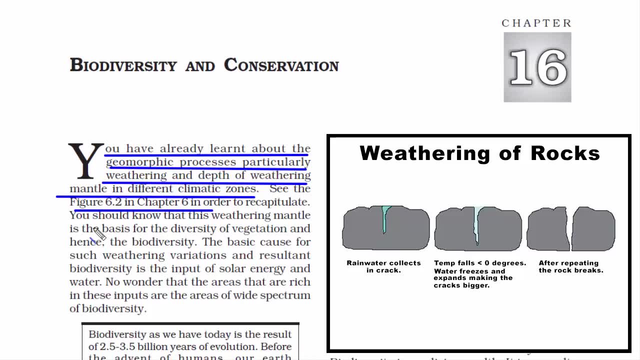 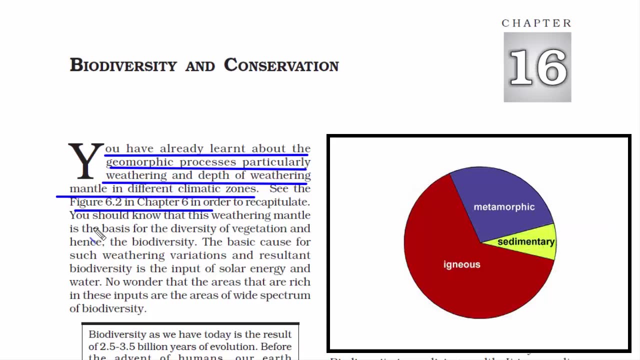 different ways in which rocks get weathered and turn into soil. you Now that you know how soil is formed from weathering of rocks. how did these rocks come into existence? Well, the most common thing that you will find on earth's crust is the igneous rock. 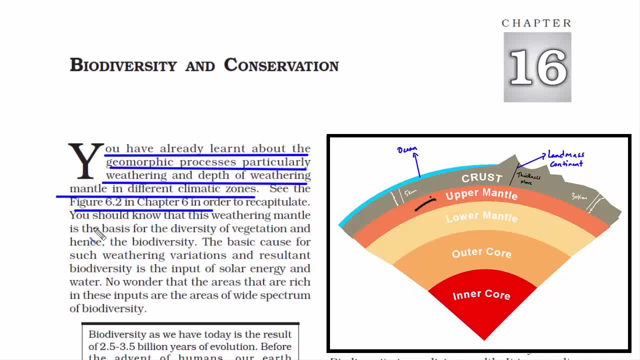 If you look at different layers of the earth, the mantle is the thick middle layer and the crust is the top layer on which we live. Magma originates in the lower part of the earth's crust and in the upper portion of the mantle. Magma is nothing but molten and semi-molten rock. 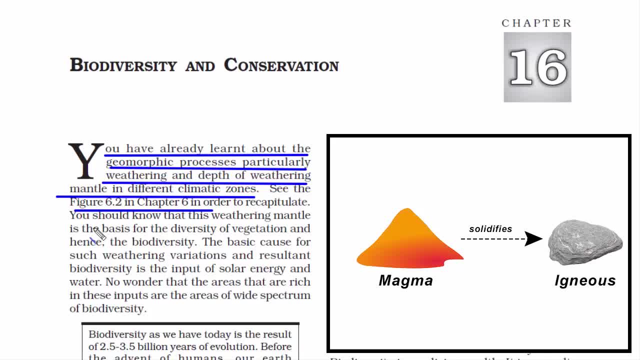 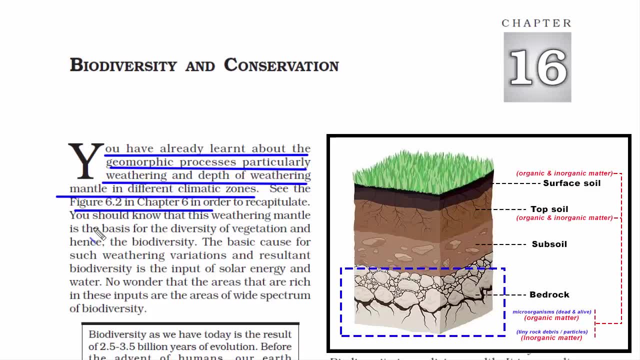 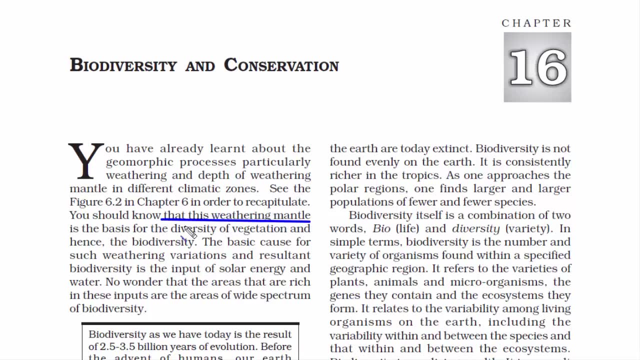 When it solidifies, it turns into igneous rock. That means when magma solidifies and turns into igneous rock, that becomes the bedrock. Slowly with time the bedrock turns into soil. Now here it says: weathering of the mantle is the basis for the diversity of vegetation. 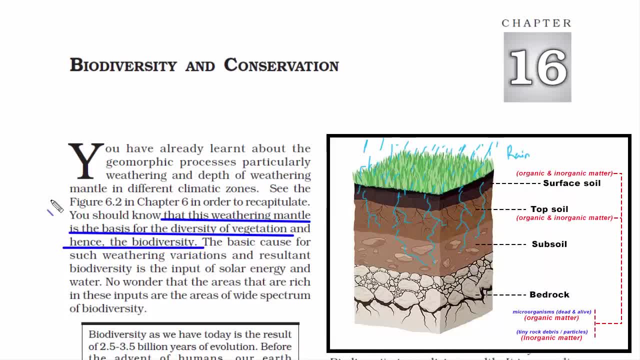 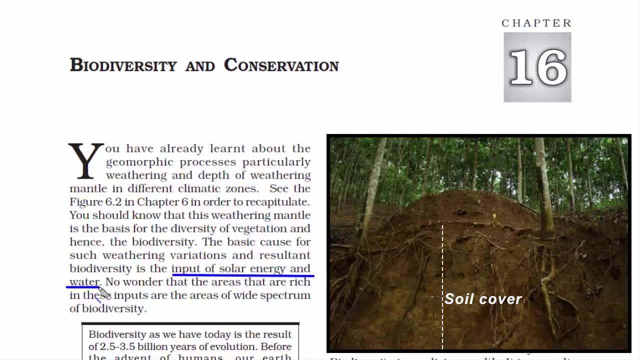 What this means is when the mantle gets weathered, obviously it will turn the bedrock into soil. If there is soil, then only trees, plants and forests will grow. So weathering of mantle has to be the starting point for the diversity of vegetation. 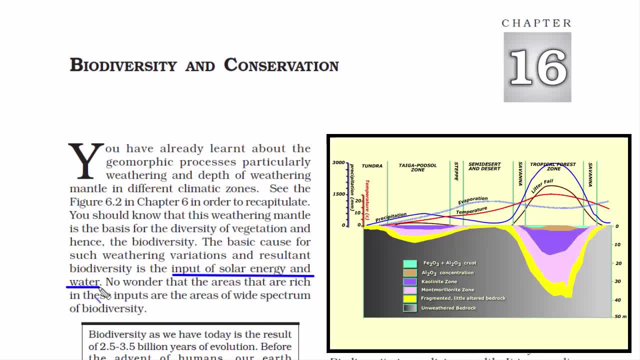 And if you look at figure 6.2 again, you will notice that the depth of weathering mantle varies in different climatic zones. This figure basically shows us a latitudinal variation of weathering mantle. It is more in the tropical region and less in the polar region. 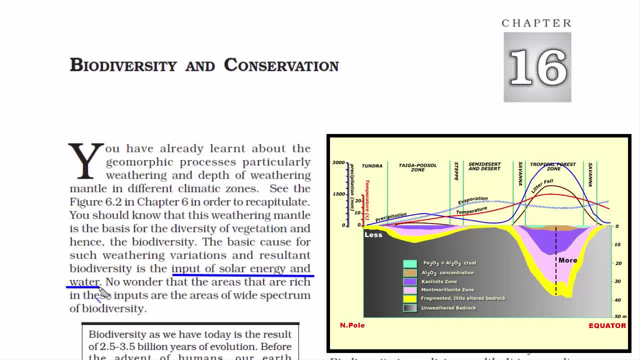 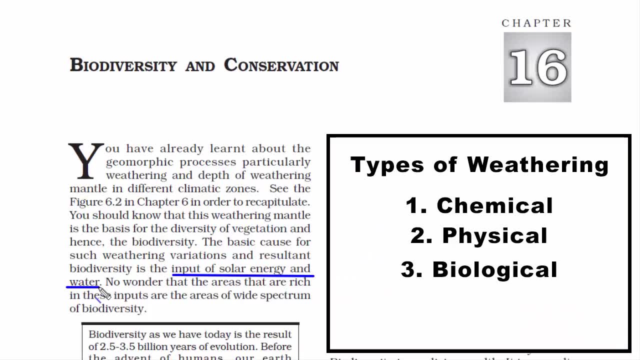 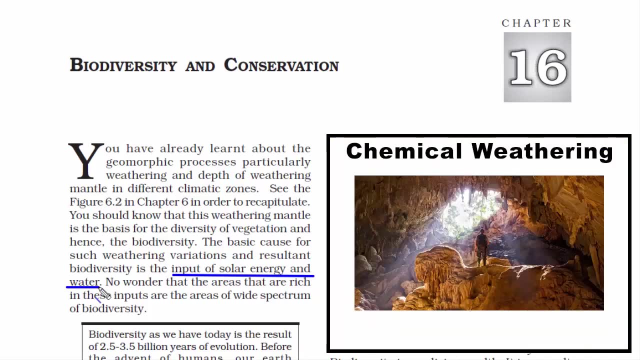 Why is it like that? It is only because of the way in which the mantle is getting weathered. So, basically, there are three types of weathering: chemical, physical or mechanical. and the last one is biological. Again, if you look at the figure, chemical weathering is most active in regions of high 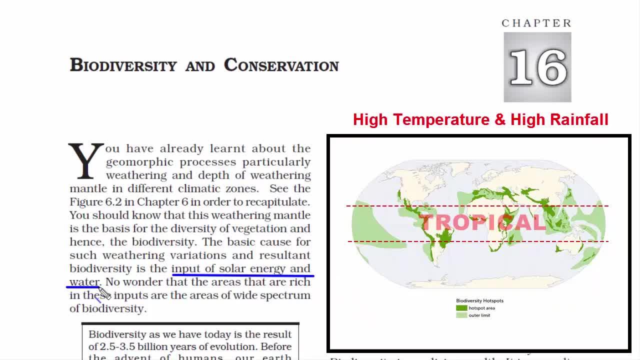 temperature and rainfall. that is your tropical region. Now, physical weathering is most active where temperature and rainfall are both low- that is tundra region- And biological weathering is most active in regions of high temperature and rainfall- again tropical region- because that's where you will find large, dense tropical forest. 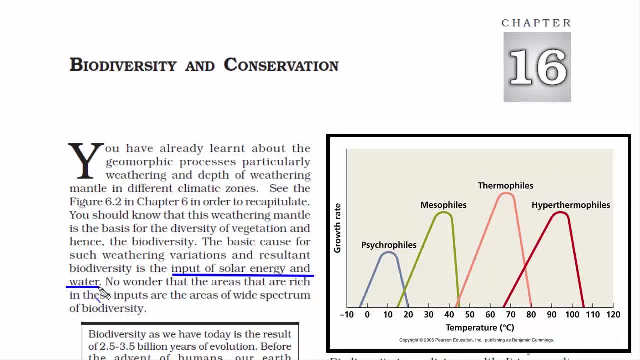 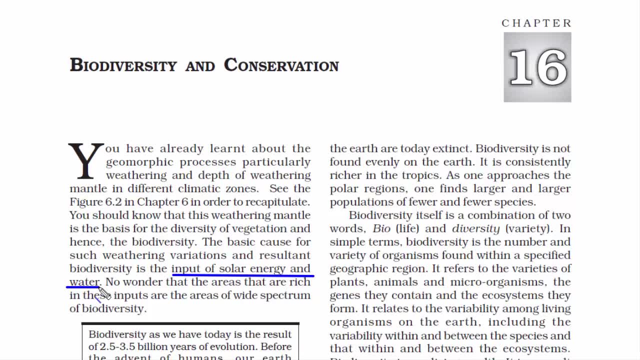 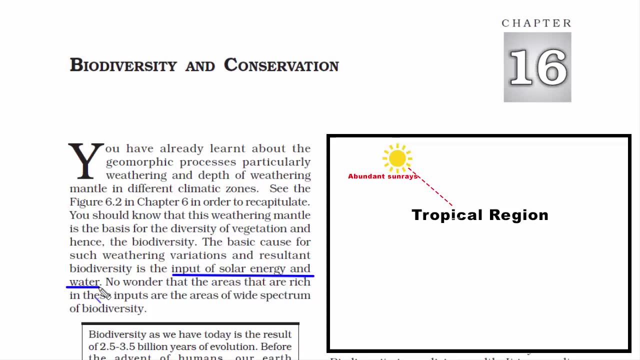 And tropical region is a moist place and bacteria thrive in moisture. The fact of the matter is, weathering of mantle is the basis for the diversity of vegetation. Now in tropical region, strong chemical as well as biological weathering takes place due to the abundant supply of incoming sun, energy and rain. 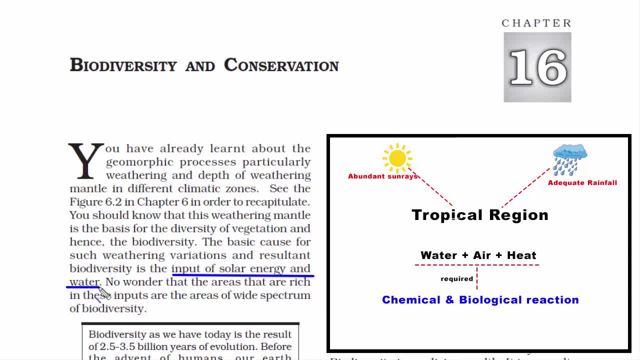 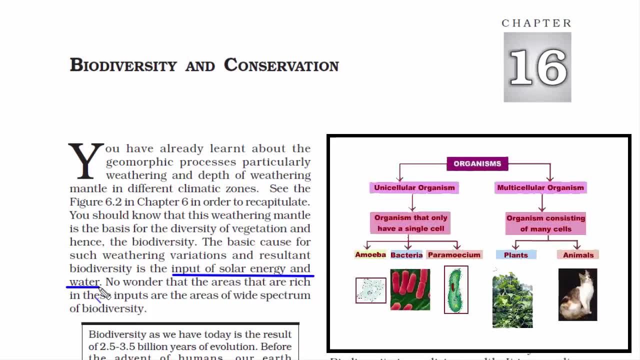 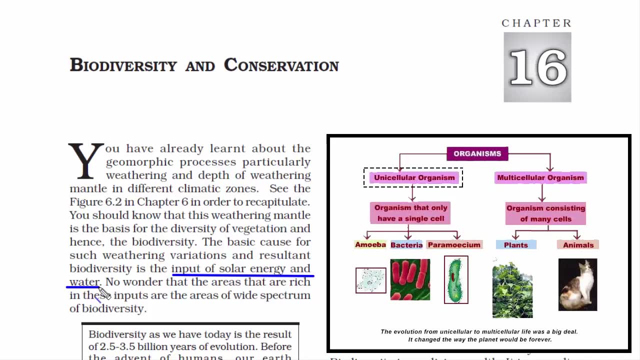 Water and air, along with heat, must be present to speed up all chemical as well as biological reactions. Another important point to consider is: long before plants and animals came, it was unicellular bacteria that transformed the atmosphere. After that, multicellular organisms came. 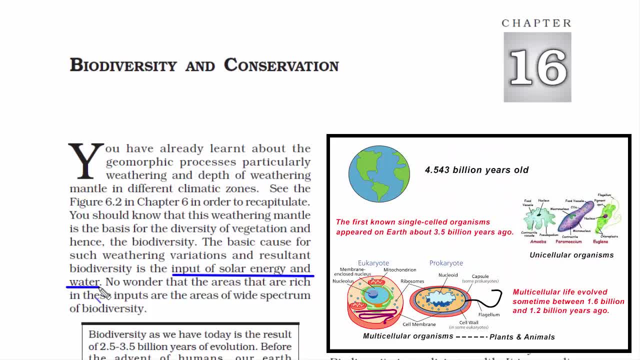 So clearly: weathering of mantle occurred first due to chemical and biological reactions. So clearly: weathering of mantle occurred first due to chemical and biological reactions. So clearly: weathering of mantle occurred first due to chemical and biological reactions And that's why it is called the weathering of mantle. 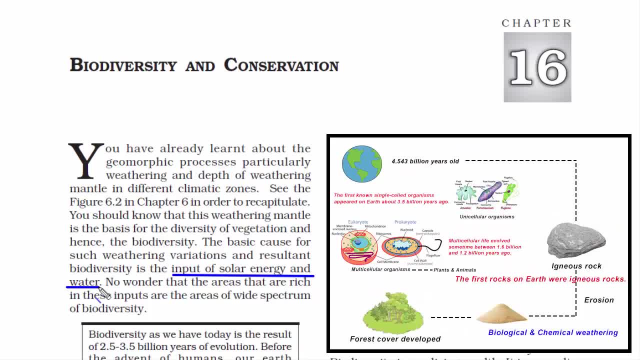 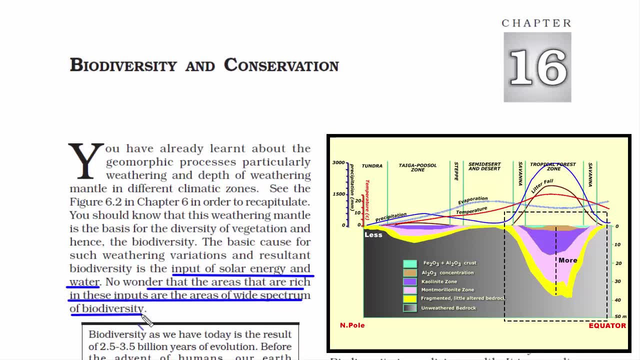 And that's why it is called the weathering of mantle. After that, there were climate changes in the last few years and after that forest cover developed Overall. the deepest weathering of mantle is found in the tropical rainforest region because of excessive input of solar energy and water. 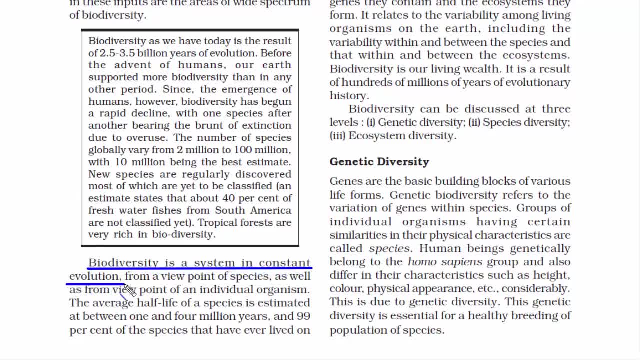 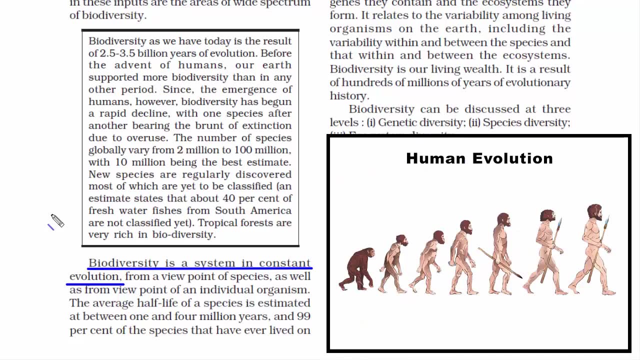 This sentence over here. it says: biodiversity is a system in constant evolution. If you see this statement, there's a lot that is going on in here, Especially these two words, constant evolution. explain with an example. If you look at the human body, it is a lengthy process of change. We never 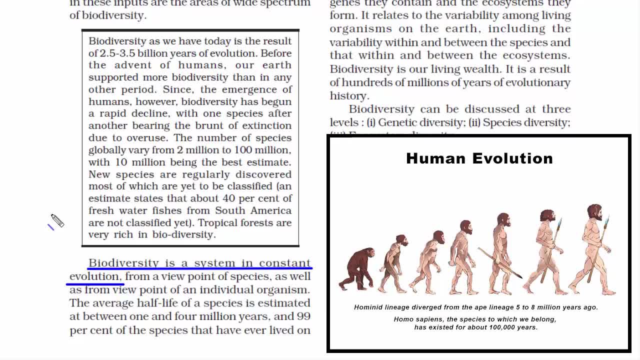 looked like this million years ago. If you can remember the picture here you will see the gradual rise of Homo sapiens. You will notice that there is a lot of physical and genetic similarities between the modern human and the apes, chimpanzees and gorillas. That means we all shared a common 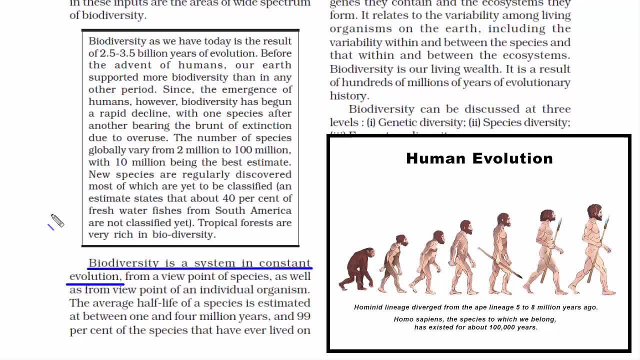 ancestor, But all of them are different species of early humans. With time, many species died and few descended. That is how we are present today. That means there must have been some change in the DNA of different species of early human. Till now, it is unknown as to how to classify. 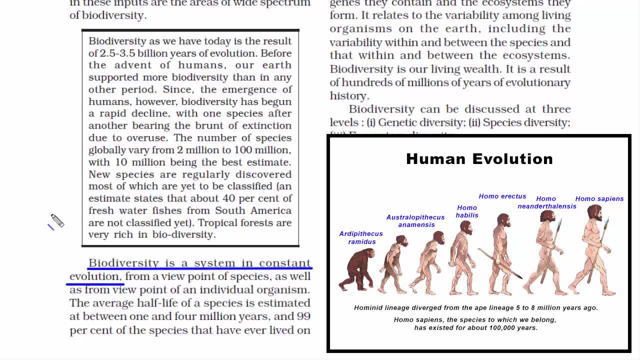 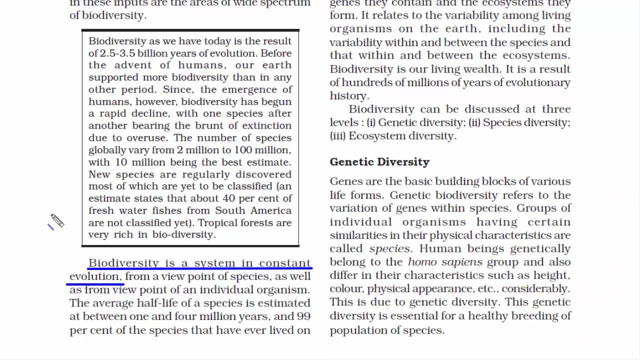 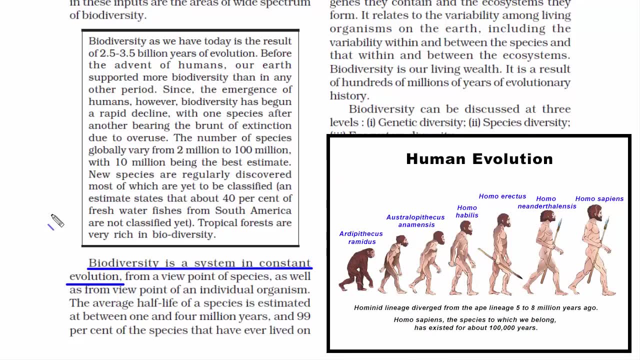 particular species of early humans and what all factors influence the evolution or extinction of early human species. So what I am trying to get is: biodiversity is a system in constant evolution. If humans have constantly evolved over a long period of time, similarly, if you look at the animal and plant species, they are constantly. 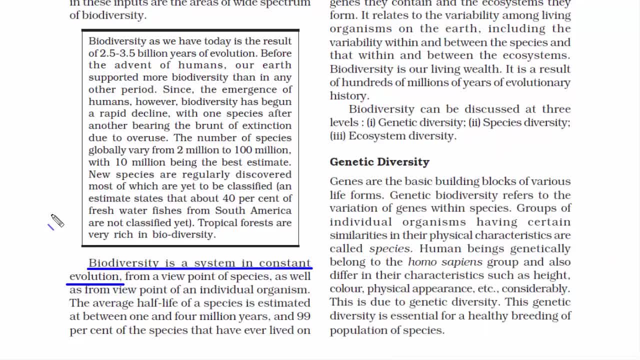 evolving with respect to their habitat and natural environmental conditions. Now that you know there is a constant evolution that is happening within all these species on our planet, another aspect that you have to understand is evolution will only take place if there is a mutation. 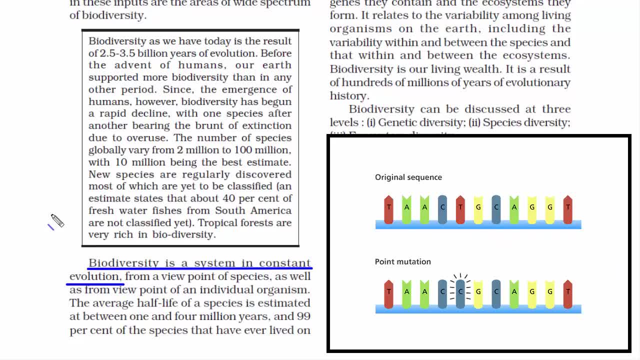 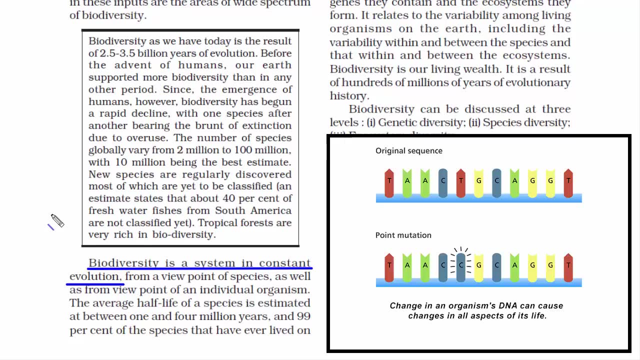 The meaning of the word. mutation is a simple change in DNA. DNA is a hereditary material of life. For example, we have DNA of our parents. Both of our parents have different sets of DNA which they acquired from their parents, So a change in an organism's DNA can cause changes in all aspects of its life, such as 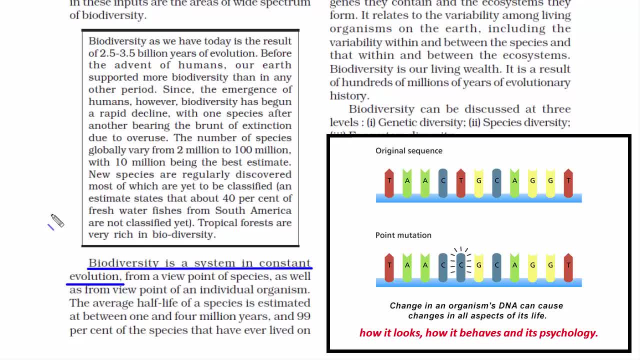 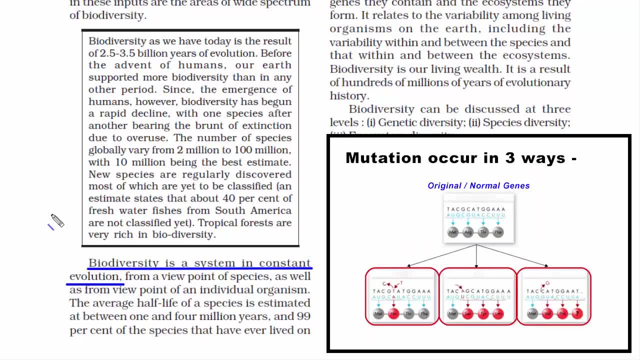 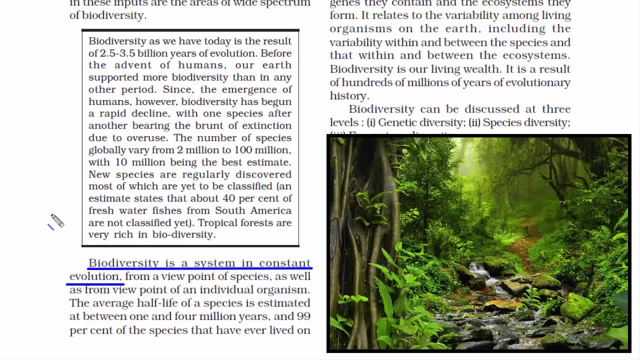 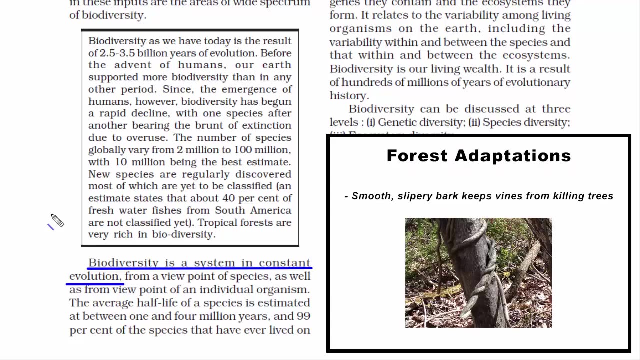 how it looks, how it behaves and its psychology. Now, this kind of mutation occurs in all living organisms. A small change in an organism's genetic material can have a wide range of effects. In a jungle, you will notice that different species of plants and animals are constantly interacting with one another for survival. 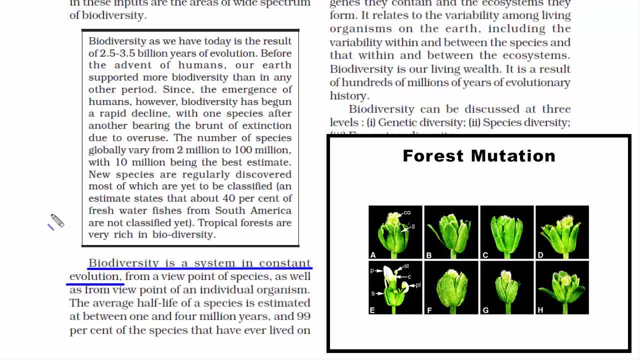 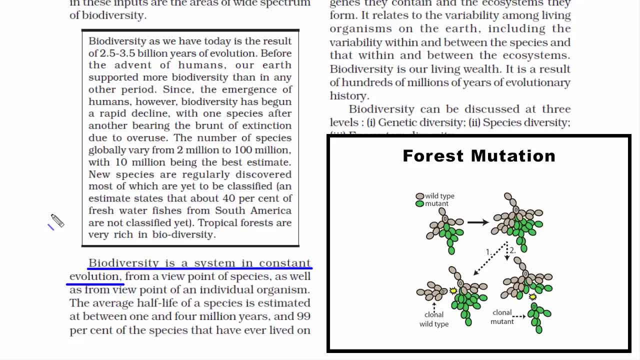 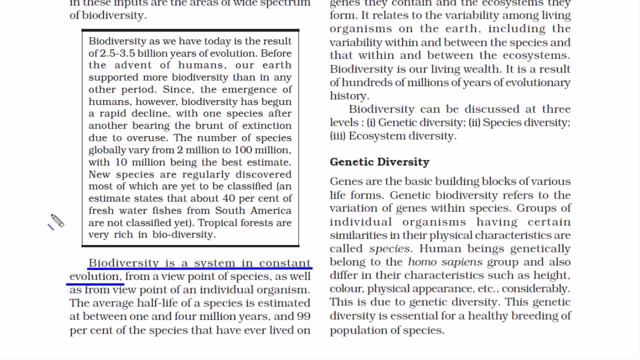 And then they adapt. Because of the interaction and adaption, there is a mutation of genes. Now this results in the evolution of a new species, And you will be able to notice the characteristics and physical traits of the new species with its parent species. 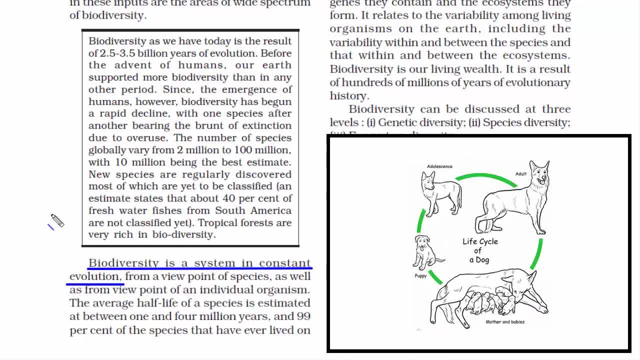 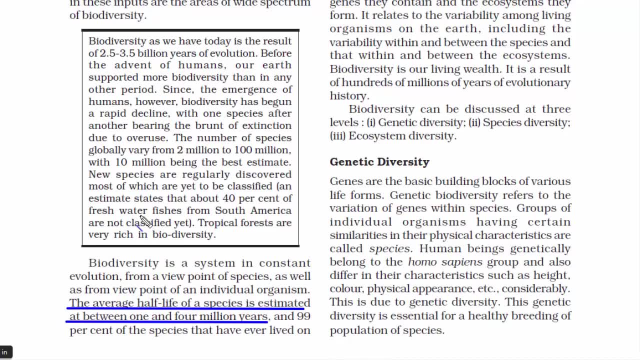 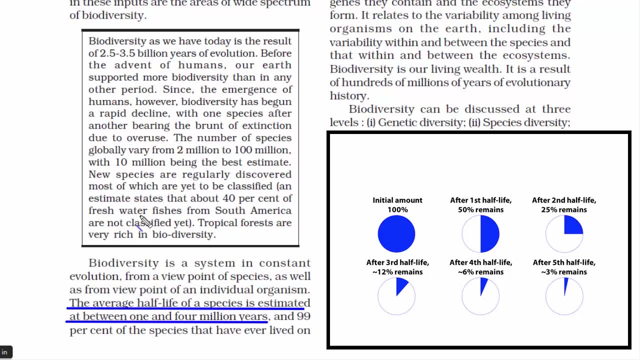 So, in a nutshell, evolution and extinction is a natural process. What comes has to go. Here it says the average half-life of a species is estimated at between 1 and 4 million years. What it means is that any species, when it reaches its half-life, where its value depreciates, 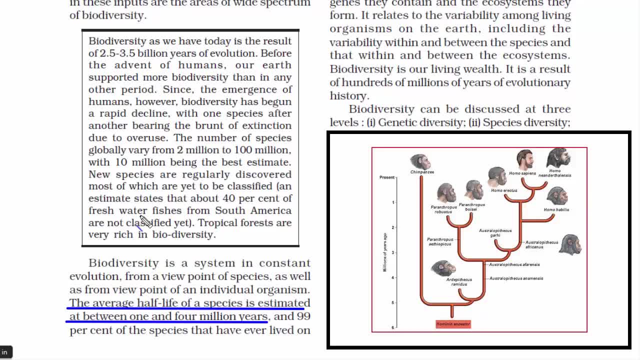 to half, Because you see a species constantly go through physical and biological changes in the DNA. So the original components of the DNA will transform into new ones over time And when that value of the original DNA is 50%, because anything beyond 50% will not have the concentration of the original component. 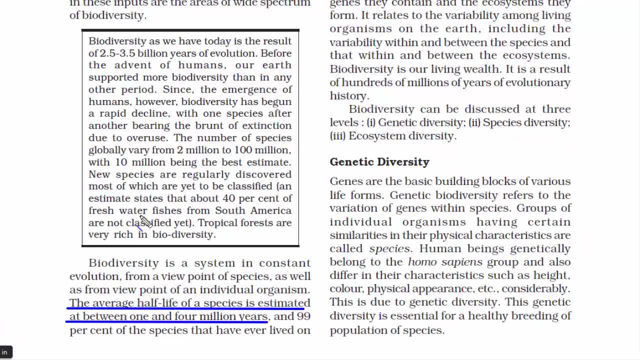 That's what is the meaning of half-life of a species. Now, this 50% of original traits of a species is estimated to live anywhere between 1 to million years. Now, that's a lot of time, But again, the deeper philosophical statement is what evolves. 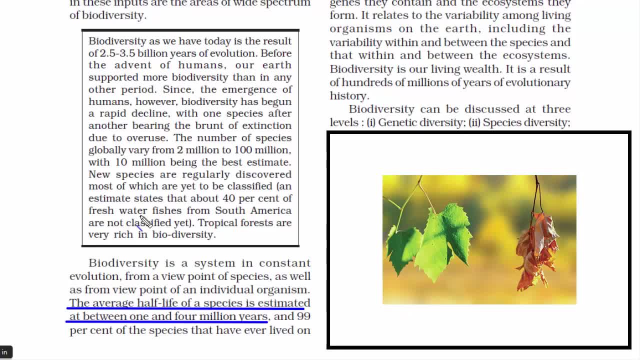 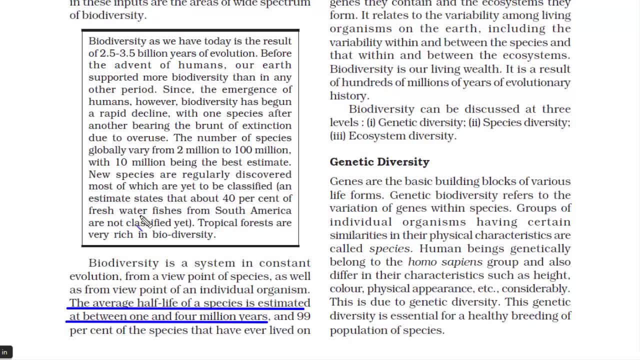 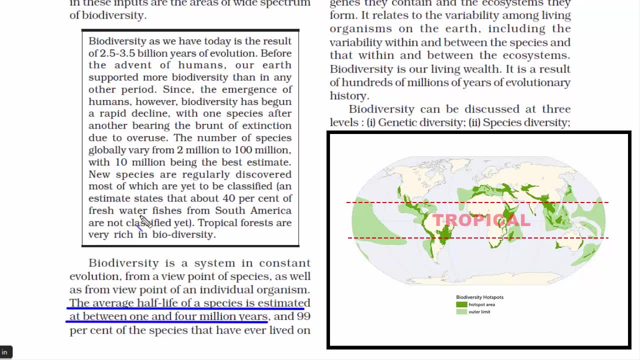 has to face destruction, or in other words, what comes has to go. Evolution and extinction is a natural process, And this is true in every aspect in life, not just in the evolutionary matter. If you look at the biodiversity hotspots around the world, you will notice that the tropical 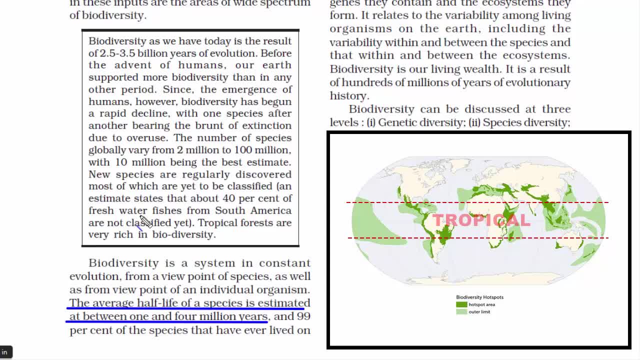 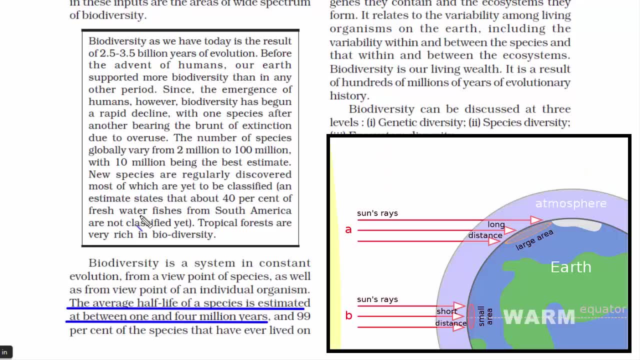 regions are richer in biodiversity, And I have given you the reason before. It is due to the abundant input of solar energy and water. At the equator, the sun's rays are the most direct on Earth. As you migrate towards the poles, the sun's angle in the sky decreases. 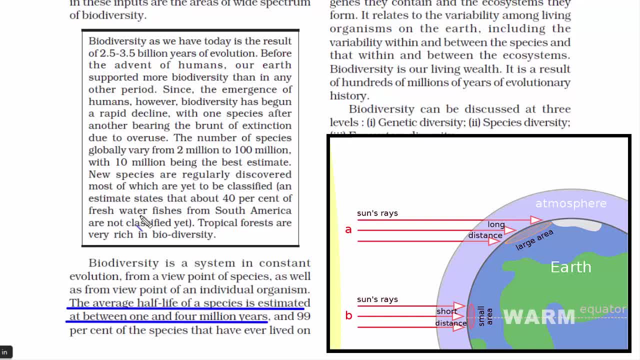 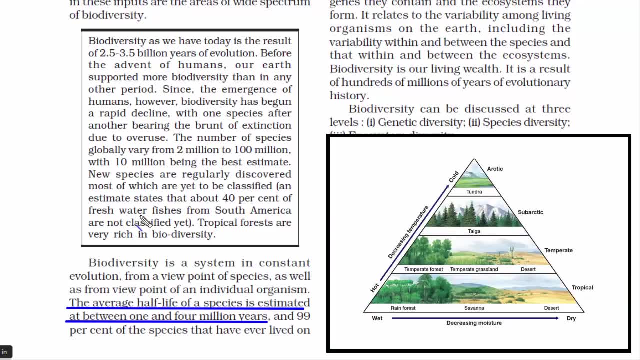 and that affects the incoming solar intensity. Likewise, as you go away from the equator towards the polar region, the biodiversity decreases because very few plants and animals survive in the extreme cold and ice that cover these regions all throughout the year. So, if you look at the polar regions, the biodiversity decreases because very few plants and animals survive in the extreme cold and ice that cover these regions all throughout the year. 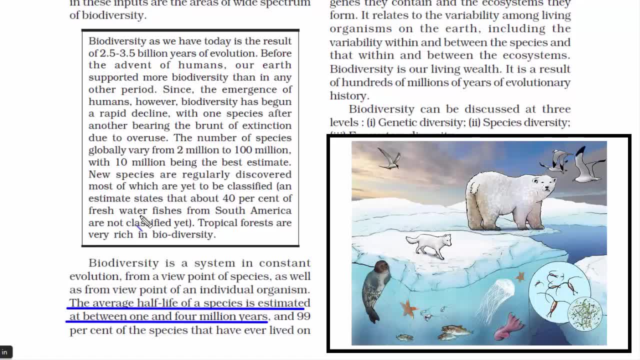 But the data on aquatic biodiversity, whether it is more or less in polar regions, is still unverified. I have read a few research papers which shows that the aquatic marine ecosystem is truly rich in polar regions, But again the research is unproven, so can't really. 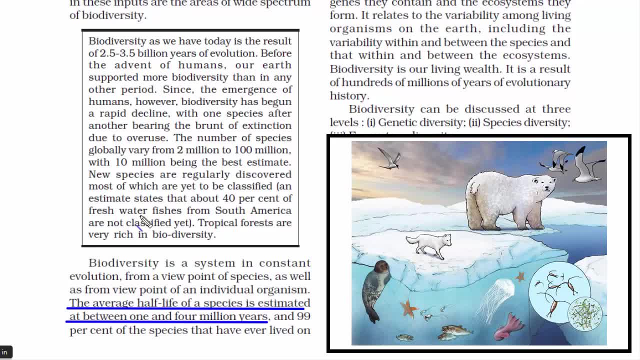 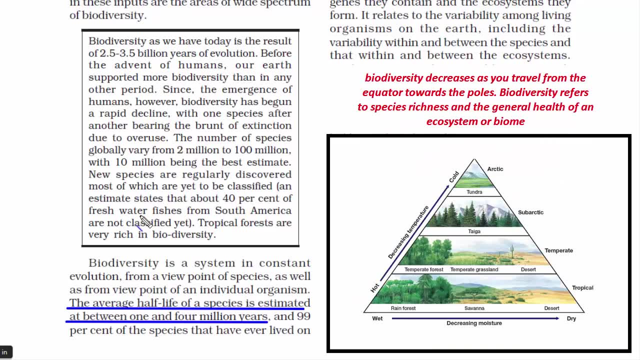 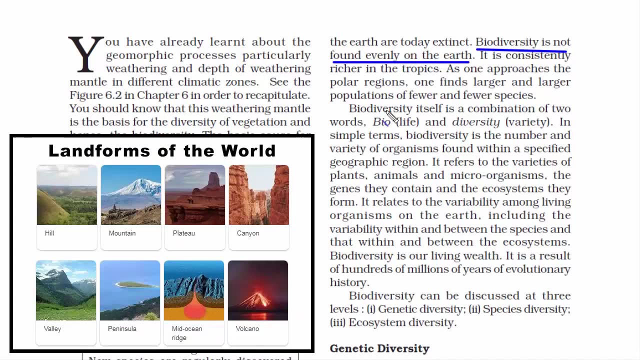 make a solid statement on it Until it's confirmed and validated. we need to stick to the claim that as we go away from the equator towards the polar regions, the biodiversity decreases. Biodiversity is not found evenly on the Earth, which is so true If you look at the 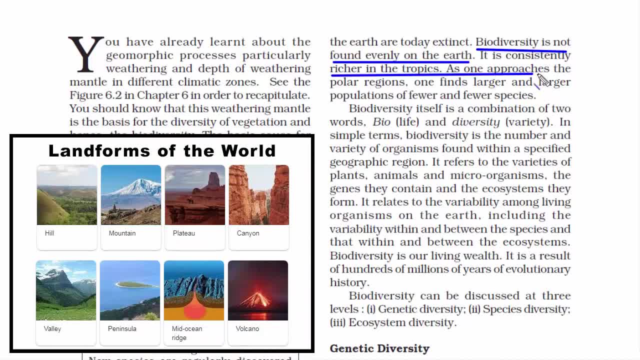 physiographic division of the Earth's landform. at some places you will find a massive mountain, then plateaus, desert, both warm as well as cold. we have islands, then we have coastal plains. You see, there is a massive difference in landform as you go from one place to another. 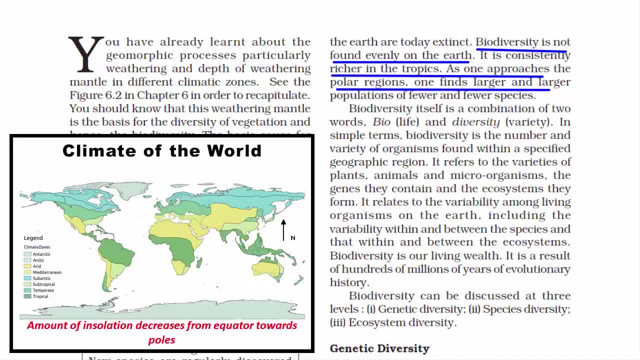 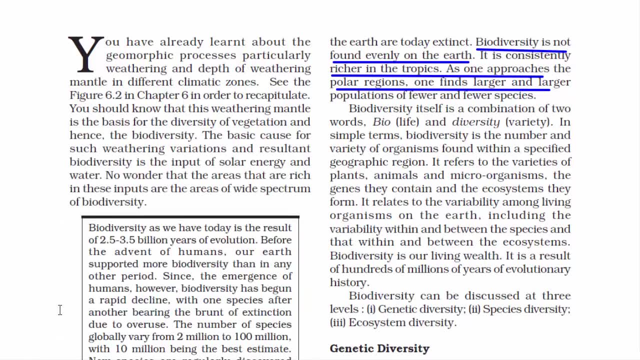 Now, landform is one part. the other part is climatic conditions. Again, if you go from one place to another, the weather changes. So if you go away from the equator towards the other, the weather and climatic conditions change drastically. And all these differences. 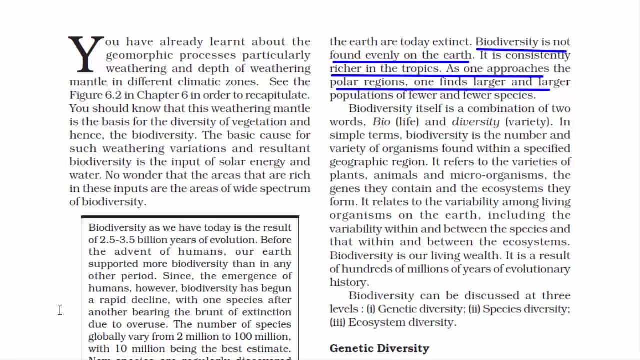 give birth to different forms of life, And that's how biodiversity is not the same everywhere. It's not evenly spread out. I don't need to tell you the meaning of the word biodiversity: Bio means life, and diversity means variety. So together it means a variety of organisms found within a specified geographic. 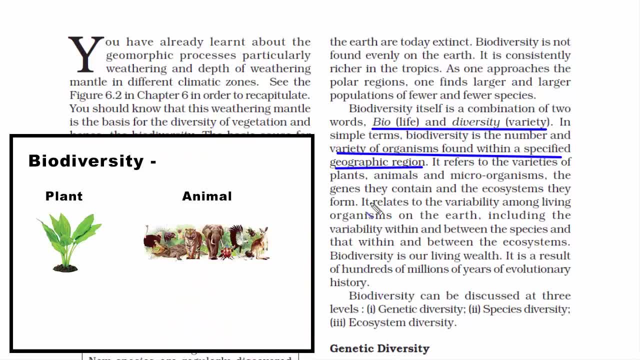 region. However, when we see the word biodiversity, it not only includes biodiversity, but also includes plants and animals. But we also have to include the microorganisms which we cannot see with our naked eyes, And moments back we learned that it's due to evolution. 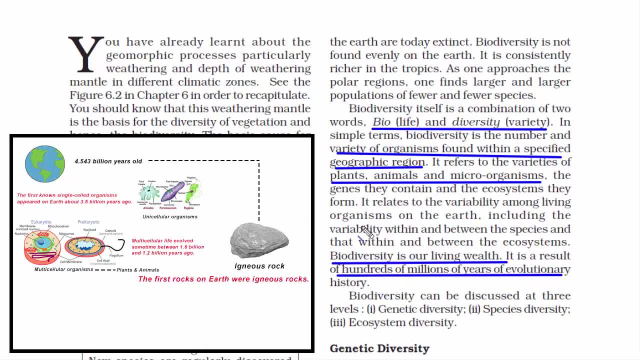 biodiversity is so rich today. In other words, whatever we see around us, I'm talking about living things. our existence is a result of hundreds of millions of years of evolutionary history. Biodiversity can be discussed in three levels. They are: Genetic diversity, Species diversity. 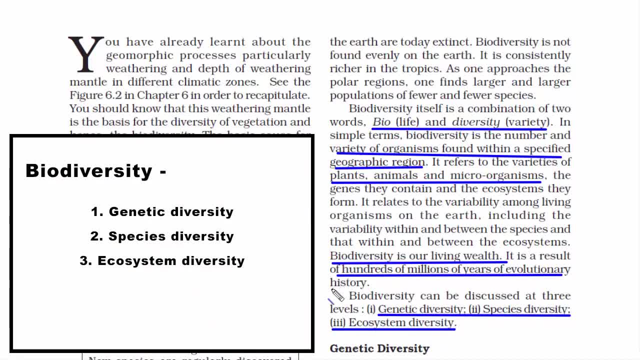 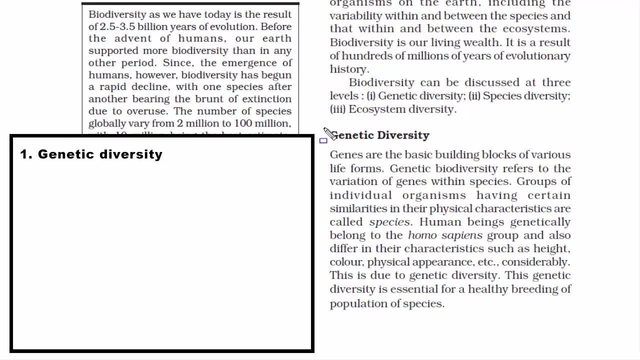 and Biological diversity. Biodiversity can be discussed in three levels. They are Genetic diversity, Species diversity and Ecosystem diversity. We will go through each one of them and try to understand them with examples and illustrations. The first one is genetic diversity. When you see the word genetics, immediately think of 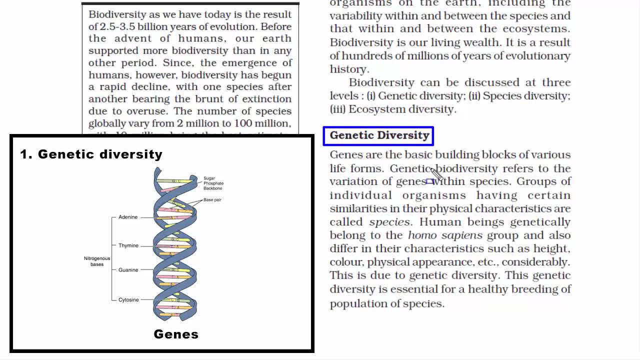 genes, Because in biology, genetics is a branch that is concerned with the study of genes. Now the next question is: what are genes? They are the basic building blocks of various life forms. What I mean by that is: let us take the example of a human, Every human being. 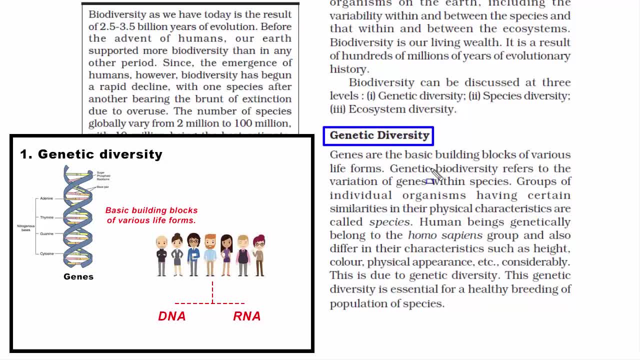 or any living organism on earth, has DNA and RNA present in their body. DNA stands for Deoxyribonucleic Acid and RNA stands for Ribonucleic Acid. First, let me show you where exactly DNA is located in our body. Here's the thing. a human 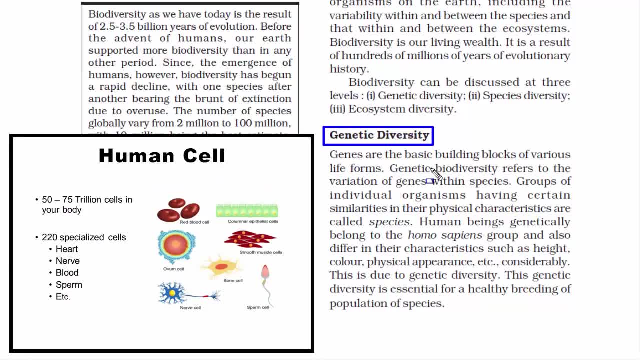 body is made of cells, And we have around 100 trillion cells in our body. The number can depend based on the size of your body. If you are big, you will have more cells, and vice versa. Now, these cells- 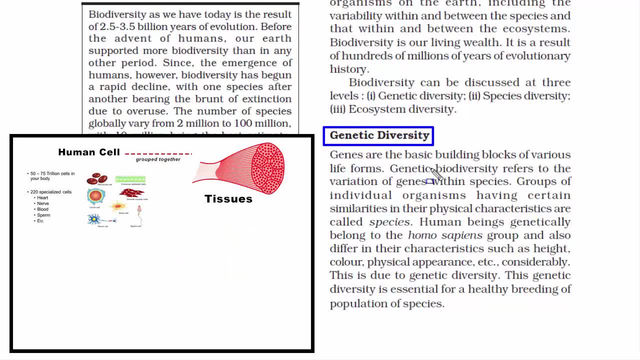 When they are grouped together, they form tissues. Now, the human body has a lot of organs, right? I am talking about the brain, heart, kidneys, liver, stomach, lungs, etc. These are some vital organs. They are made of tissues. 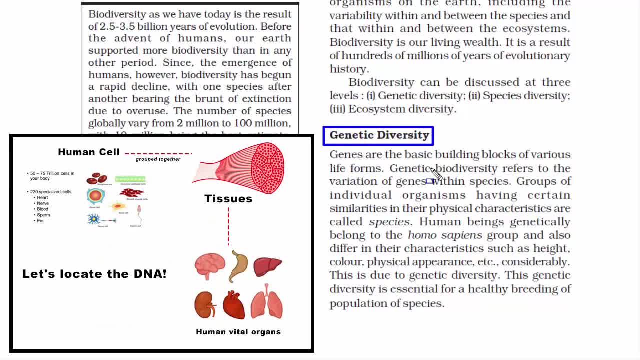 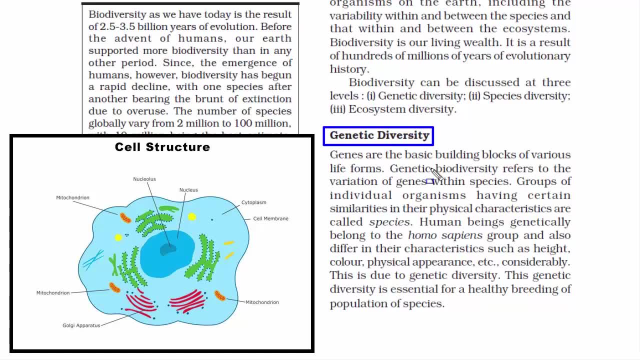 Now let's locate the DNA. As I said, a human body is made of cells and we have around 100 trillion cells in our body. If you look at a single cell closely through a microscope, you will find a nucleus inside almost every cell in our body. 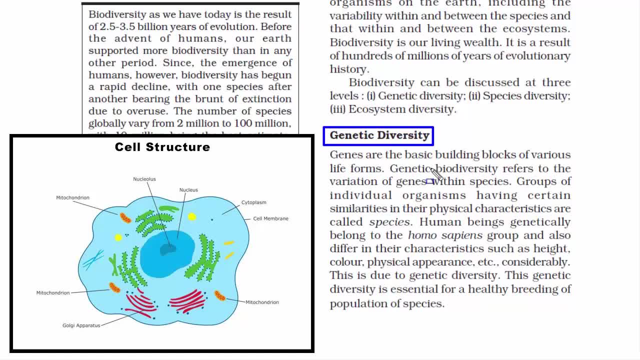 The reason I said almost is that not all cells have a nucleus. I am not going to make it too technical, otherwise this will become a biology lesson. All you have to know is that cells are of two types: Eukaryotic and prokaryotic. It is the prokaryotic cells. 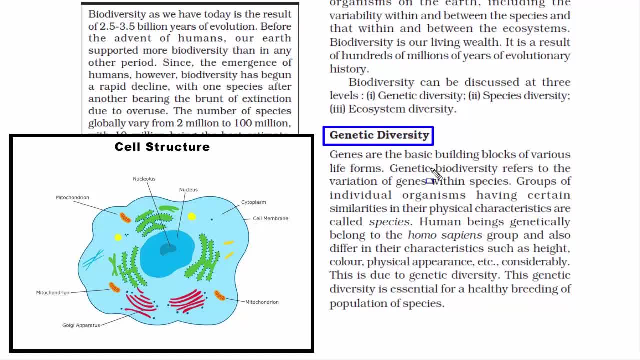 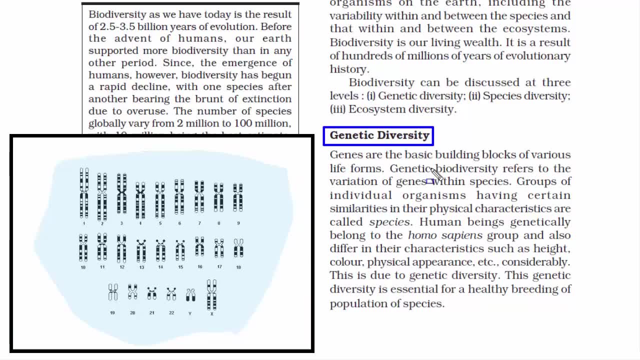 that don't have a nucleus. That's all you have to know as of now. Anyhow, as I was saying that a single cell has a nucleus inside, now, each nucleus contains 46 chromosomes that are arranged independently, And this is even less important when you put 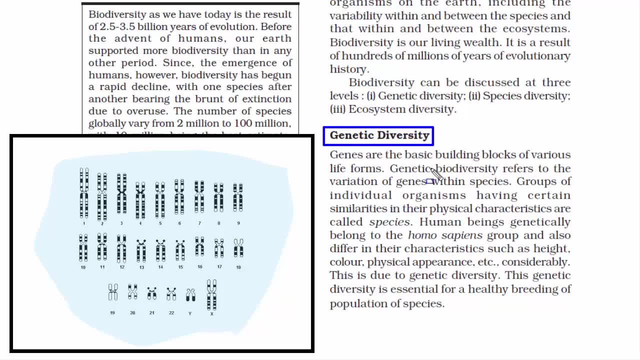 in a few neutrons and getting the full structure These neutrons, wherever they are located, have are arranged in 23 pairs. That means every human will have 23 pairs of chromosomes. 22 of these pairs look the same in both males and females. The 23rd pair is the sex chromosome, which determines 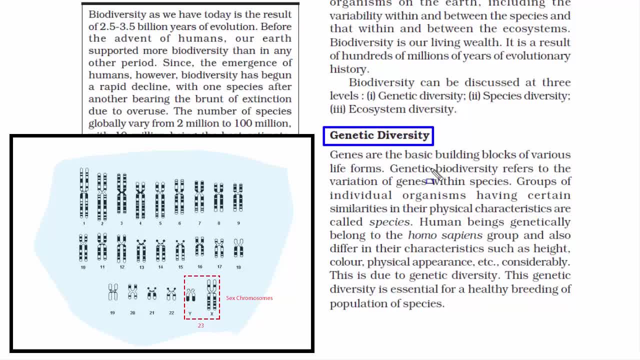 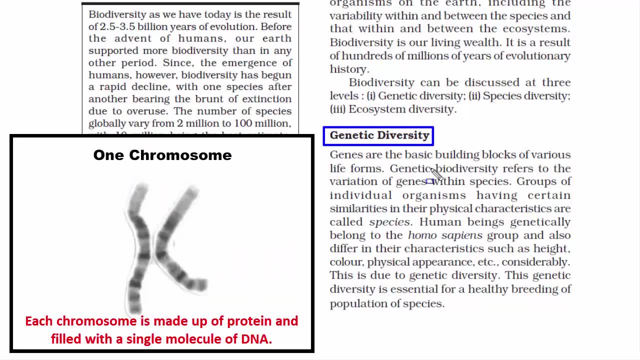 males and females. Anyhow inside the nucleus of a single cell, there are 23 pairs of chromosomes arranged in a thread-like structure. Each chromosome is made up of protein and filled with a single molecule of DNA. It looks like a double helix, that is, two long, thin strands. 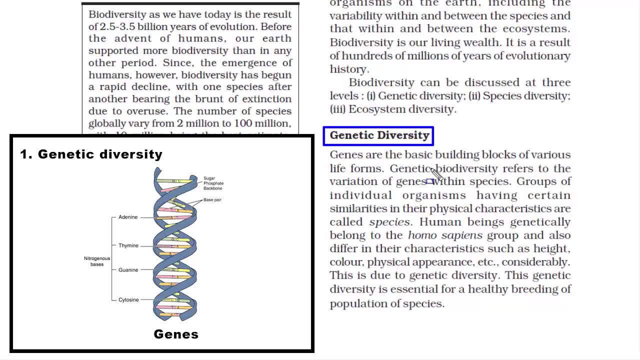 twisted around each other like a spiral staircase. These strands are held together by the hydrogen bond that is present in between. If you look at an individual segment of a DNA strand, this is what is called as a gene. It is in this segment you will find the instruction to make. 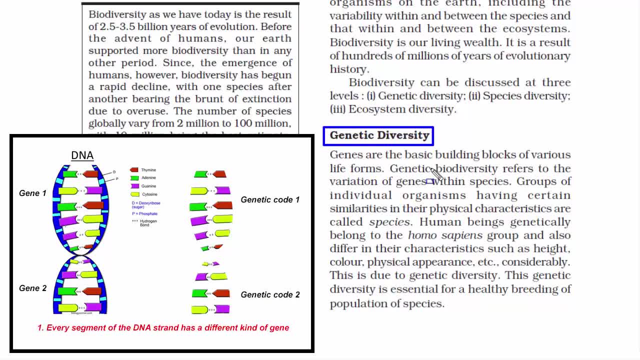 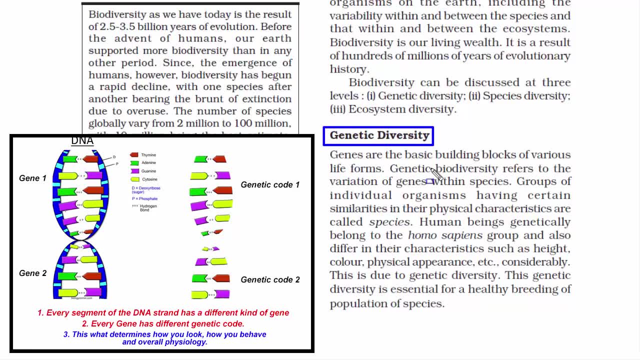 proteins that form the building block of life. Now, every segment of the DNA strand has a different DNA strand. Every segment of the DNA strand has a different DNA strand, And this is what determines how you look, how you behave and overall physiology, And it is also 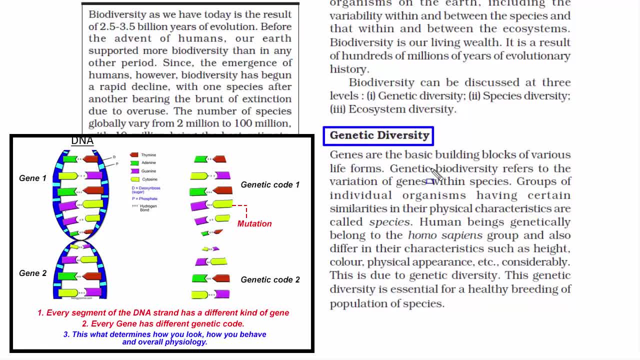 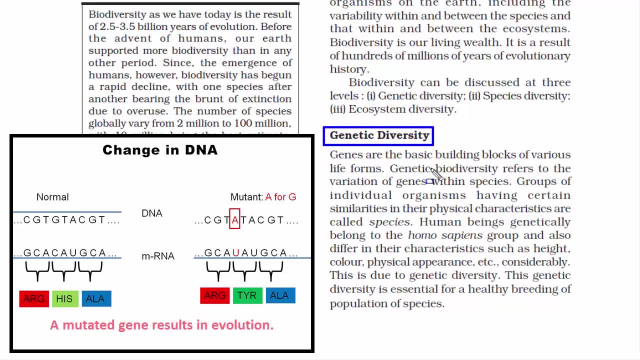 this place where mutation takes place, which is basically an incorrect code that results in a failure to correctly produce its specific protein. A mutated gene results in evolution. Basically, now there is a change in DNA And this can cause changes in all aspects of the organism's life. 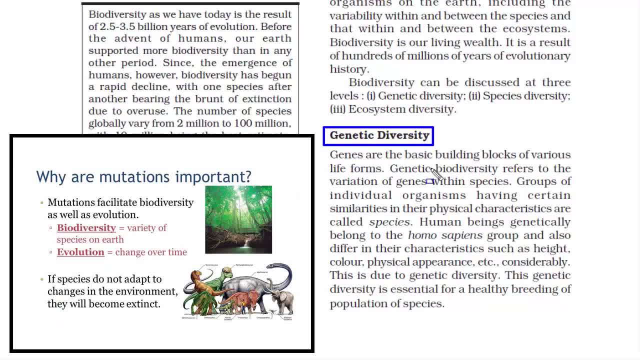 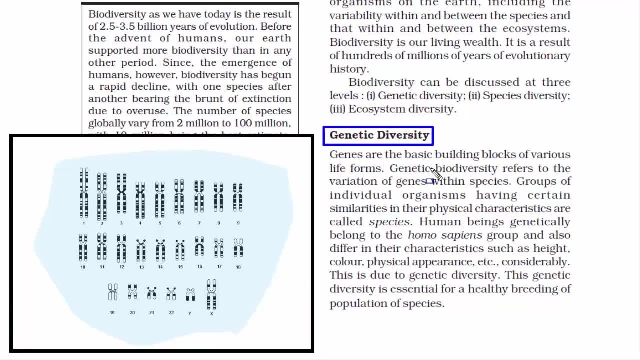 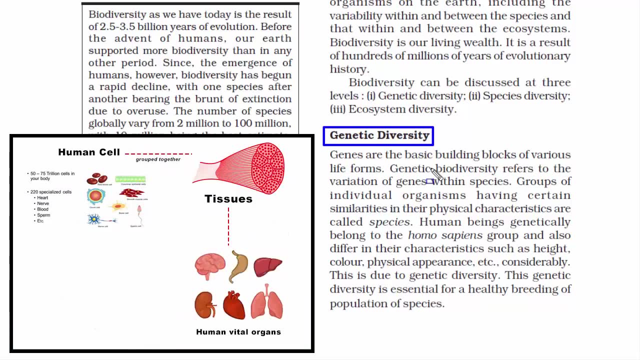 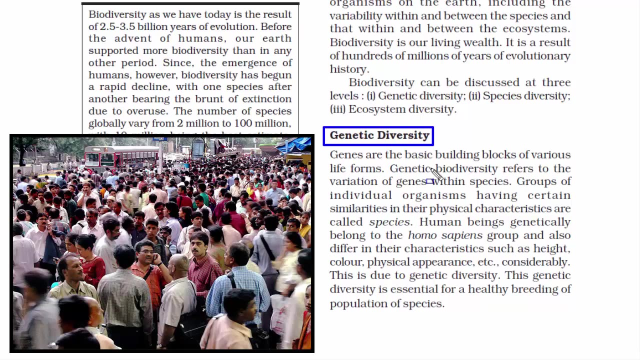 That's why mutations are essential to evolution. They are the raw material of genetic variation. Now imagine this: Every cell in your body carries some genetic information which determines how you look, how you behave and overall physiology. And we have also learned that cells are grouped together to form tissues, And tissues form organs of a body. That means we. 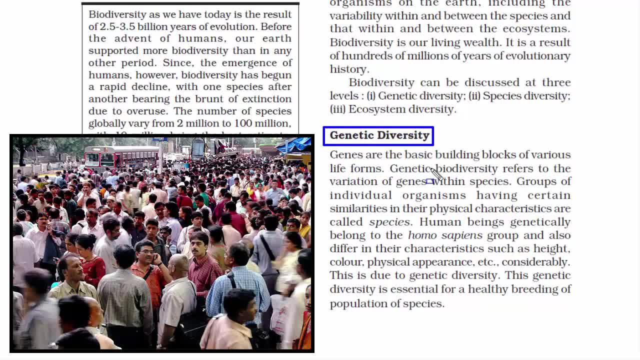 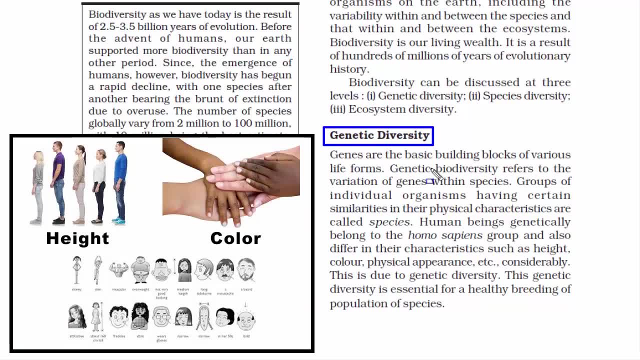 humans have so much of similarities in our physical characteristics And that's how we are called human species, But then we are called human species, And we are called human species And we are called human species. We do differ in characteristics such as height, color, physical appearance, etc. So this is what 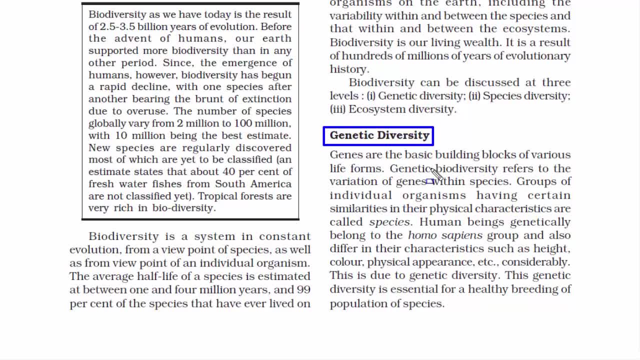 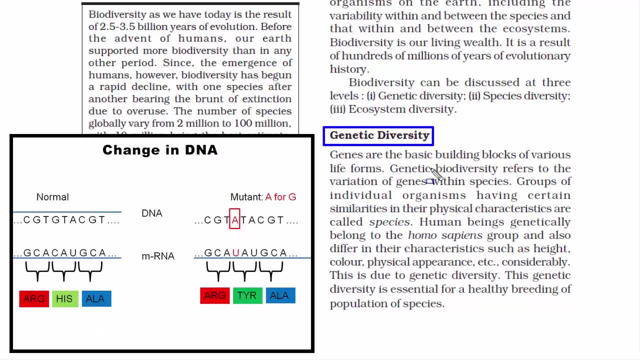 is called genetic diversity. Diversity means uniqueness, So if genes determine our physical characteristics, such as height, weight and skin color, that means, due to changes that occur in the segments of DNA will cause diversity, or in other words, gene mutation. Now it is true that 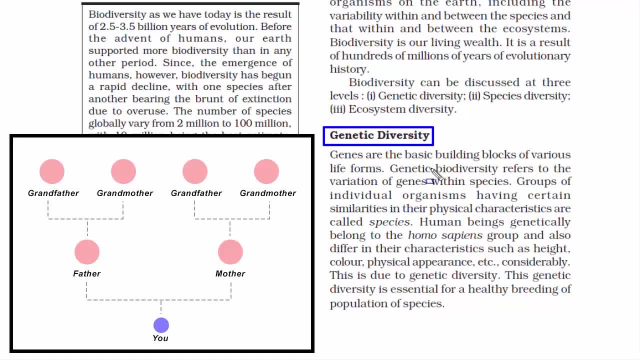 most of the genes you acquire are from parents, but then some of it you also acquire throughout your lifetime. So this is what is called genetic diversity, And it is true that most of the genes you acquire are from parents, but then some of it you also acquire throughout your lifetime. 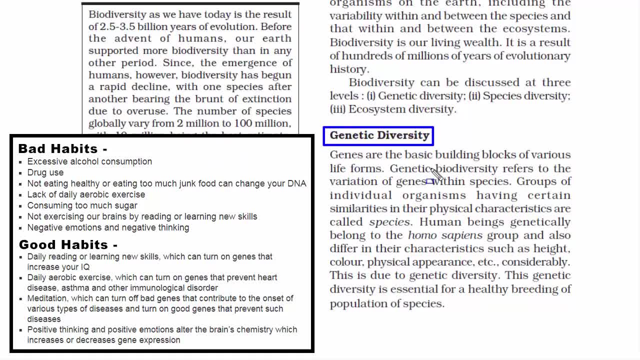 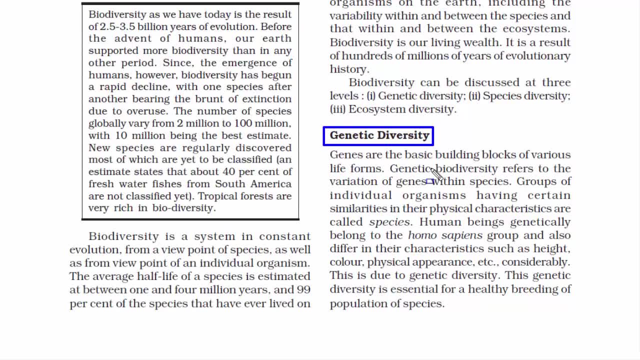 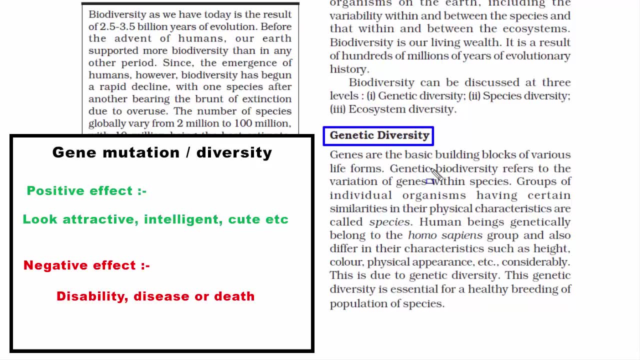 For example, you develop habits, routines, behavior etc. So this kind of change is also encoded in the segments of your DNA. That means we can say that gene mutation or diversity has both positive as well as negative effectA negative impact may cause disability, disease or death. Likewise a positive 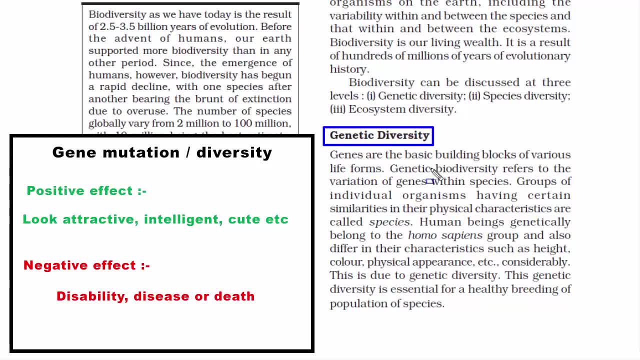 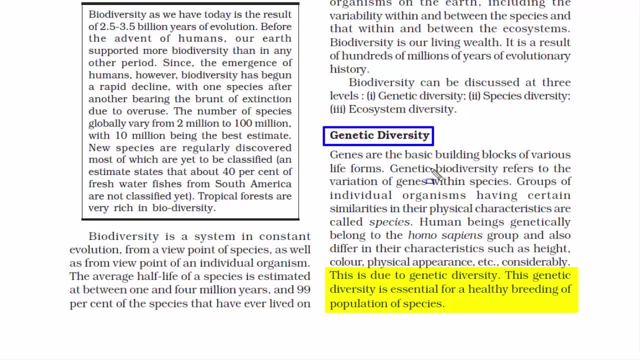 impact can make you look attractive, intelligent or cute. Here it says genetic diversity is essential for healthy breeding of population of species. It is true, a healthy population of species has tremendous economic as well as environmental benefits. But for a second, just think about it. can we make a claim that healthy breeding of any 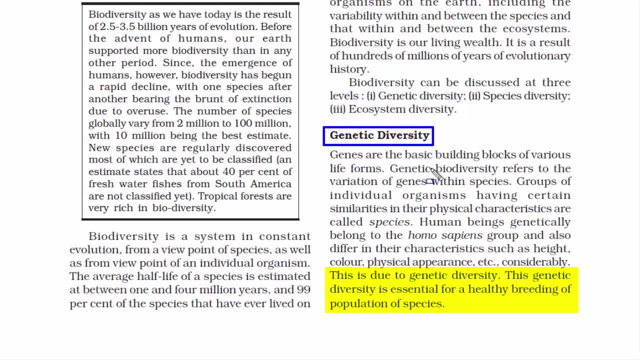 population also has an external factor associated with it. You see, sometimes we cannot blame individuals for having poor health, because it is determined by their circumstances and environment. You see, on one hand, genetic diversity is important for healthy breeding and on the other hand, I am saying that it's not in our hands to have healthy genetics. 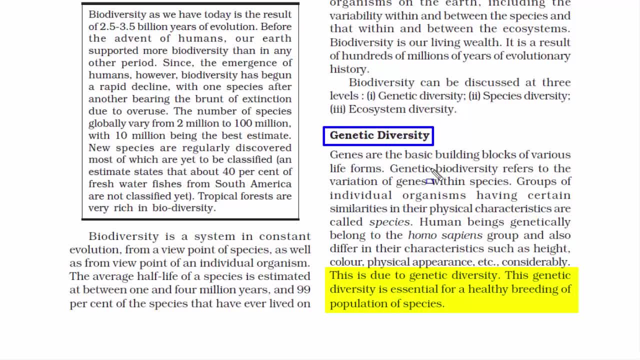 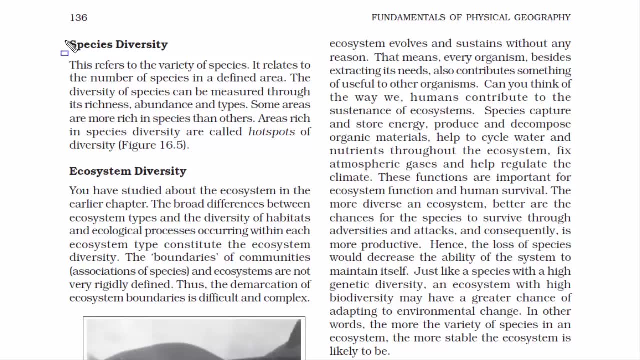 Sometimes the external environmental factors affect and shape our genes. I am talking about food, lifestyle, poverty, pollution. Anyways, I hope you understood the meaning of genetic diversity and how genes are the basic building blocks of various life forms. The second one is species diversity. 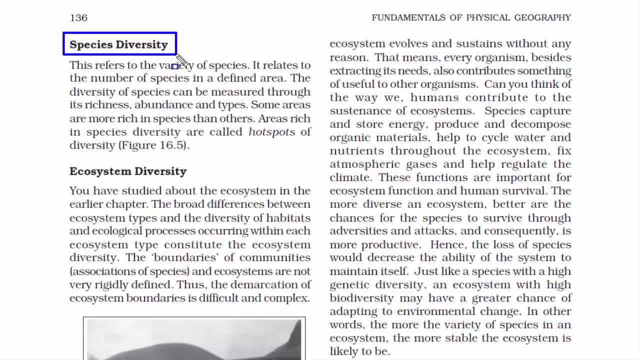 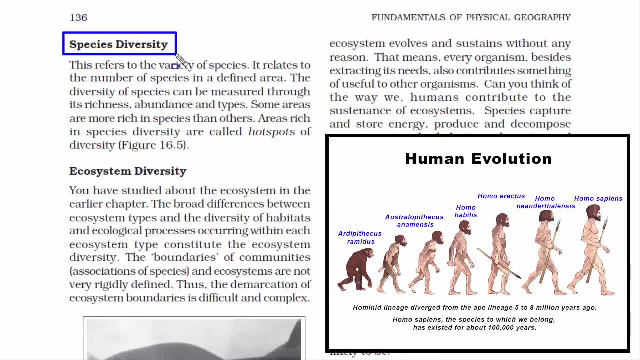 We already know the meaning of the word diversity, So it only makes sense if we could understand the word species in a much better sense. Let's take the example of a human. again, Human is classified as species. right, That's how we call the human species. 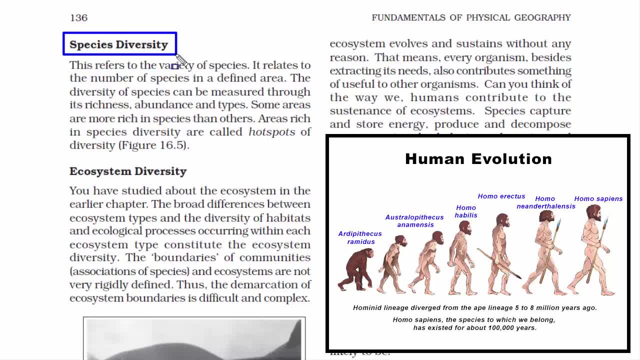 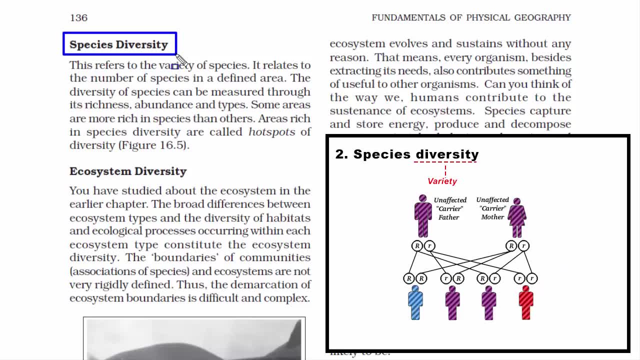 Now, in order to call a group of living organisms as species, there have to be some similarities so that they can exchange genes or interbreed with each other and produce offspring. Now, when we see the words species diversity, we already know the meaning of the word diversity. 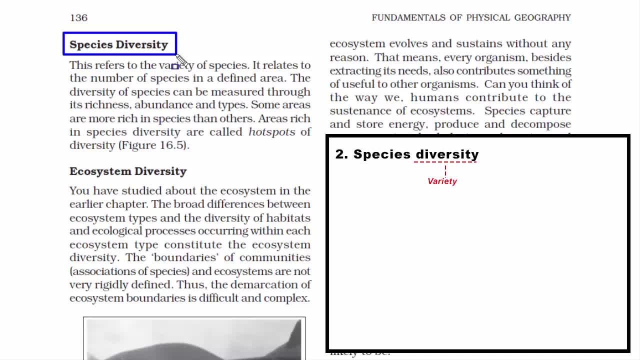 We already know the meaning of the word diversity, So it only makes sense if we could understand the word species in a much better sense. When we say species diversity, it means a variety of species. For example, we have human species, then plant species, animal species. 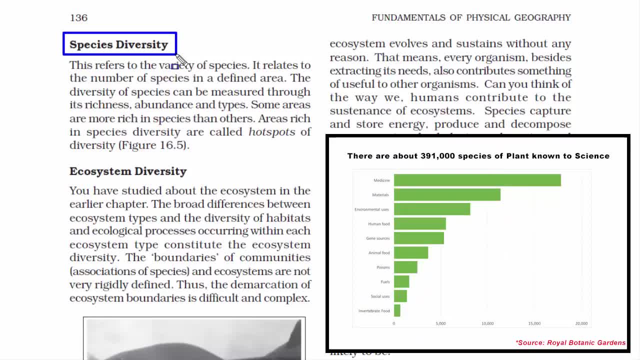 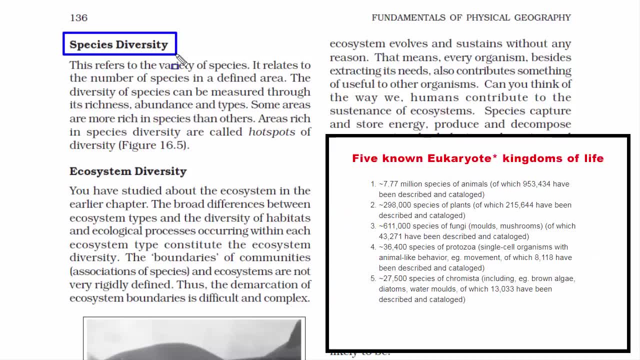 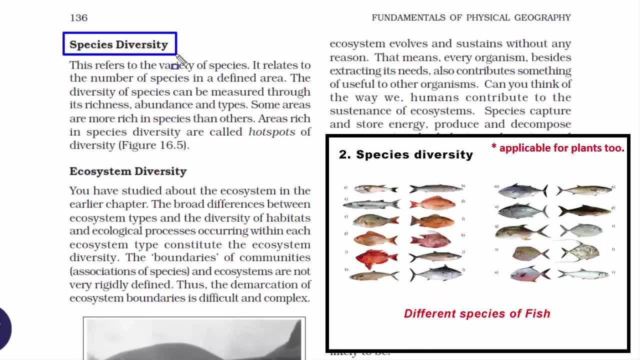 Within the plant species, there are about 400 000 species of plants that have been documented so far. Similarly, within the animal species, there is an estimation of 9 million species of animals on earth. So you see, every group of living organisms have a variety of species and all these species 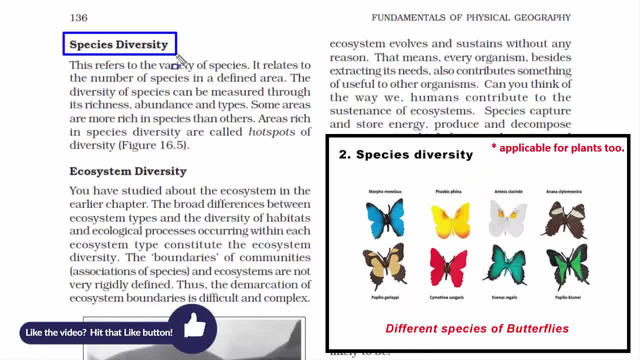 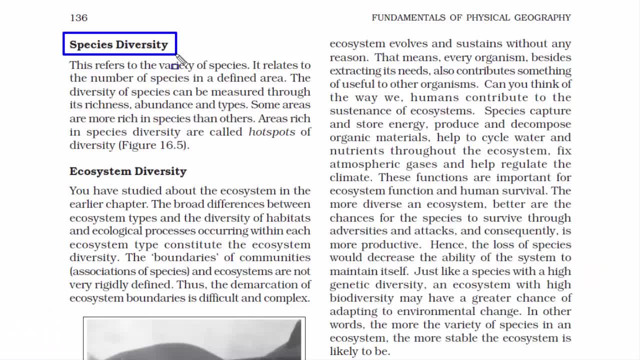 have evolved with time and many have disappeared with time. The unique part about the distribution is that it is spread all over the world unevenly, and the reason behind that is the physical and environmental factors that allow the organism to get its food to reproduce and to do all the things that the organism is meant to do, If you 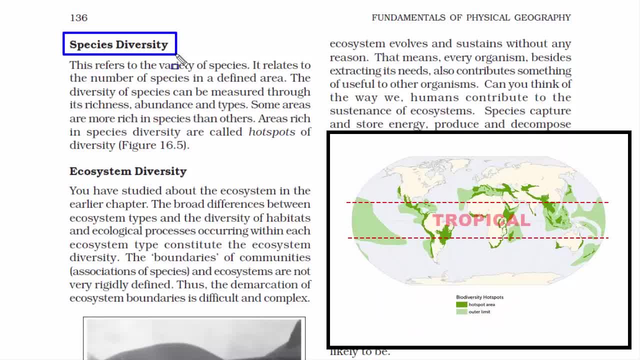 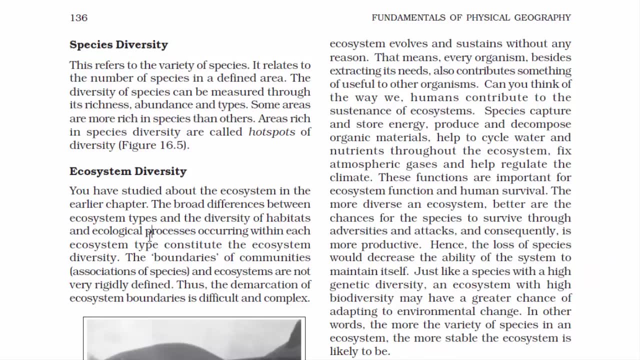 look at the world map. not every place on earth has the same environment. Because of this unevenness, there are some areas that are rich in species diversity. Those areas are called biodiversity hotspots of the world. We will learn more about them later in this chapter. And the third one is ecosystem diversity. If you look 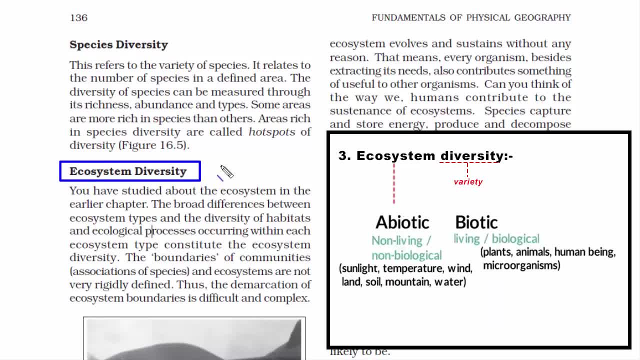 at the word ecosystem. it means when all the living things in a given area interact with each other and also with the non-living environment, In other words, direct contact between biotech and abiotic components of the environment. Here the biotech component includes all the living things, such as plants, animals and 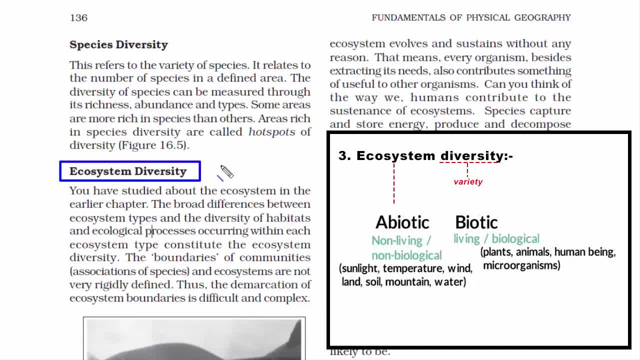 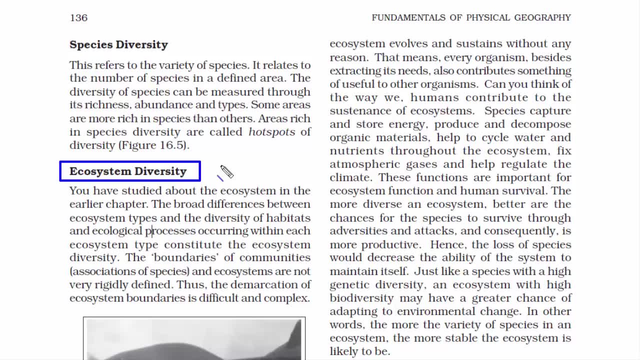 organisms, On the other hand, non-living, which is abiotic component, include climate, temperature, soil, sun, atmosphere, etc. Now, if you look at the word ecosystem diversity, it refers to the variation in the ecosystems within a geographical location, Let's say if this is a particular place. Now this particular. 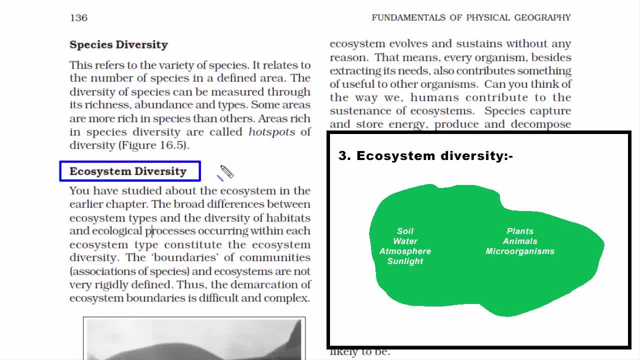 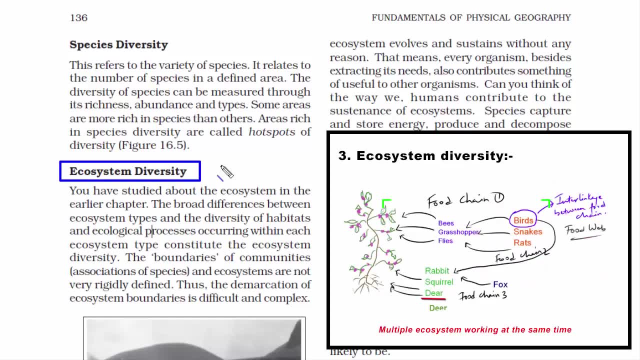 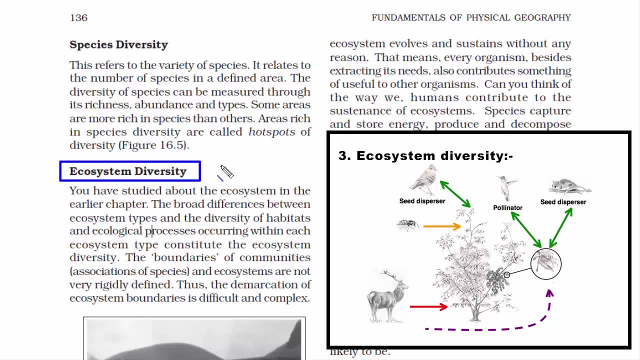 place has some non-living components, such as soil, water, atmosphere, sunlight. Now, within this place, there will be not just one, but many ecosystems that exist. There will be many different species of plants. animals and organisms interact with each other, as well as with the outer environment for food and mating purpose. This is what 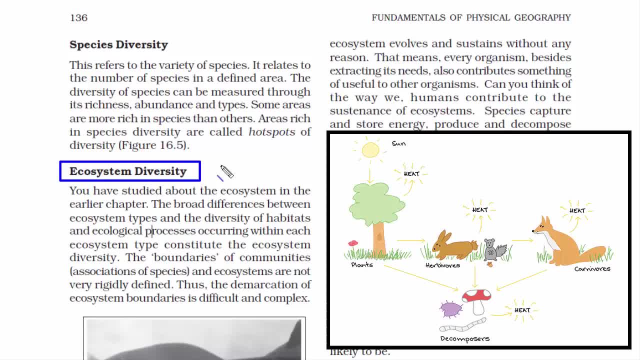 is the meaning of ecosystem diversity And, let's say, if you are somehow able to find out the different ecosystem that are working. still, it is going to be difficult to actually draw a line or create a boundary between two ecosystems, Why? Simply because their occurrence is natural, difficult and complex. We still don't know entirely about. 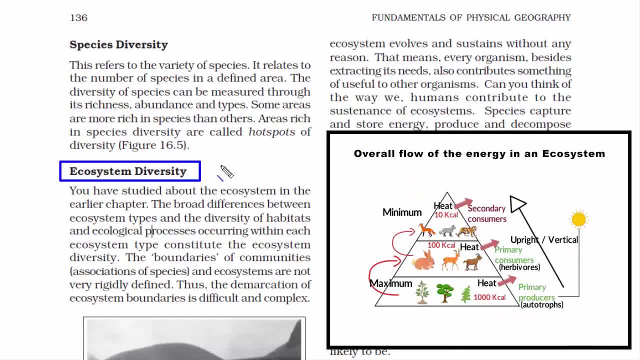 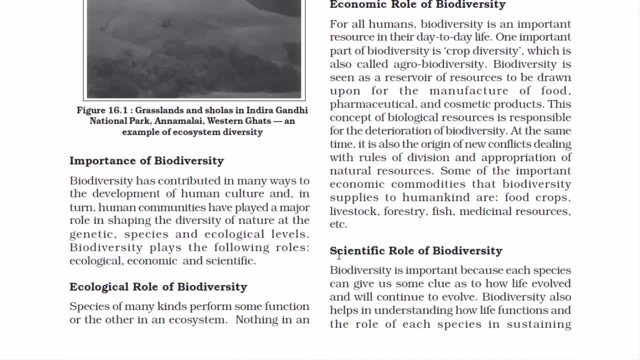 the interconnection of ecosystems and how the flow of energy, material and organisms across ecosystem boundaries take place. Alright, the next topic is the importance of biodiversity. So here it says: biodiversity plays the following roles: Ecological, economic and scientific. Now you may ask: how is it so? We will quickly. 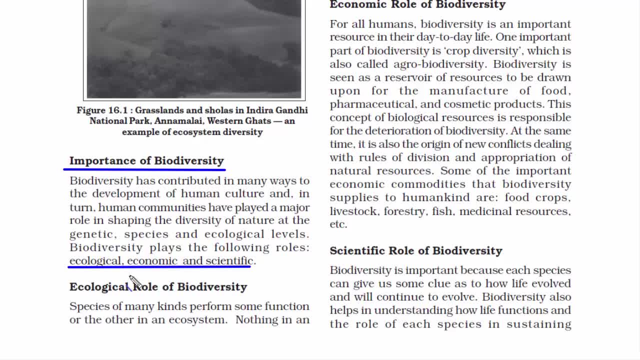 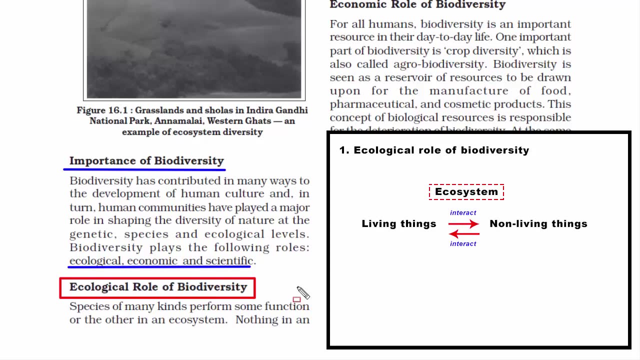 look at the ecological, economic and scientific roles of biodiversity. This way, it will also answer how biodiversity contributes to the development of human culture. Let's first look at the ecological role of biodiversity. We already know the meaning of ecosystem right, When all the living things in a given area interact with each other and also with the non-living things in a given area. We already know the meaning of ecosystem right. When all the living things in a given area interact with each other and also with the non-living thing in a given area, We may ask how does ecosystem and disease interact? 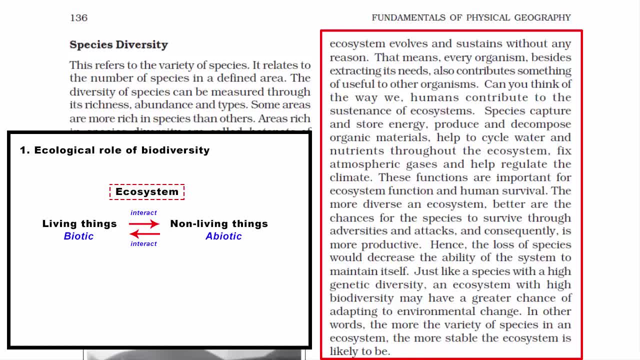 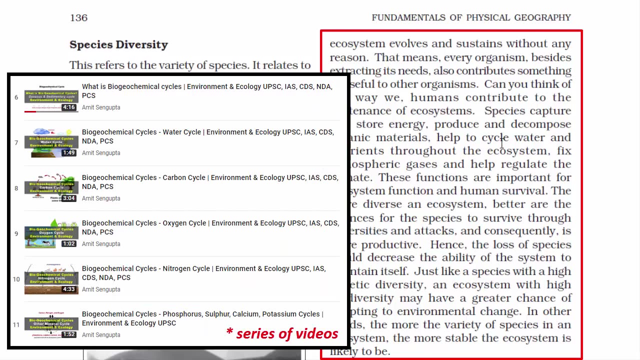 with each other and also with the organisms in the same environment. We already know they interact with each other and what kind of organisms they are. Someone may be controlling the wholeSet This- that video in the description. please have a look at it. After watching the video, you will get an. 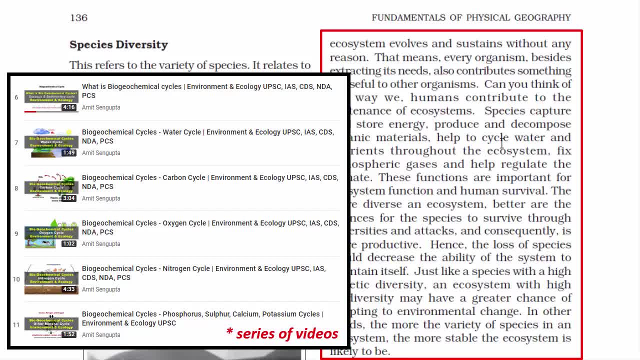 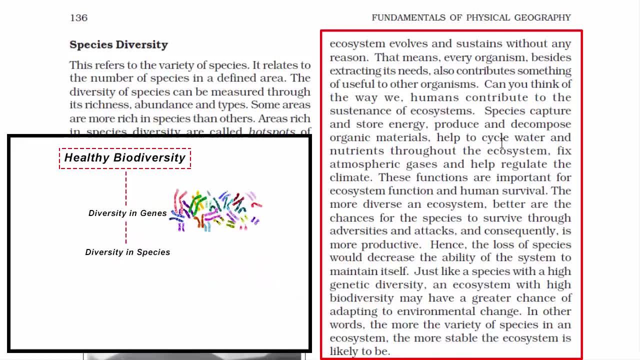 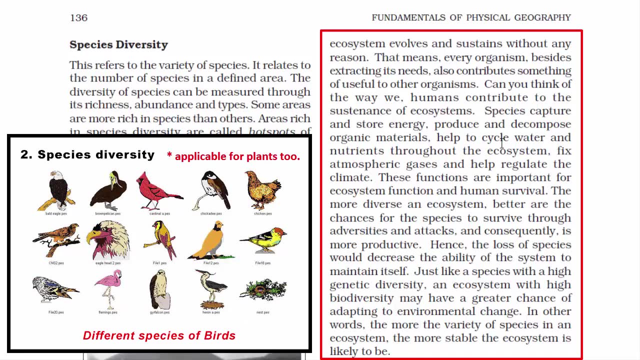 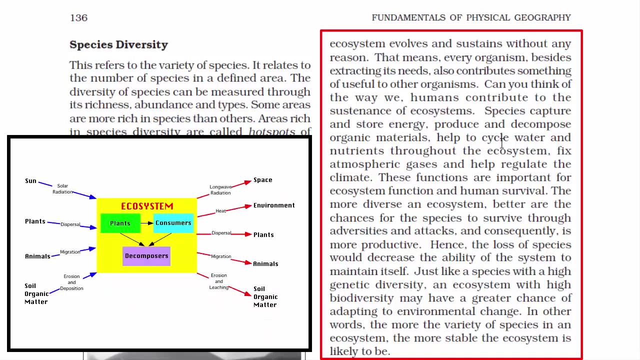 idea as to how organisms contribute to the ecosystem, which in turn supports human survival. So a healthy biodiversity provides diversity in genes, species and ecosystems. It will boost the ecosystem's productivity by providing a large number of plant and animal species. When an ecosystem's productivity increases, in other words, when there is an interaction between a 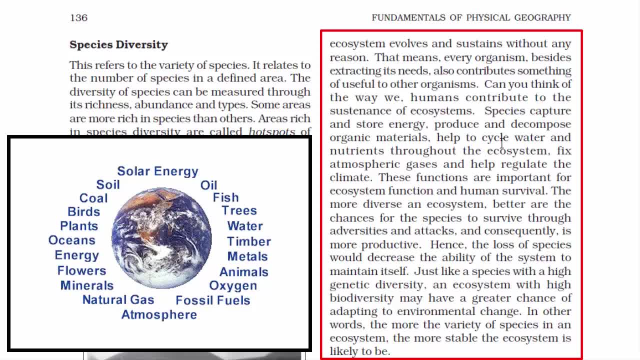 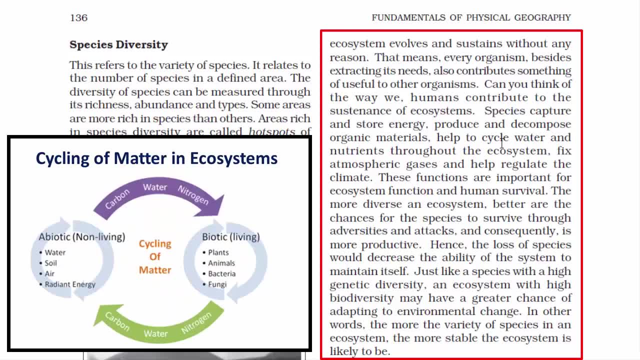 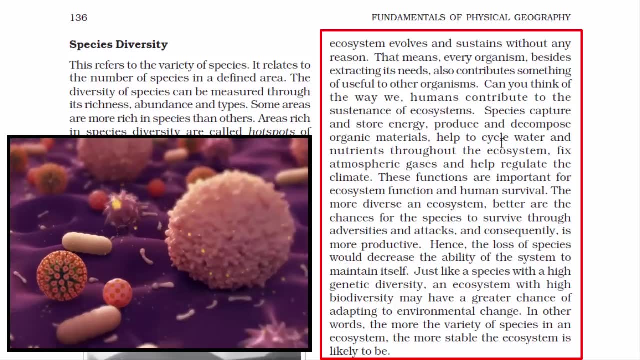 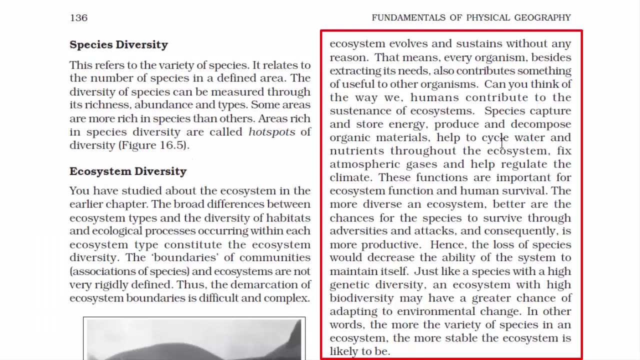 wide variety of organisms. that helps in replenishing future natural resources. It helps in increasing nutrient storage and recycling. Then it also contributes to climate stability. A rich ecosystem helps in breaking down pollution and absorbs it. Plants deploy multiple physiological, biochemical and molecular mechanisms to counter the effects of environmental. 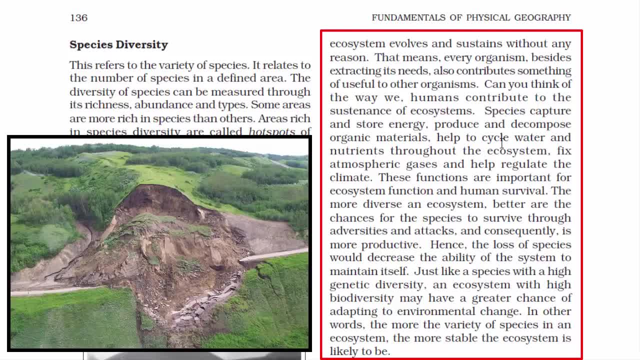 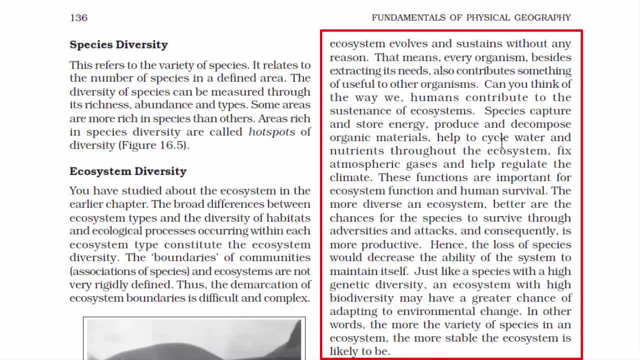 pollution. Plants deploy multiple physiological, biochemical and molecular mechanisms to counter the effects of environmental pollutants, Then it also reduces the occurrence of any natural calamity. The more the variety of species in an ecosystem, the more stable the ecosystem is likely to be. So all these are 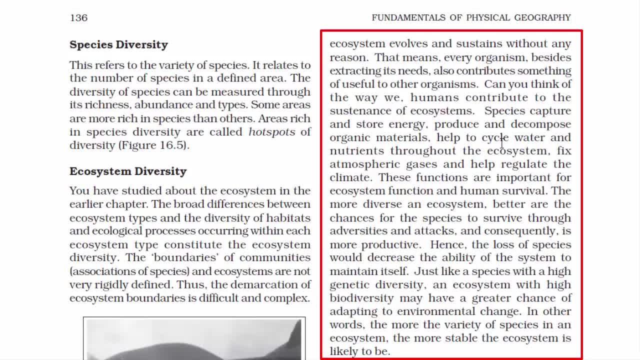 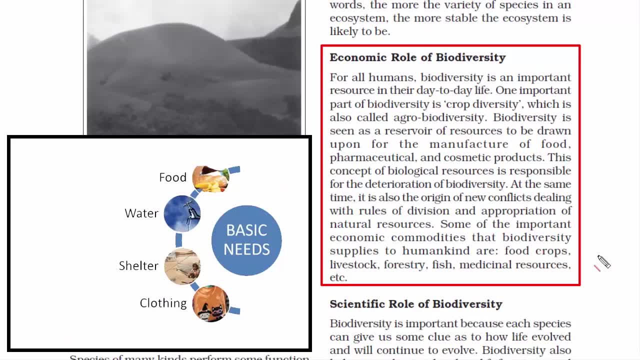 some notable ecological benefits of a rich biodiversity. Now let's look at the economic roles of biodiversity. Two essential basic human needs are food and livelihood security. That's how biodiversity is an important resource in a human's day-to-day life. Because of rich biodiversity, it gives humans the food it needs to survive. 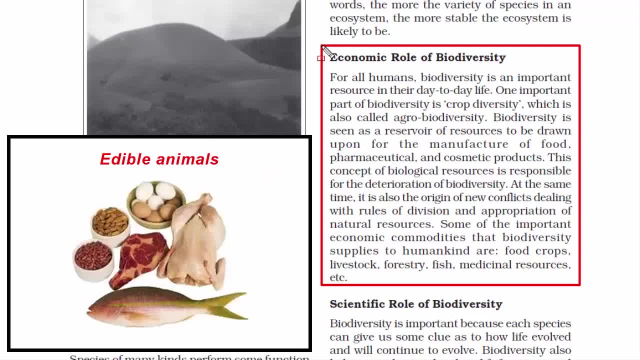 Although humans consume only a small number of plant and animal species, but those species depend on many others in order to survive. Therefore, biodiversity is important to food and agricultural systems. The right term to use here is crop diversity or agrobiodiversity. It contributes directly to food and livelihood security, nutrition and well. 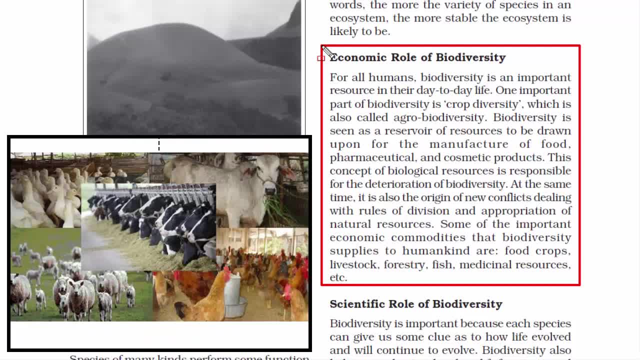 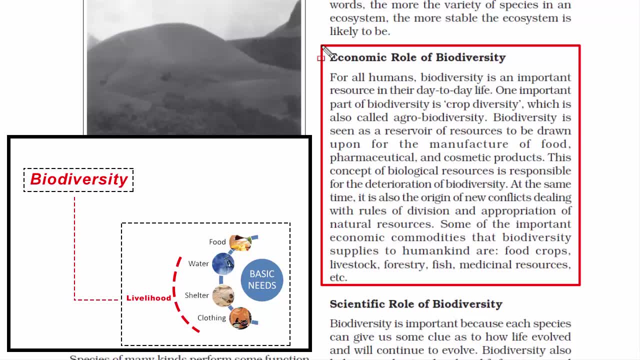 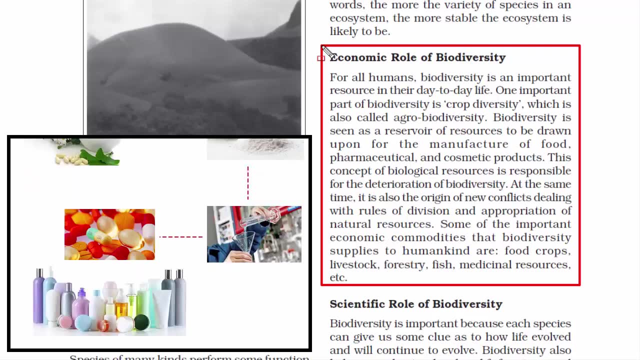 being by providing a variety of plant and animal, domestic as well as commercial usage. Biodiversity provides much of the basic necessities of food, water, clothing and shelter. The environment also provides raw material to the pharmaceutical, cosmetic and personal care industry. If you see many of the traditional and modern medicines, then personal care products. 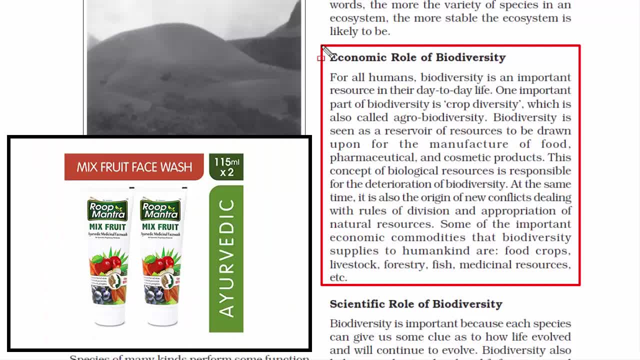 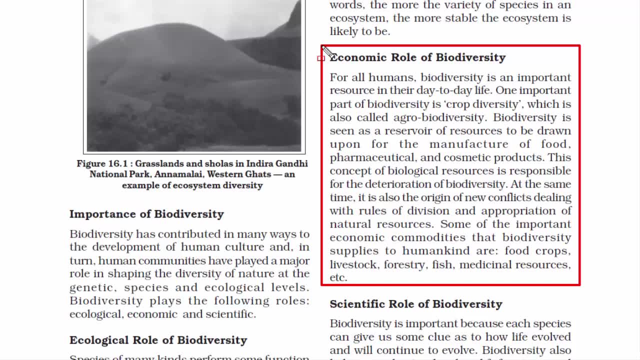 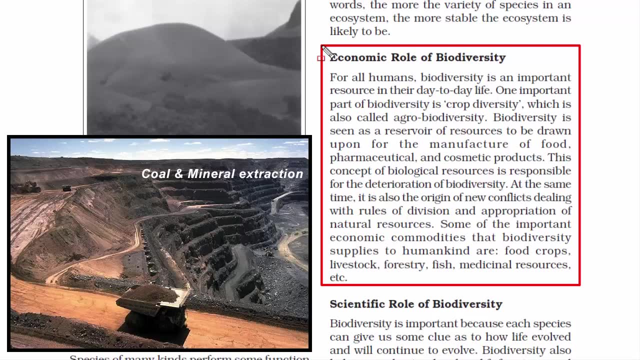 have raw materials and chemicals that are extracted from many species of plants and animals. Biodiversity loss diminishes the supplies of raw materials of these industries. The environment also provides the raw material for paper, construction and fuels. Although these all come under non-renewable sources, they are essential for human being, Forest and wetlands. 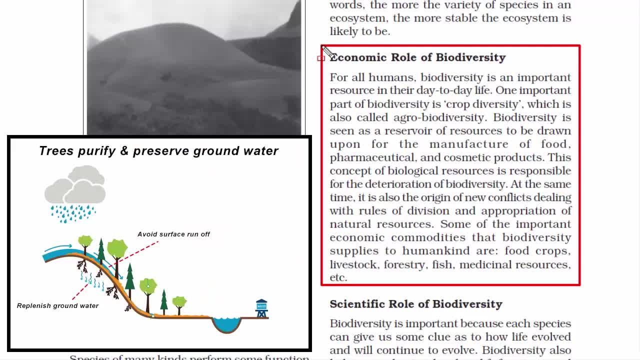 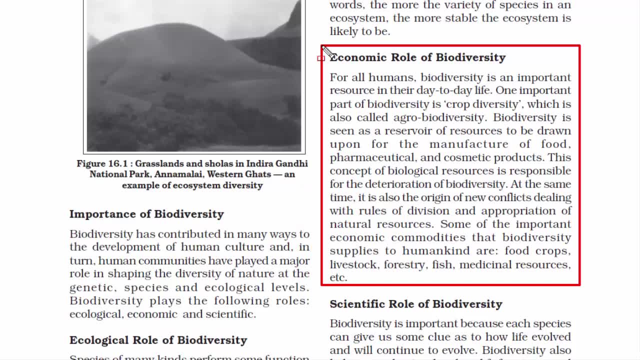 play a significant role in the well being and proper function of the hydrological cycle. It filters by absorbing pesticides and chemicals and removing harmful waste from water. Hence biodiversity works like natural chemical detoxification. So, in a nutshell, some of the important economic commodities that biodiversity supplies to. 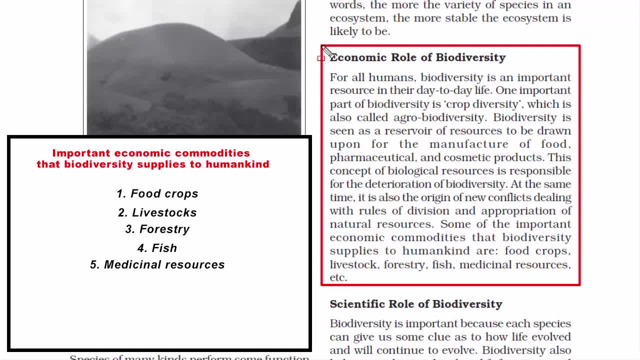 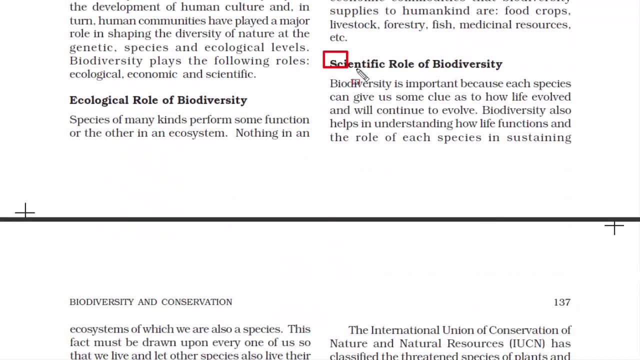 humankind are food crops, livestock, forestry, fish, medicinal resources, etc. Now we will look at the Scientific role of biodiversity. Biodiversity provides important resources for medical research By studying and conducting research on plant and wildlife anatomy, physiology and biochemistry. 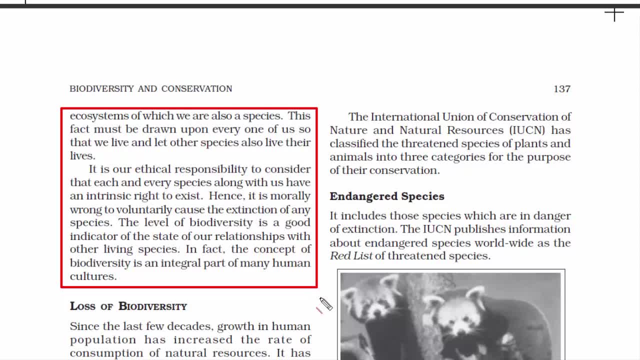 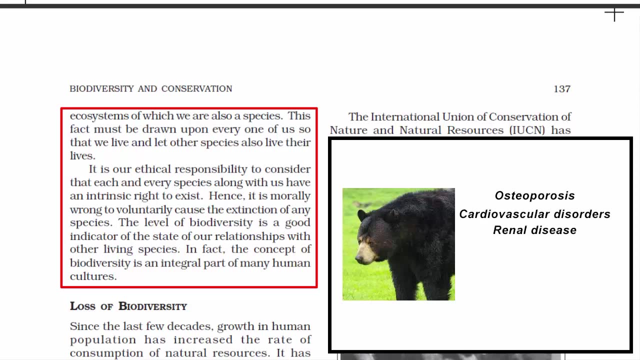 It can lead to an important development in human medicine and it can give us some clue as to how life evolved and will continue to evolve. Some of the species which are important for medical science include bears. It can provide an insight into osteoporosis, cardiovascular disorders, renal disease and. 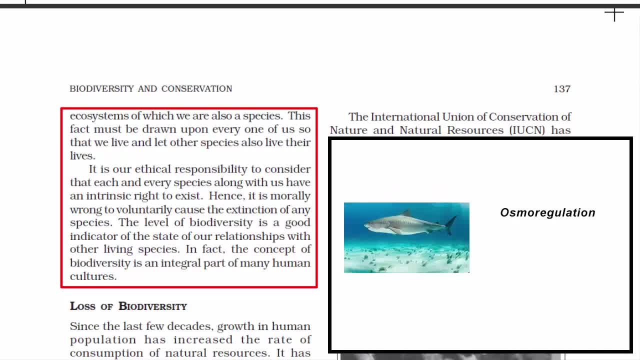 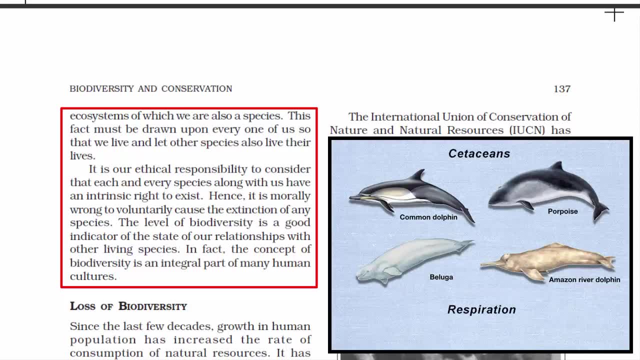 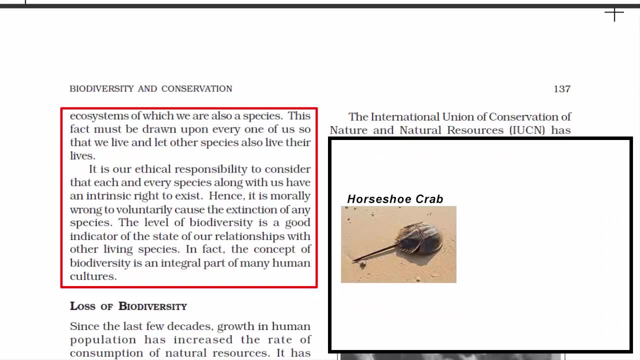 diabetes. Then we have sharks: Through their anatomy we can study osmoregulation and immunology. Then we have cetaceans: It provides an insight into respiration and treatments for divers suffering from decompression sickness. And then we have horseshoe crabs. 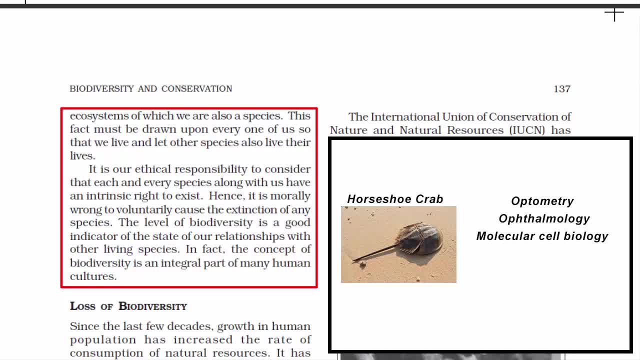 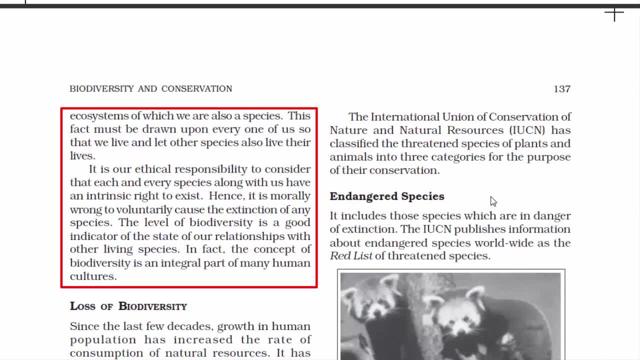 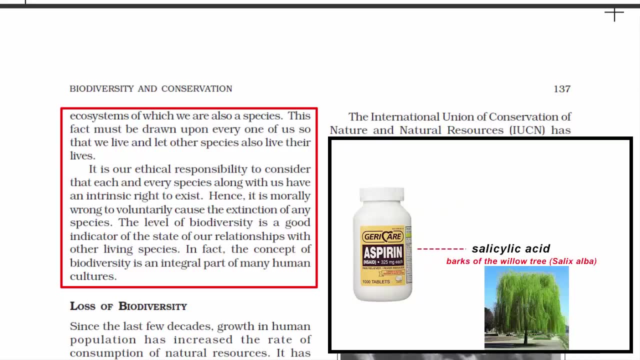 Study of them can provide insights into optometry, ophthalmology and molecular cell biology. Even plants contribute to many of the modern medicine. If you see aspirin Which is used to treat cancer, To treat pain, fever or inflammation, It contains salicylic acid. 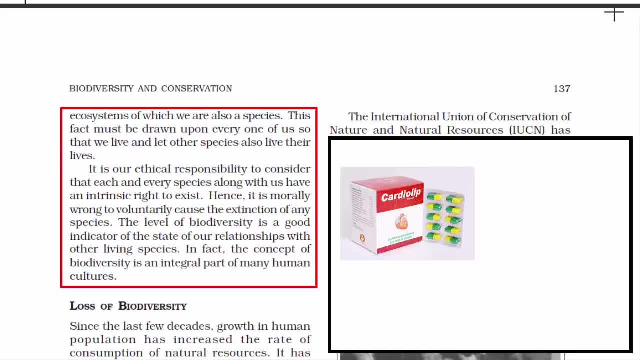 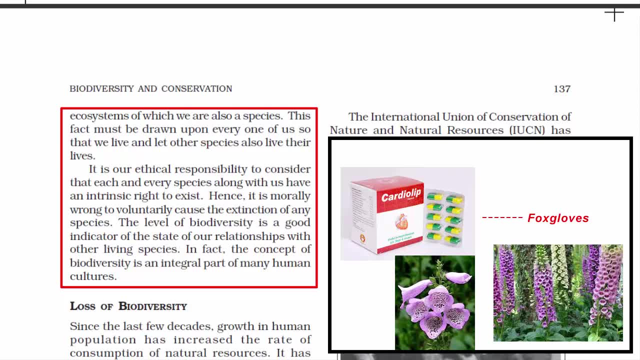 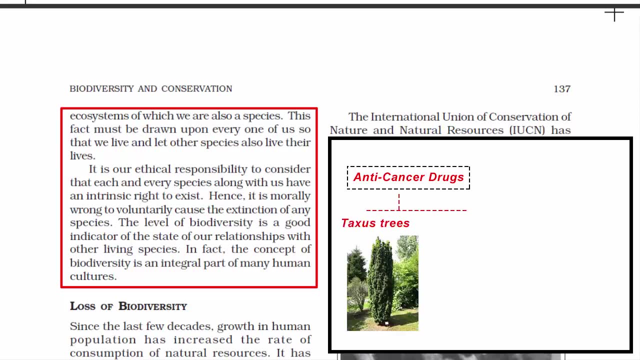 Which is extracted from barks of the willow tree. Then we have heart medicines Which are prescribed for any sort of heart failure. The content of those medicines are extracted from a plant called foxgloves. Then anti-cancer drugs contain ingredients from taxus trees and camptotheca plants. 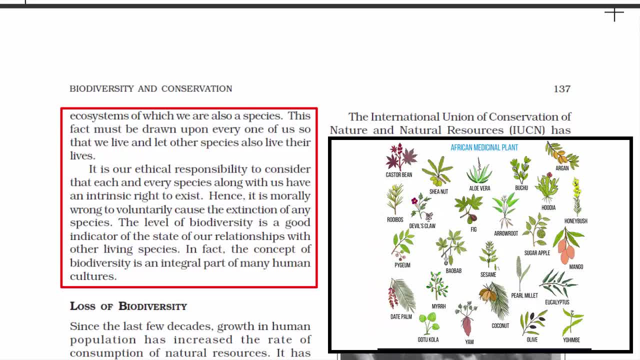 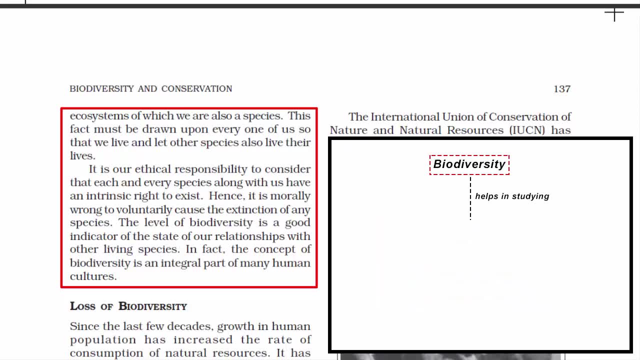 And there are many more potentially important plants That have yet to be investigated or discovered. So you see, biodiversity provides a great opportunity to study and conduct research on many different species of plants and animals, Which is not only beneficial to the human being, But it also helps in understanding the environment and how to maintain its sustainability. for 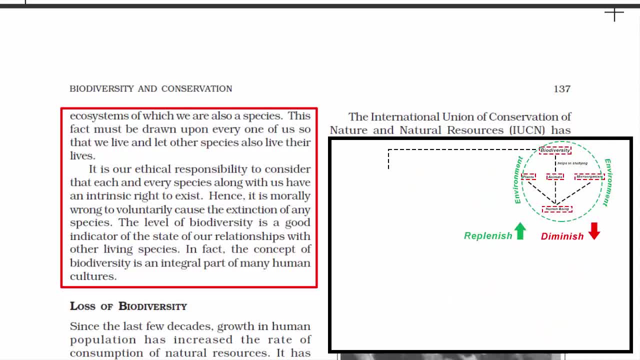 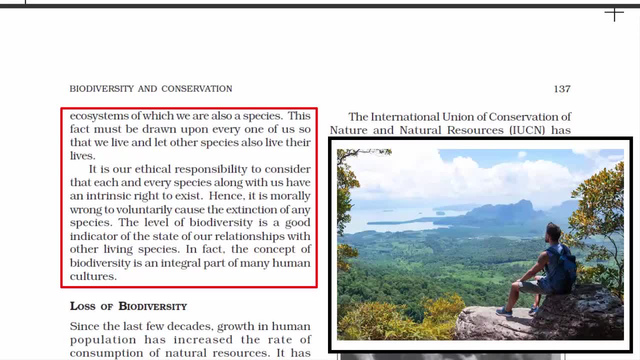 future resources, And that's how the concept of biodiversity is an integral part of many human cultures. So once you understand that biodiversity has the solution to lot of the human's health problem, Then it becomes a question of morality and ethics. Therefore, it is wrong to voluntarily cause the extinction of any species due to human. 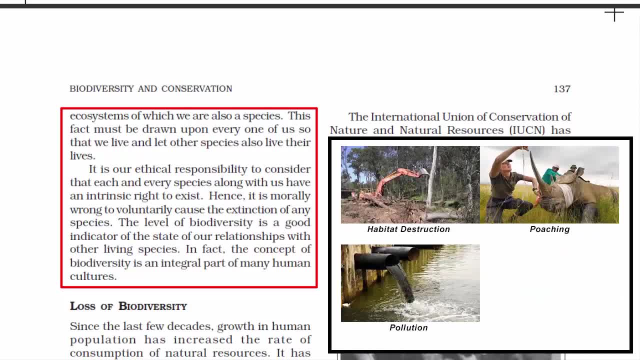 caused activities like habitat destruction, poaching, pollution, introducing invasive species that act as new predators and food competitors. You see, to a lot extent humans have always altered their environment And that's why we have to understand that biodiversity has the solution to a lot of. 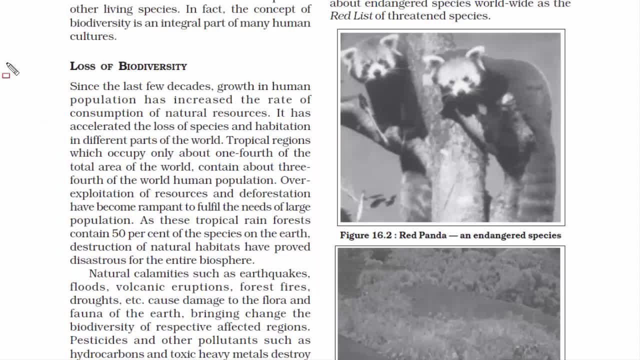 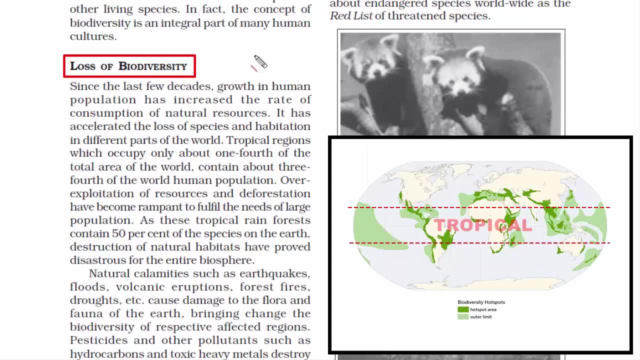 the human health problems. So what is it that helps human beings bites environment. Let us go to the next topic: loss of biodiversity. If you look at the world map, we know the tropical region is rich in biodiversity. That is why, if you see the biodiversity hotspots of the world, they are located only in tropical 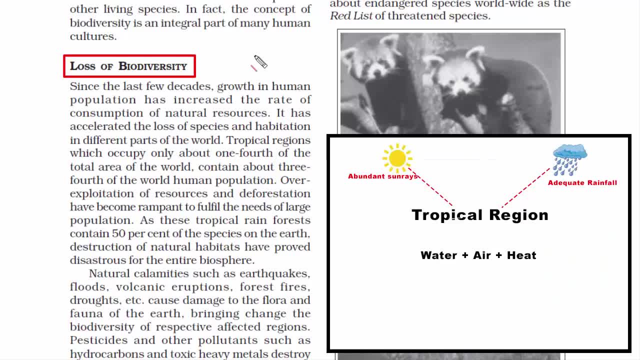 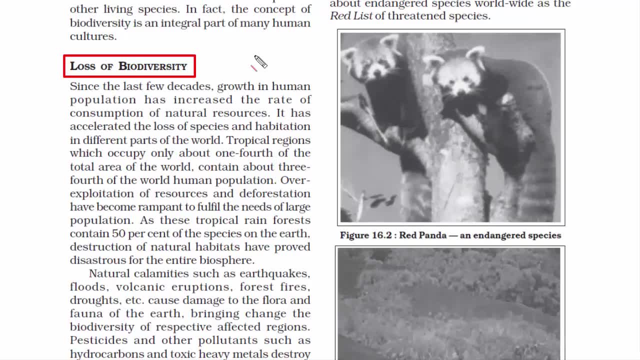 regions, Because in this region, you will find ample amount of sunshine as well as rainfall, Which is ideal for the existence of many plants and animal species. Now, you shouldn't think of that as an impossible task. In fact, it's not impossible. 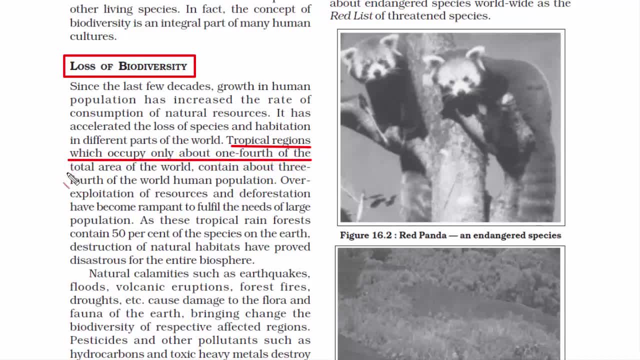 is also the place where most of the world human population reside. I think around 40% of the world population live in the tropical region. Again, the reason is suitable temperature and climatic condition, which has enormous social and health benefits on humans. 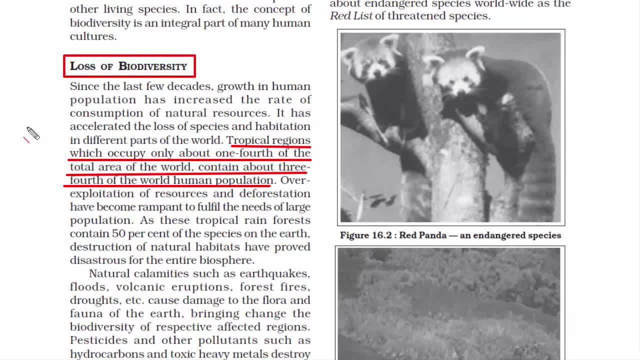 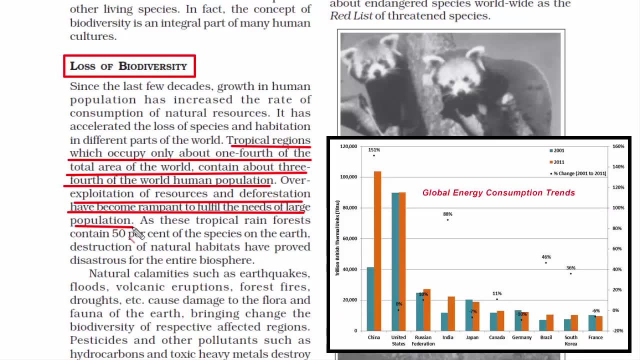 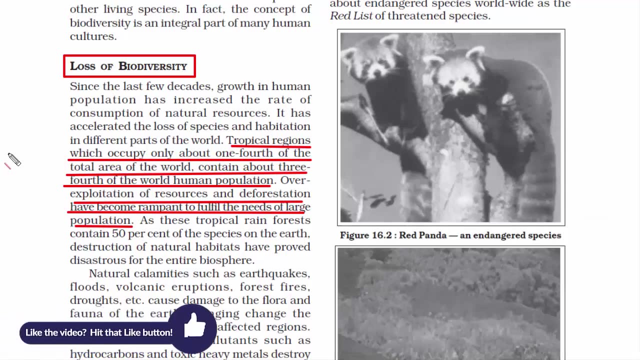 With so much of the human population residing in tropical region, areas need to be cleared. that means nature has to be destroyed. Then humans have demands in the form of consumption. With that comes great demand in consumption of natural resources. Sometimes it leads to overconsumption or exploitation of resources. 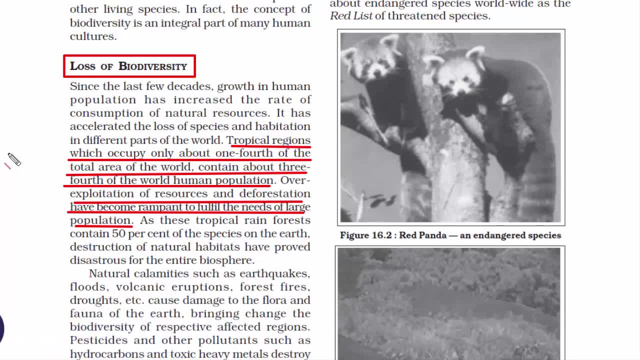 And that's when natural habitats are destroyed. When we mess with nature, nature sometimes hits back in the form of natural calamities such as earthquakes, floods, volcanic eruptions, forest fires, droughts, etc. So any kind of change, be it through natural calamities, 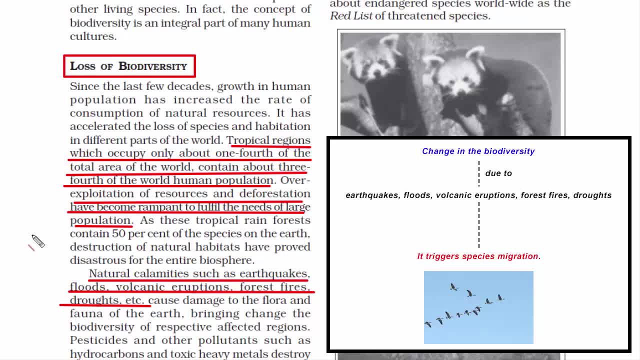 or human activities will bring change in the biodiversity of the affected regions, Because the word biodiversity means biological diversity, meaning a variety of living organisms. These organisms interact as well as depend on each other. That's how ecosystems exist Now, if one species is dependent on another species for food and mating, 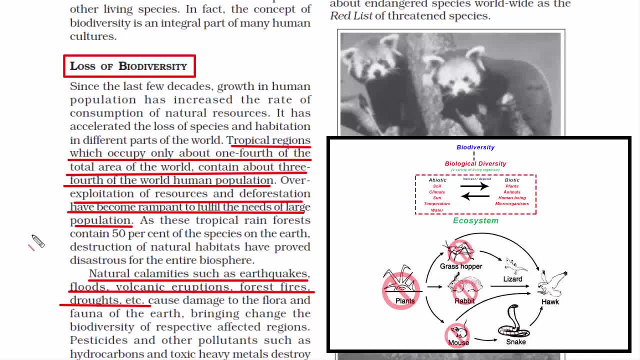 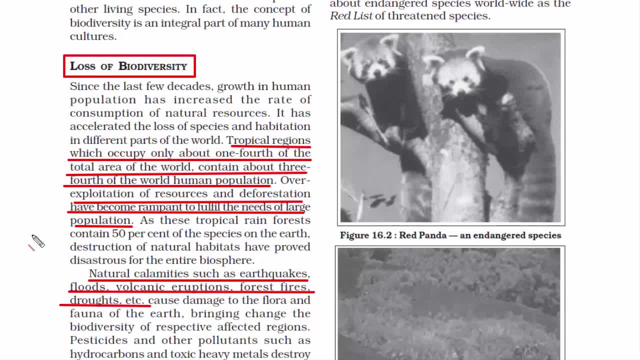 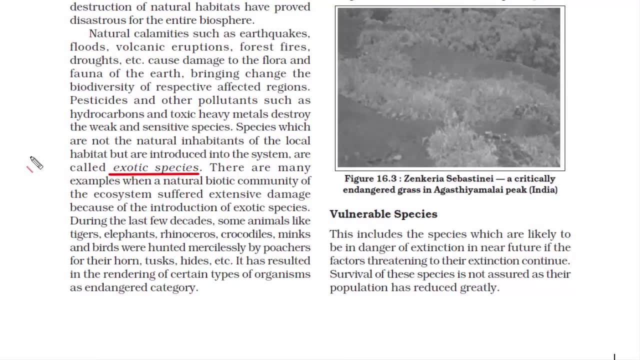 and if that primary species goes extinct or disappears, then obviously it will affect other species. That's how there will be a change in the biodiversity. There is this term called exotic species. Let's quickly understand this. The word exotic means unusual and exciting. 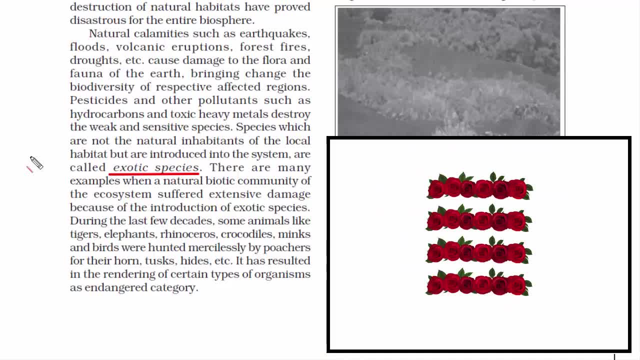 Now, let's say there is a garden and you have all red colour roses growing in that garden. Because these species of flowers are natural inhabitants, Your garden is their local habitat. That's why there are plenty of red roses. That's why there are plenty of red roses. 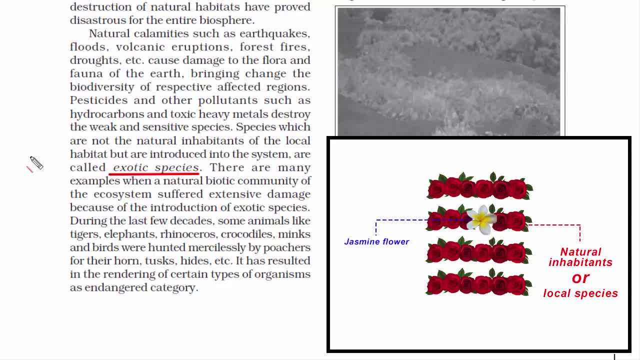 Now, all of a sudden, you notice a jasmine plant, Basically a white coloured, different looking flower plant. Now, this different looking plant is called an exotic species Because it's unusual and different in your garden. So you have so many rose plants. 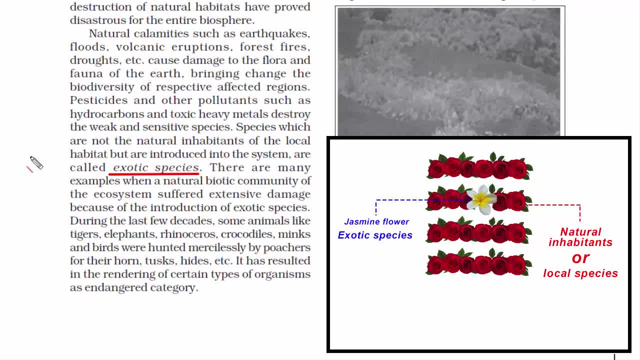 and all of a sudden there is one jasmine plant. So the rose plants become local species and the jasmine plant becomes exotic species. That is what is the meaning of exotic species. This is applicable for any kind of living organism. It can be an amphibian plant, insect, fish, fungus, bacteria. 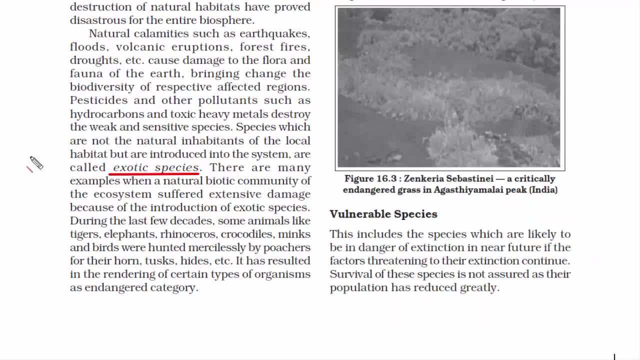 or even an organism's seeds or eggs, Species which are not the natural inhabitants of the local habitat but are introduced into the system. Now, any species that lives outside its natural habitat have various effects on the local ecosystem. There are many ways these species get trapped in the ecosystem. 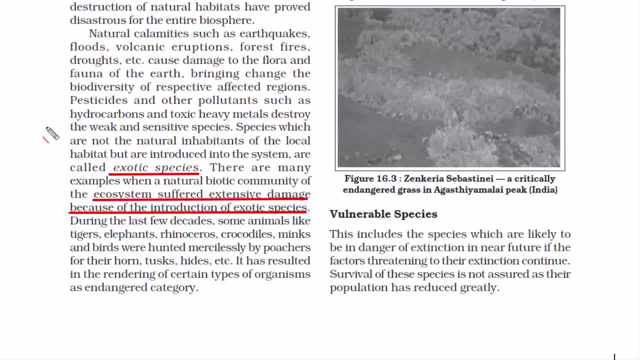 There are many ways these species get trapped in the ecosystem. There are many ways these species get trapped in the ecosystem. They are transported from one place to another. Sometimes it's through human activities. Human beings travel all around the world. Many times they carry flowers, herbs. 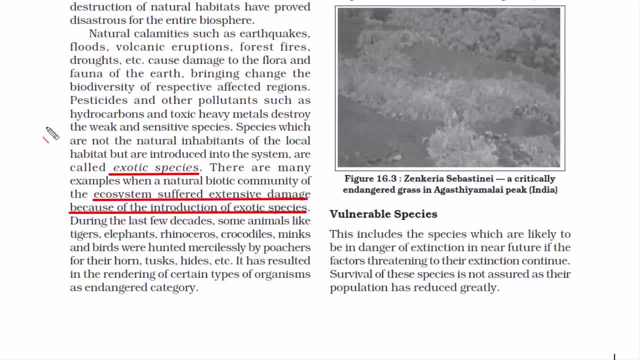 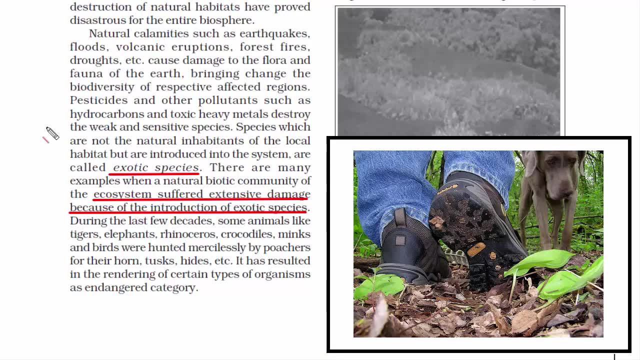 unintentionally and it escapes into the wild and become invasive. You must look at your shoes or socks when traveling. You will notice that your shoe collects some patches of plants and weeds And, let's say, the next day you fly and you wear the same shoe. 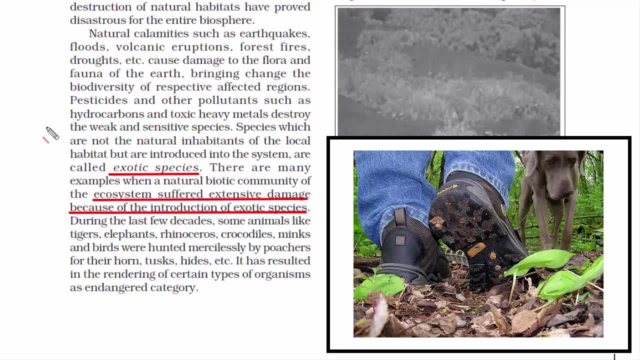 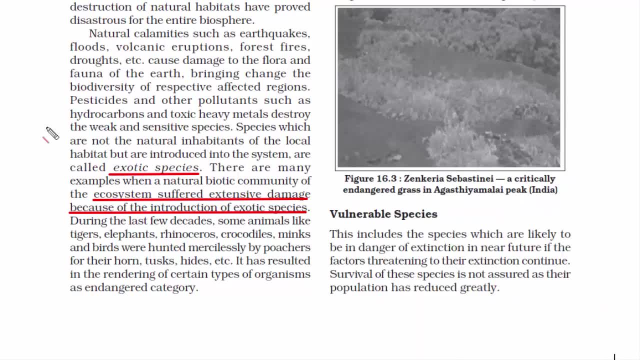 Those sample of plants and weeds drop along the way from your shoes. Those sample of plants and weeds drop along the way from your shoes. This way, you successfully transported a plant species from its natural habitat. Even birds are responsible for transporting species from one place to another. 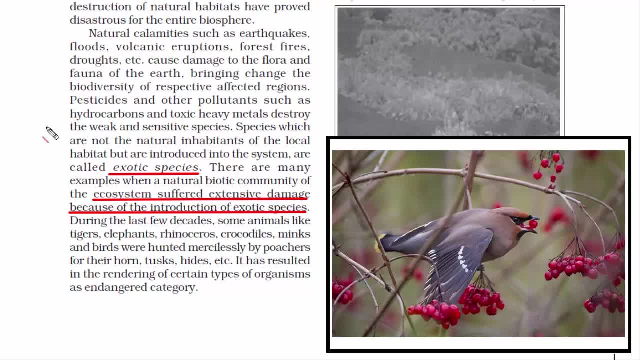 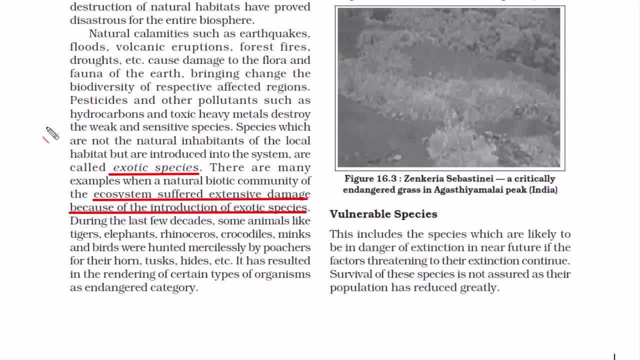 They carry seeds to a new location. Along the way, the bird may drop a few seeds, allowing them to reach new spots far from the parent plants. So you see, all these are ways- and there are many more- through which exotic species are introduced in an ecosystem. 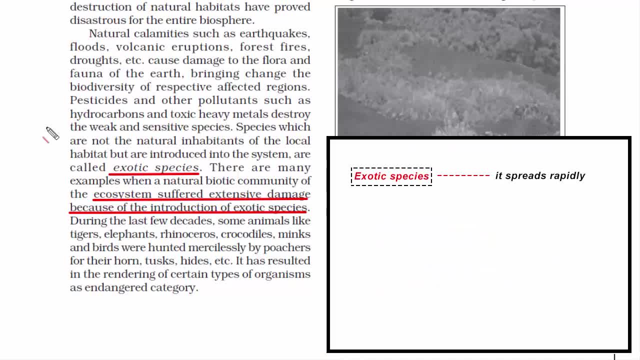 So you see, all these are ways- and there are many more- through which exotic species are introduced in an ecosystem. exotic species is that it spreads rapidly in the new habitat. It is generally aggressive and since it's a new species, therefore it doesn't have any predator. No other species can compete. 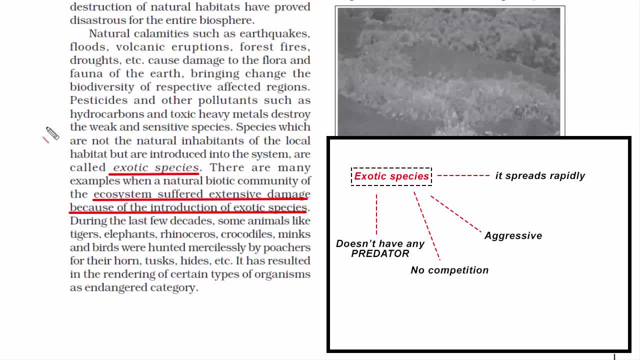 with them in their new home and that gives them an advantage. They can cause harm to the environment. it can then has an effect on the economy and ultimately to human health. If you look at some of the recent infectious disease like swine flu, ebola, dengue fever, these are some various. 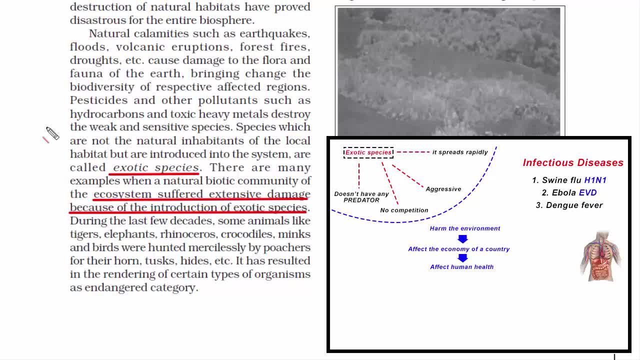 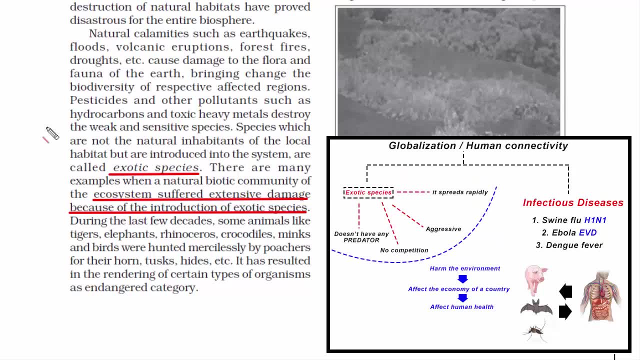 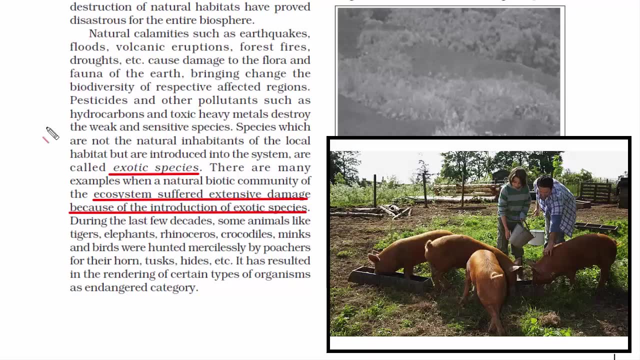 contagious diseases caused by viruses that spread from animals to people and vice versa. That means exotic species and infectious diseases are becoming more prevalent and widespread with increased connectivity and globalization. As people increase their contact with wildlife, their habitat and domestic animals, it's more likely that 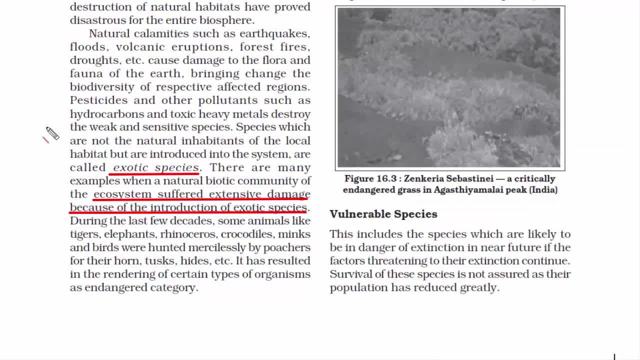 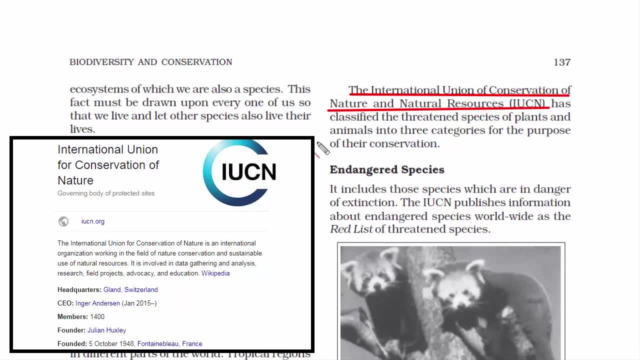 diseases like swine flu, ebola and dengue fever will spread to the environment. There is an organization called the International Union for the Conservation of Nature. The short form is IUCN Now. this organization works in the field of nature conservation. 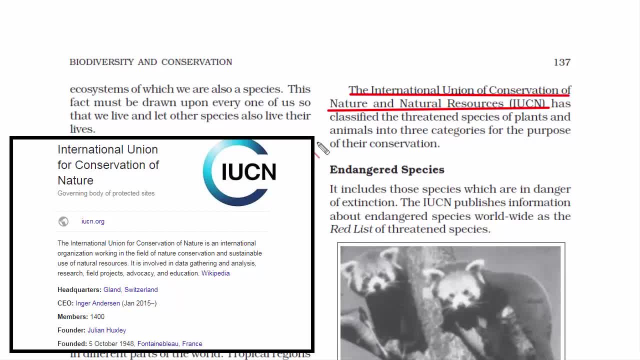 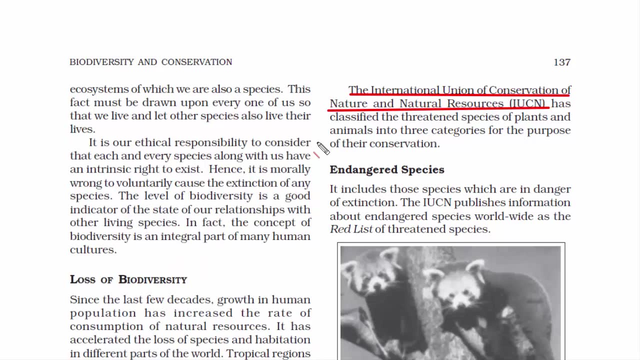 Basically, they collect data and analyze it, They do research, they have many projects through that they educate. So this organization provides knowledge, information and tools to the public, private and government organization So that strong steps are taken towards nature conservation. If nature is conserved and 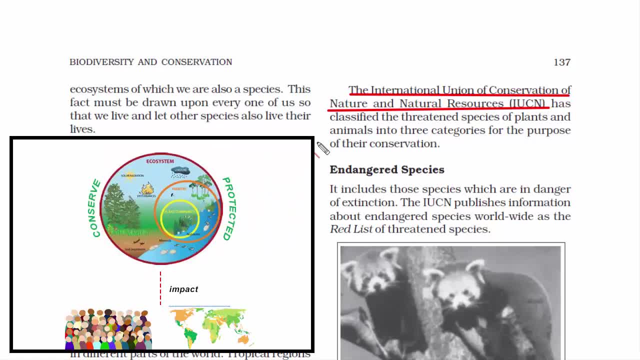 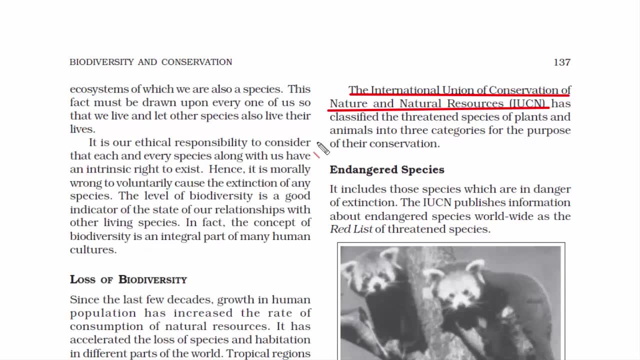 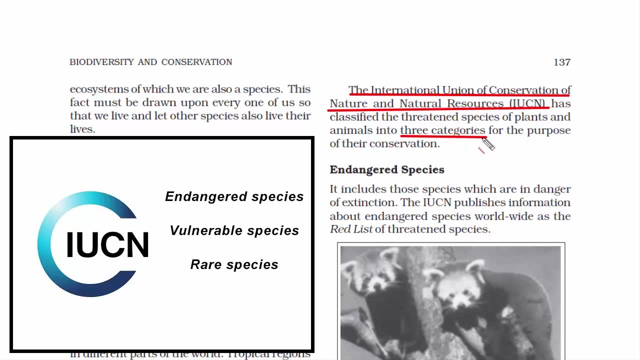 protected, then it has a huge impact on the economic development of humans as well as nations, Now that you have a little understanding of this organization. so what this organization does is it classifies those plants and animal species which are on the verge of getting extinct. 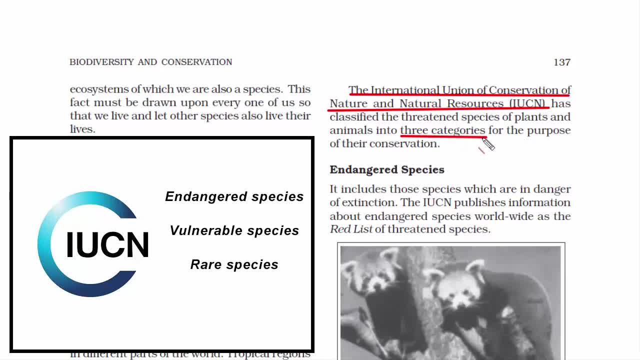 So they have classified them into three categories. We'll look through each of these three categories quickly. The first one is endangered species. By the word endangered you can easily figure out that it's talking about those species of plants and animal which are in danger of extinction. In simple terms, 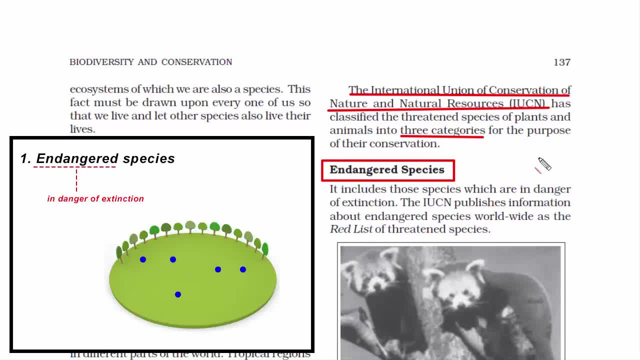 their number is so small that you will not see them in near future. Therefore, you cannot hurt them, kill them or injure them. The purpose behind assigning them the endangered word is to help, preserve and assist these species and their ecosystem to survive. So let's get started. 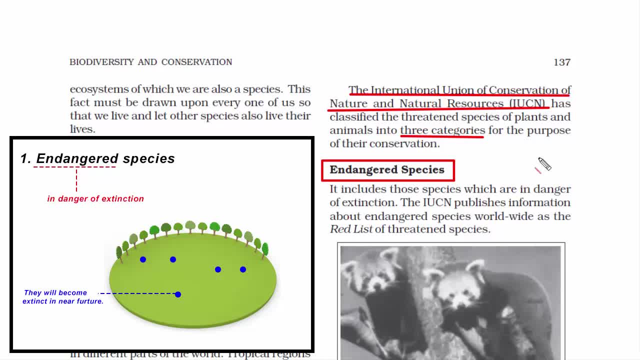 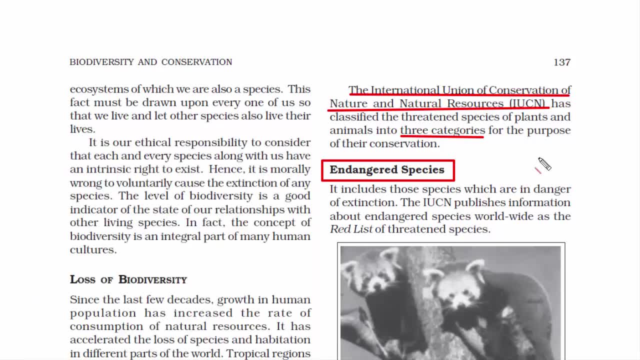 The first category is endangered species. By the word endangered you can easily figure out the sobrevivor species So that they might come a time when they recover and their numbers may increase and they survive extinction. The IUCN publishes information about endangered species worldwide. 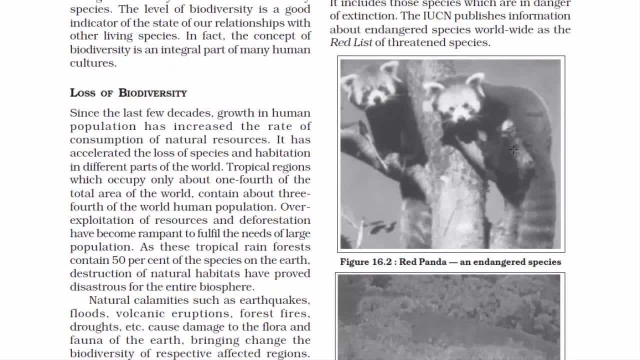 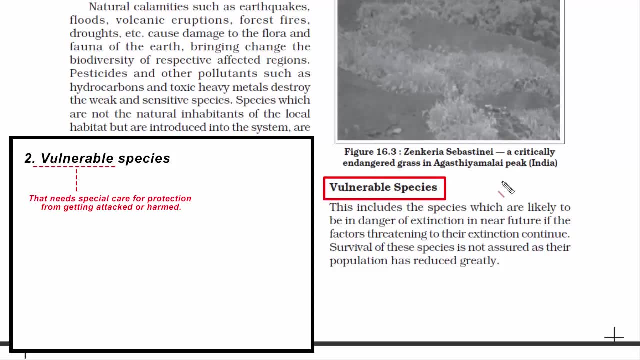 as the red list of threatened species. The second one is vulnerable species. Now, when you look at the word vulnerable, it means something that needs special care for protection from getting attacked or harmed. That's why, under this category, we will call it endangered species. The second category is: 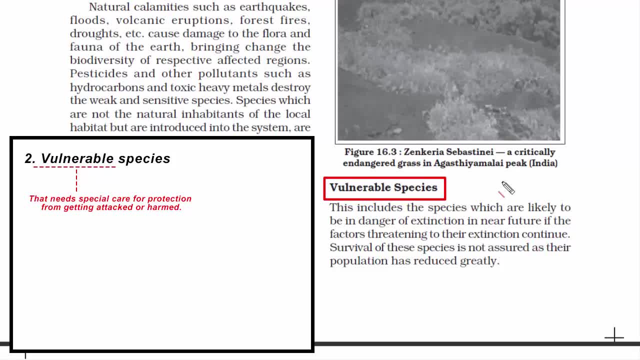 They include species which are likely to be in danger of extinction in the near future if the factors threatening to their extinction continue. There is a very thin line between vulnerable species and endangered species. Vulnerable species are those species whose numbers are falling drastically and they will vanish from the face of the earth if they are not given any special care. 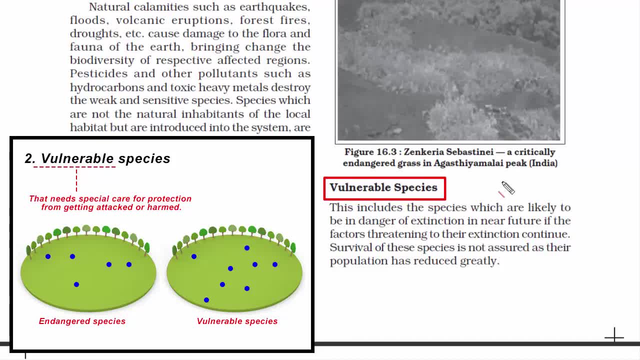 But the endangered species are those species which are almost on the verge of getting vanished from the face of the earth. So the subtle difference between both the category depends on the population of the species. The population of endangered species is already so less that they are bound to disappear if proper steps are not taken. 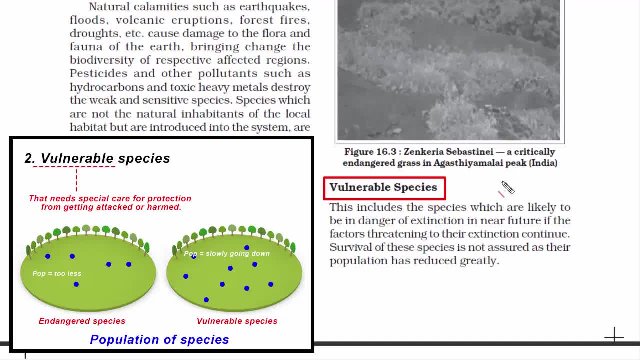 Whereas on the other hand, among the vulnerable species the population is not so less, but then there is also a fear that their population will reduce greatly if nothing is done. But then, if you see, if proper steps are not taken, then the vulnerable species are very close to becoming endangered species. 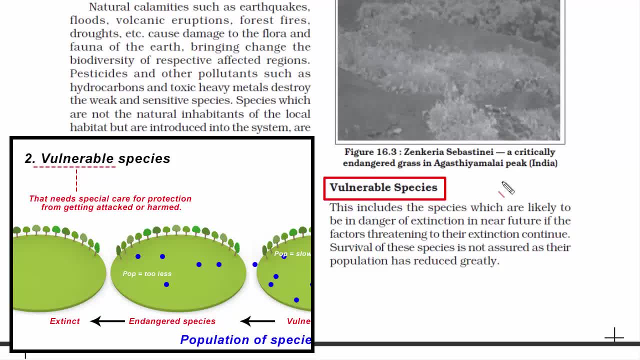 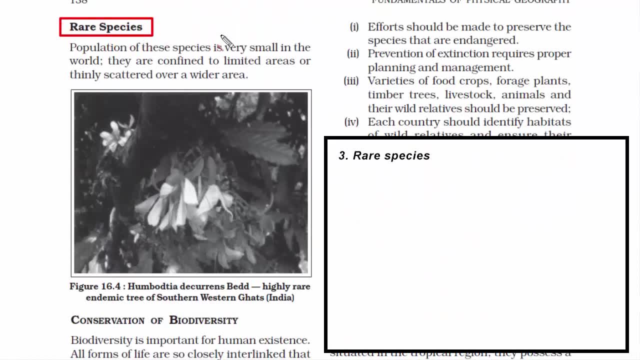 Similarly endangered species are very close to becoming extinct species if no proper steps are taken. The third category is rare species. I think by looking at the word rare you can easily figure out that the population of these species is very less in the world. 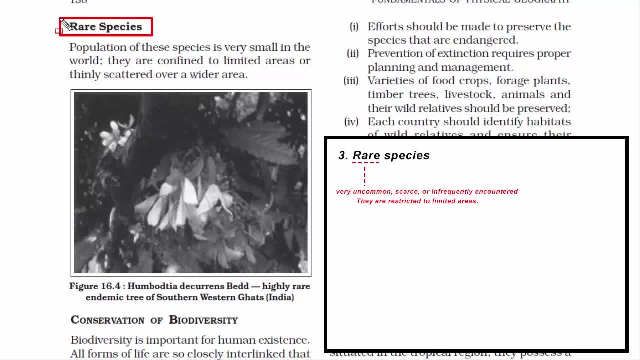 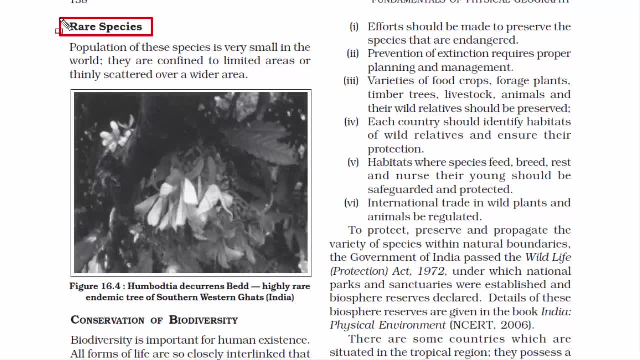 And they are also not seen everywhere. They are restricted to limited areas, or in other words, they are not widely seen, They are not easily spread. For example, let's say, an organism is found only on an island. Or let's say a particular species is found at a place where the temperature is suitable. 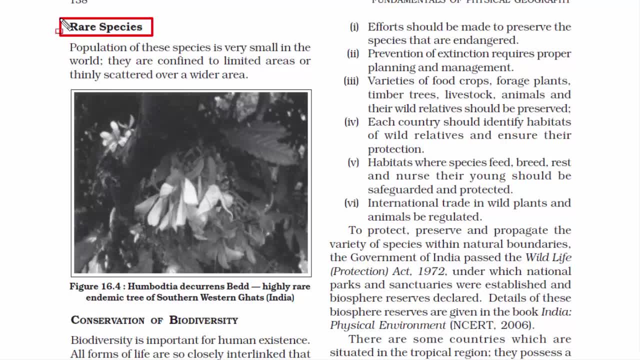 and anything beyond that temperature range is unsuitable. You see, that particular location, along with the location's climate and the environment, becomes a habitat for that species. So naturally you will not find the animal or plant anywhere else apart from that location. 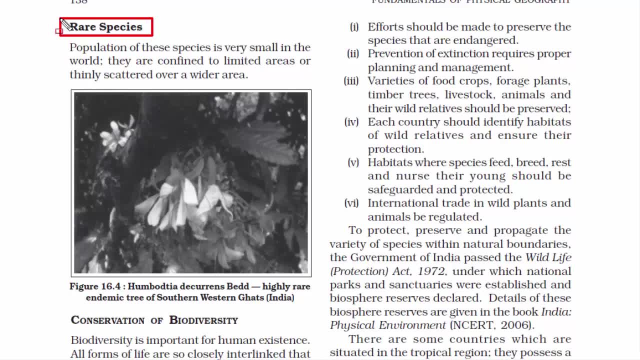 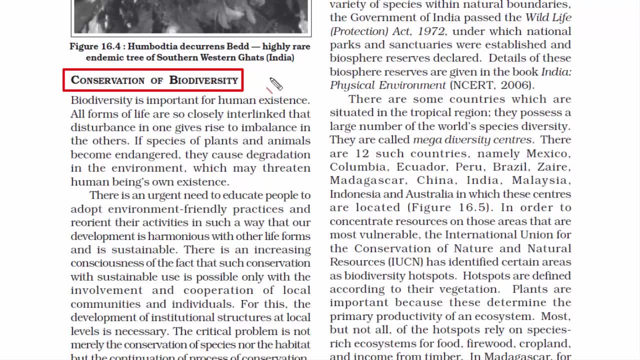 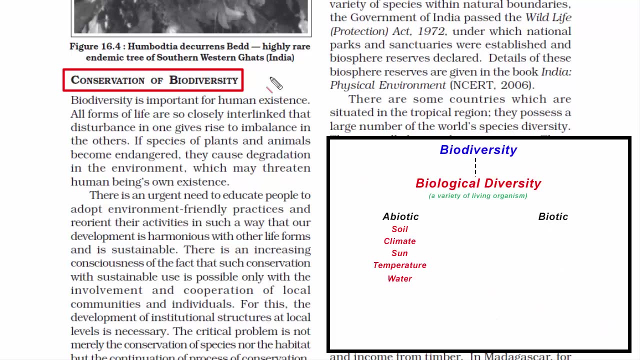 That's how endangered species are. That's how it becomes a rare species. Let's go to the final topic of this chapter: conservation of biodiversity. In this chapter, I have explained about the importance of biodiversity. I also told you the meaning of the word biodiversity. 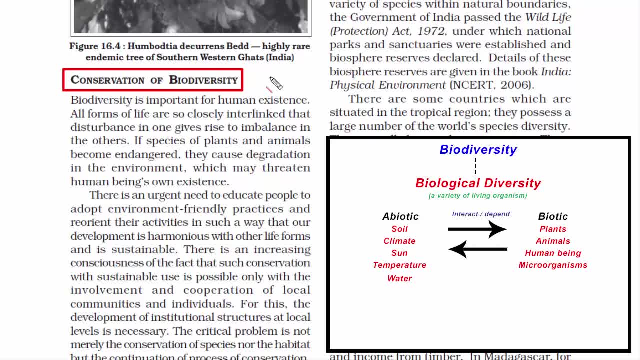 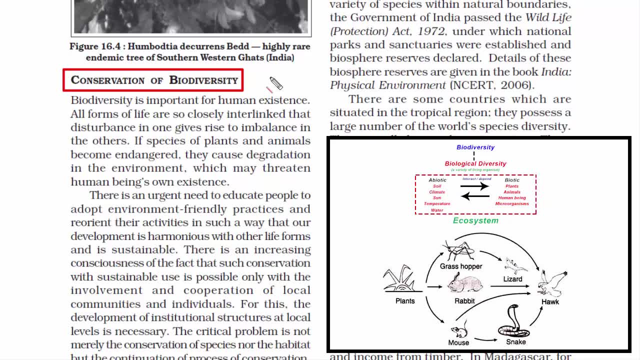 It means biological diversity or a variety of living organisms. These organisms interact as well as depend on each other. That's how ecosystems exist Now, if one species is dependent on another species for food and mating, and if that primary species goes extinct or disappears, 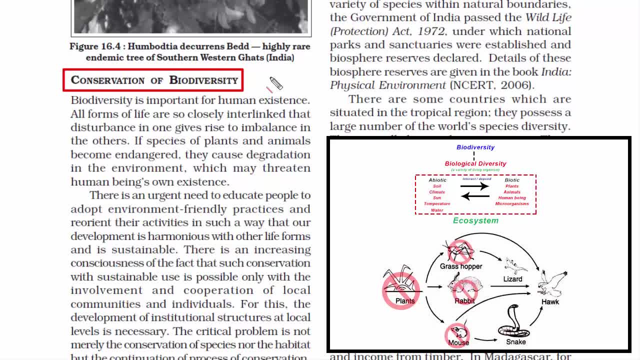 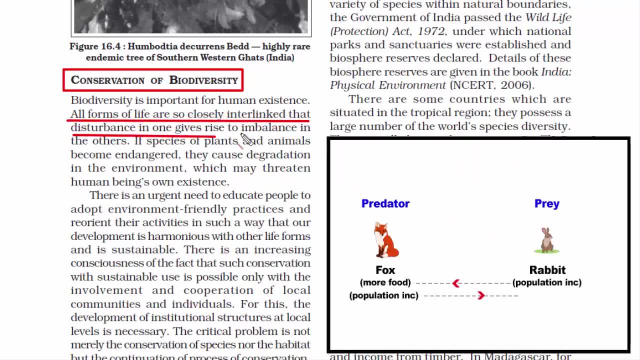 then obviously it will affect other species down the line, And that's what is written over here. All forms of life are so closely interlinked that disturbance in one gives rise to imbalance in the others. Human population has been the main reason behind overconsumption. 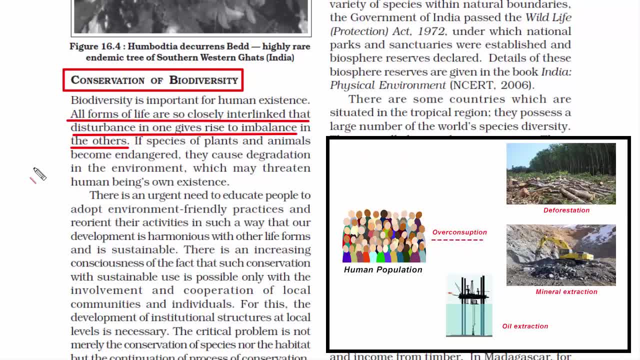 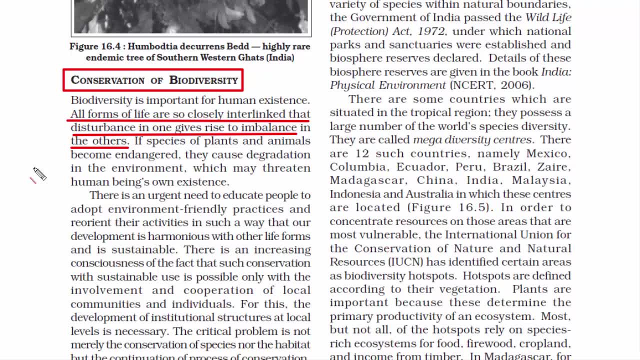 as well as the exploitation of natural resources, Many natural habitats have been destroyed. In return, nature heads back in the form of natural calamities such as earthquakes, floods, volcanic eruptions, forest fires, droughts, etc. That means any harm to the biodiversity will threaten human beings' own existence. 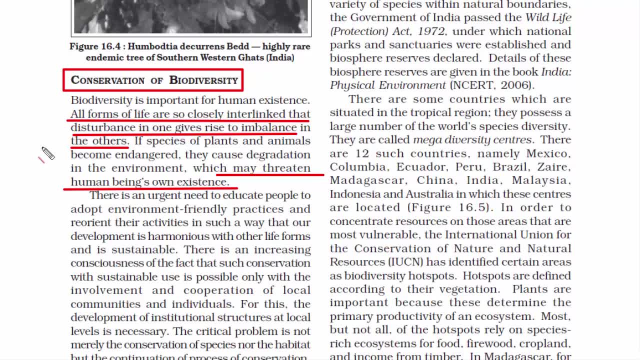 Now, having said all of this, it is clear that human beings are the reason behind a lot of problems in this world, Since we have wants and needs, and it is the earth from which we get all of that. therefore, it is right to say that. 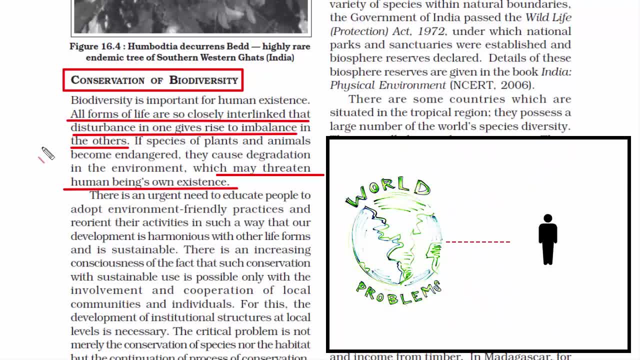 human greed is causing irreparable damage to the environment. Now that we understand that humans are the center of all the problems, therefore, it makes absolute sense to educate people about the environment and how to use it in a sustainable manner To conserve nature. 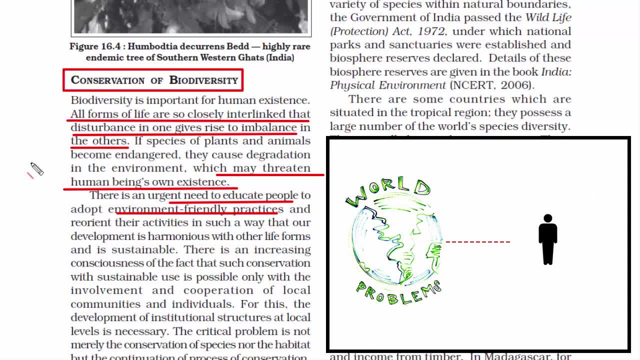 we cannot expect individuals to take any effort. If you remember, Gautam Buddha said: Life is suffering. There's a lot that happens in life and there's nothing wrong with that. When so much goes on in an individual's life, it is senseless to expect anyone to think about nature. 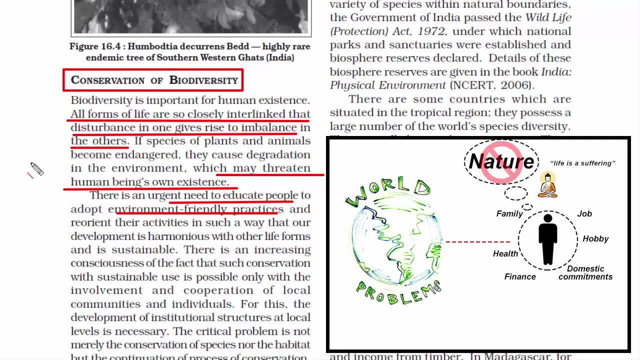 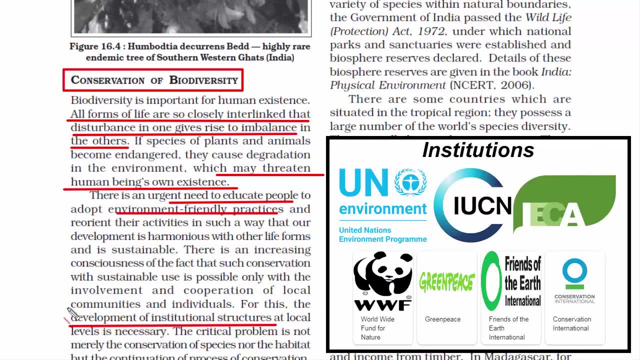 As funny it may sound, the truth is we don't even know how to take care of ourselves. How can we take care of the earth? And that is where institutional structures come into the picture. Institutions come with a set of rules and regulations. 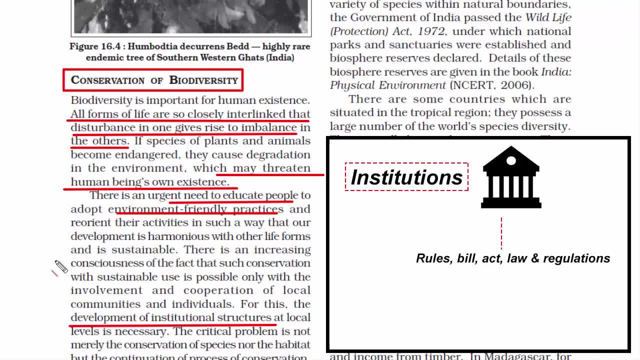 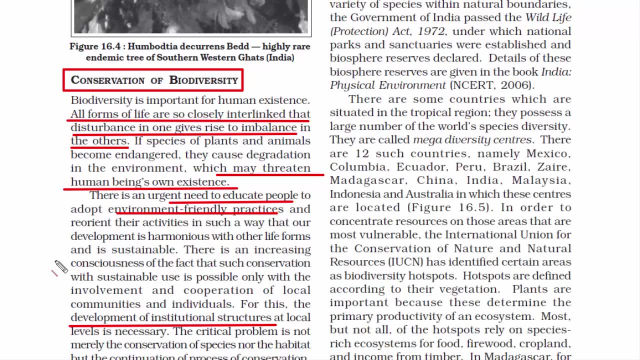 and they ask people to follow them. Institutions can be in the form of government, local bodies. at the community level, even different nations come together to create international agreements. So, basically, institutions are necessary. It brings people together for a common purpose, which is impossible on an individual level. 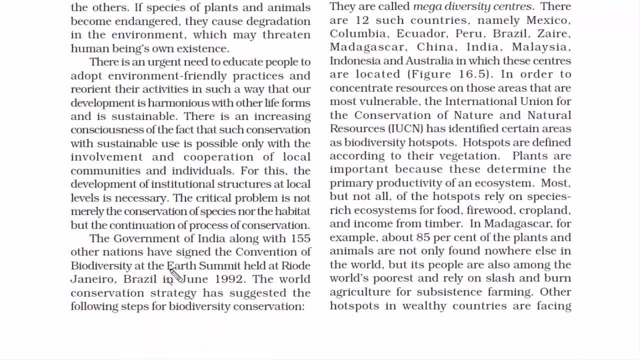 On June 1992, the United Nations had conducted an international conference on environment and development in Rio de Janeiro, Brazil. The name of the conference was the Earth Summit. Some 155 nations, including India, came together and supported the idea of biodiversity conservation. 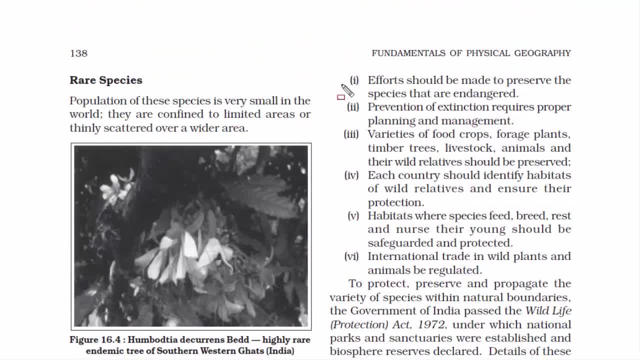 So here's the list of things that they all agreed upon. If you see, all these are guidelines that the government of the member nations have to follow. The whole objective is to preserve animal and plant species from getting extinct, to protect their habitat and environment. 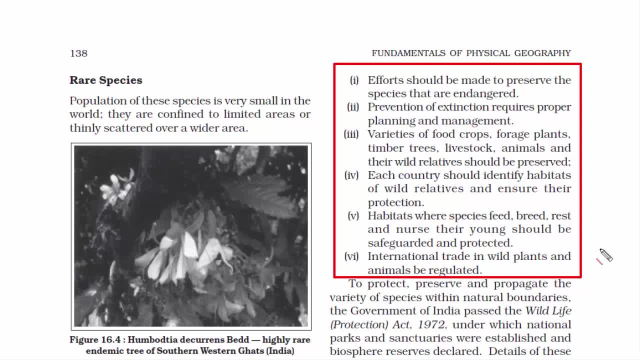 from any kind of human activities like poaching, smuggling, killing, etc. So this is what I meant when I said that you cannot expect an individual to conserve the environment. There have to be institutions that produce laws, guidelines, policies which people have to follow. 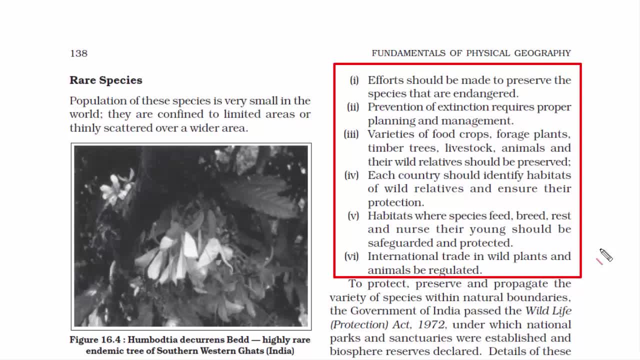 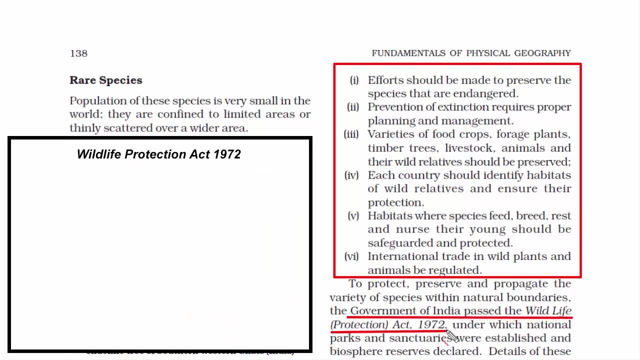 Without law, there is no order. There will be no constructive instrument for a positive social change. So that's why we need institutions to conserve the environment. Similarly, the government of India has passed the Wildlife Protection Act in 1972. The whole purpose behind passing this law. 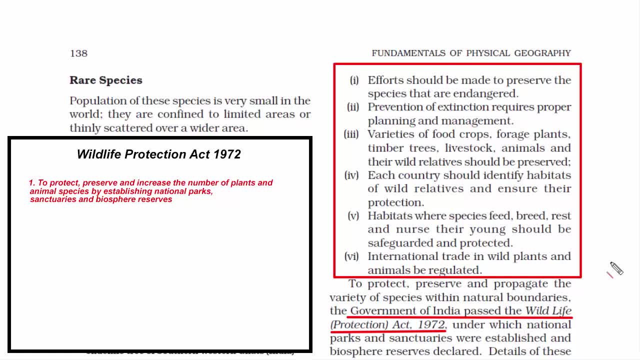 is to protect, preserve and increase the number of plants and animal species by establishing national parks, sanctuaries and biosphere reserves. This law extends to the whole of India, except the state of Jammu and Kashmir, which has its own Wildlife Act. The law also has provisions for penalties. 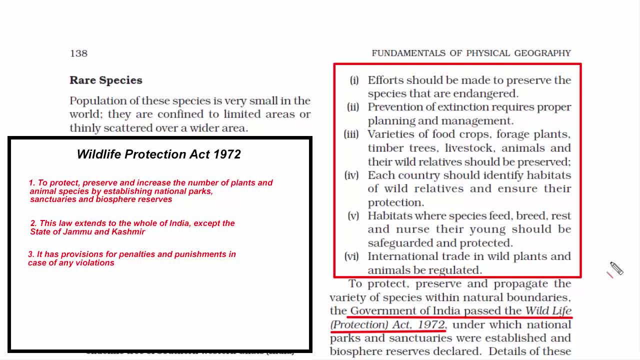 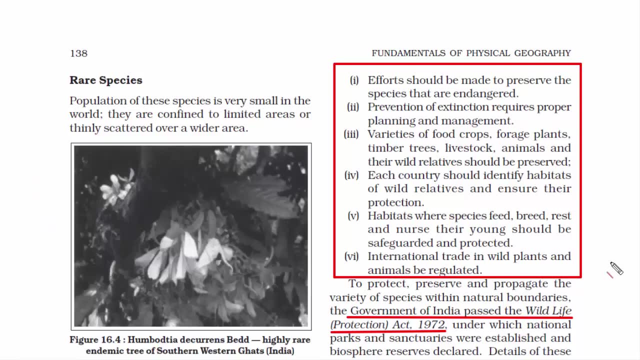 and punishments in case of any violations. The law has been amended 7 times. This means it has been improved or altered from time to time, And that speaks a lot, if not entirely, about the government's intentions about the conservation of biodiversity. I have a separate video where I have 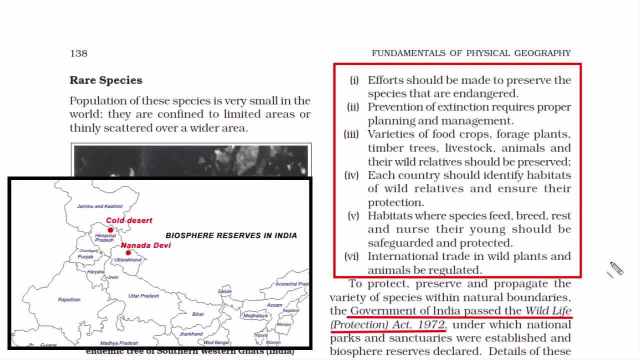 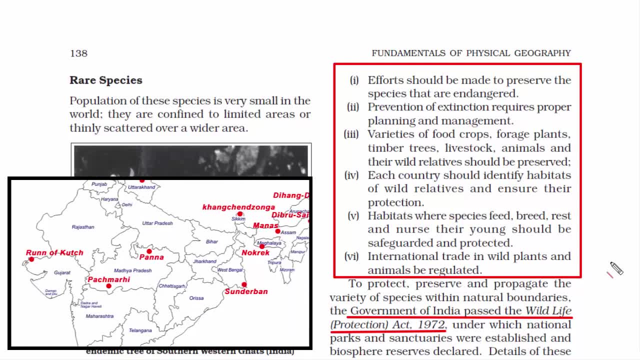 pinpointed all the biosphere reserves that exist in India. The link to that video is in the description. Regarding national parks and wildlife sanctuaries, I still have to make one. Meanwhile, do check the video on biosphere reserves Again. the link is there in the description. 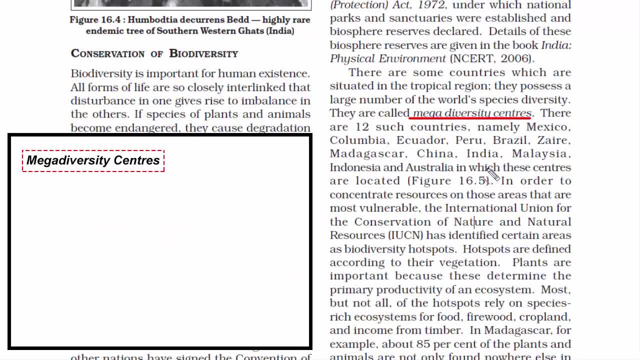 Now there is a term called mega diversity centres. The word mega means large. That means we are talking at the international level. What it means is the countries that have a large number of the world's species diversity are collectively known as mega diversity centres. 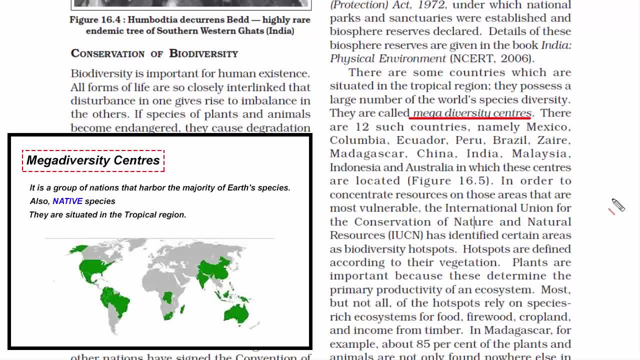 And, coincidentally, these countries are situated in the tropical region. In a nutshell, the mega diverse countries are those countries that are home to a majority of the earth's species and are therefore considered extremely biodiverse. Initially, there were 12 such countries, Presently it's 18, and they are: 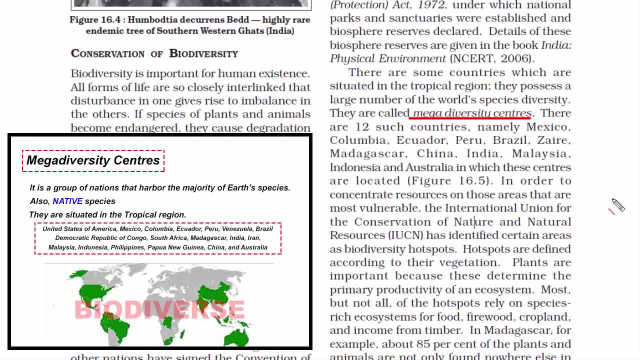 United States of America, Mexico, Colombia, Ecuador, Peru, Venezuela, Brazil, Democratic Republic of Congo, South Africa, Madagascar, India, Iran, Malaysia, Indonesia, Philippines, New Guinea, China and Australia. These 18 countries meet for consultation and cooperation. 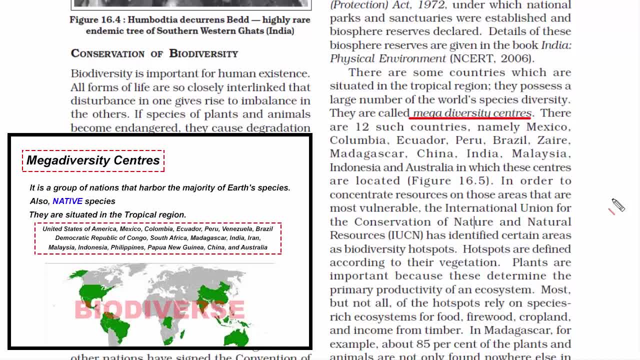 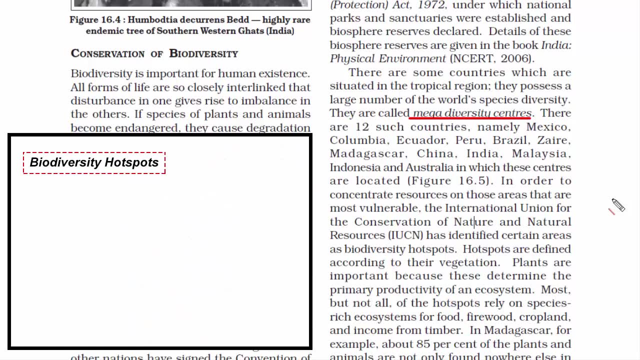 related to the preservation and sustainable use of biological diversity, So these countries are collectively called mega diverse countries or mega diverse centres of the world. However, don't confuse it with biodiversity hotspots. If you look at the biodiversity hotspots of the world, they also exist. 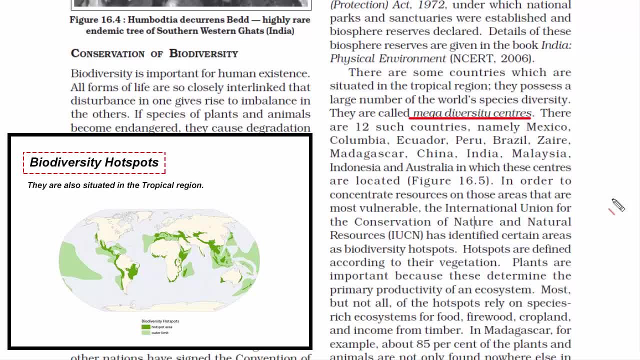 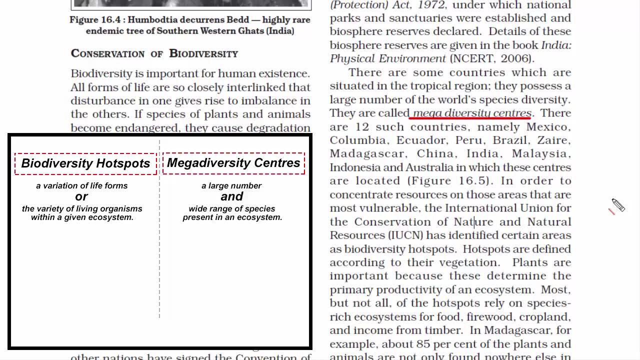 in the tropical region. But the subtle difference between biodiversity and mega diversity is that biodiversity means the variation of life forms or the variety of living organisms within a given ecosystem, And mega diversity means a large number and wide range of species present in an ecosystem. 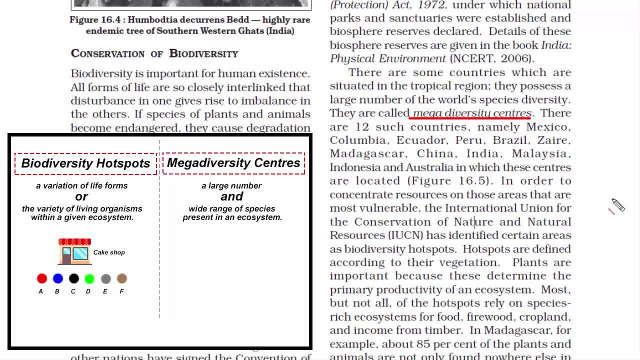 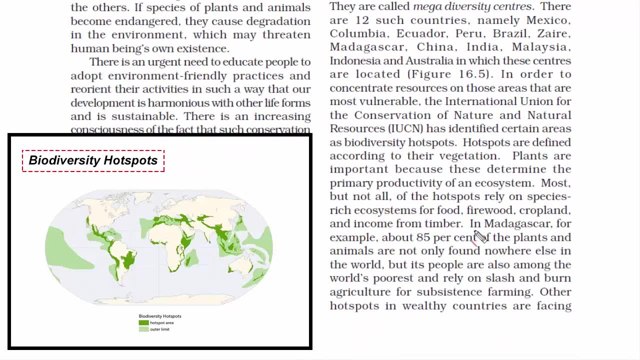 In simple terms: biodiversity is like a shop that has a different variety of cakes, And mega diversity is like a shop that has different variety as well as a large number of cakes. I hope you get the difference between the two. And the last thing is all these biodiversity. 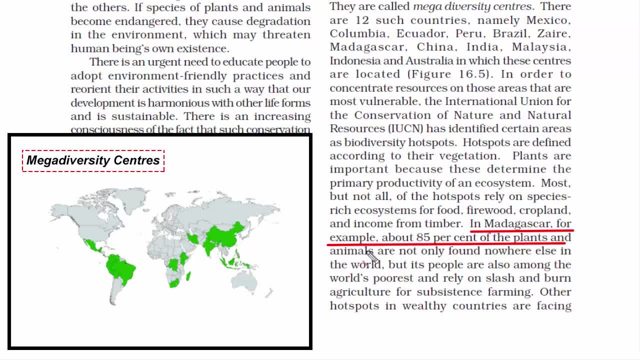 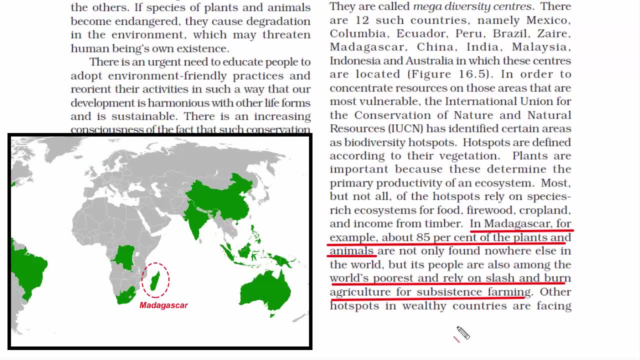 hotspots and mega diversity centres that you just saw moments back. they all are facing different kinds of environmental challenges. Some regions are facing an extreme loss of biodiversity due to the habits of the native people. For example, here it says: in Madagascar, about 85% of the plants and animals. 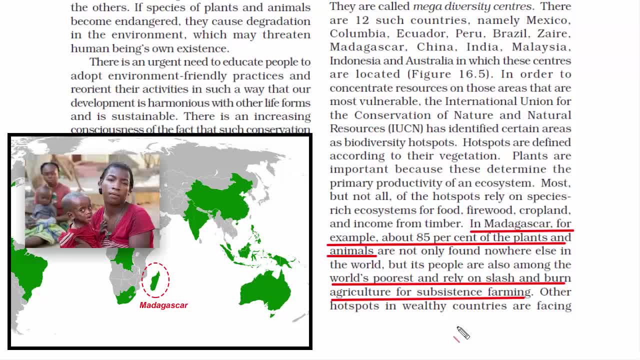 are so rare in the world, but its people are also among the world's poorest and rely on slash and burn agriculture for subsistence farming. I hope you know what is slash and burn agriculture. It is a method that involves the cutting and burning of plants. 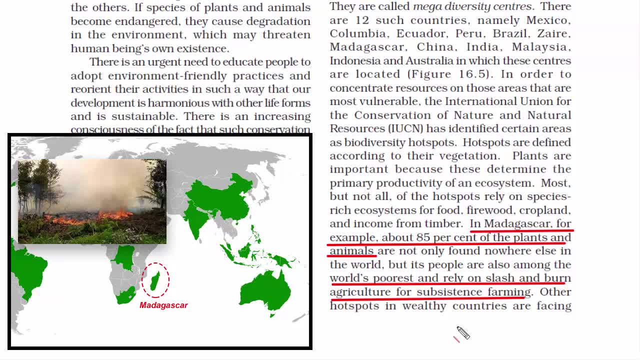 in a forest to create an irrigation field to grow crops. You see, there are two sets of problems. On one hand, these local people need food and they have to grow it, And on the other hand, to grow food they need land, and for that 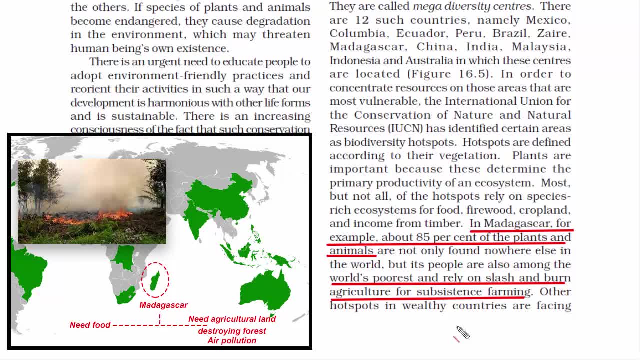 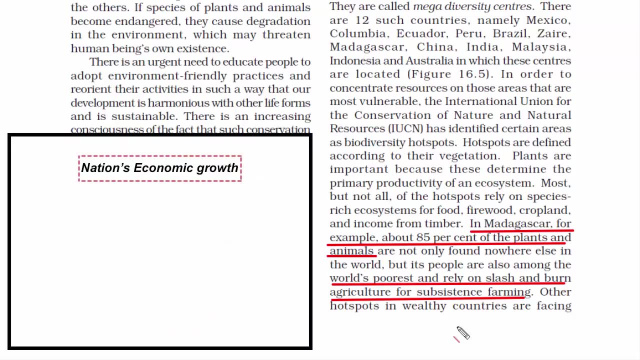 they are destroying the forest, and the smoke from the fire will cause air pollution. Anyhow, if you look at the technique, it can be compared to deforestation, and this process has a dramatic effect on the ecosystem. Now, if you look at the wealthy nations, what do you think? 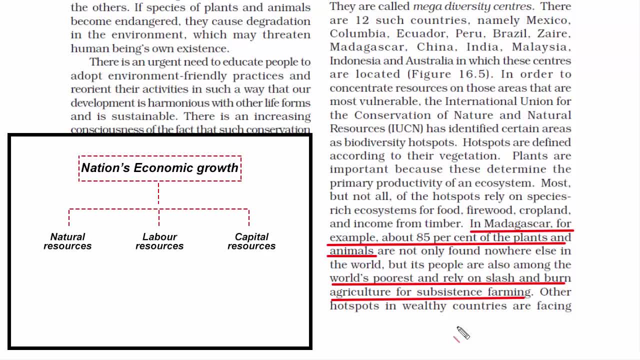 are the key drivers for a nation's growth. They are natural resources, labour resources and capital resources. If you focus on natural resources, you will realise that today, about 80% of the world's energy consumption is sustained by the extraction of fossil fuels, which consists of oil, coal, 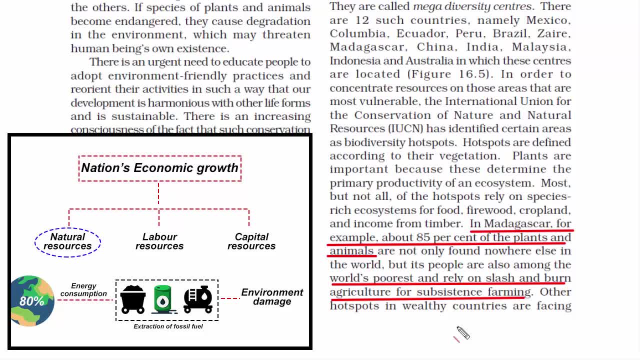 and gas. The extraction as well as the usage of fossil fuel both causes great environmental damage. However, at present we cannot move away completely from fossil fuels. The world economy heavily depends on the oil and fuel industry. You see, this is another set of problems. 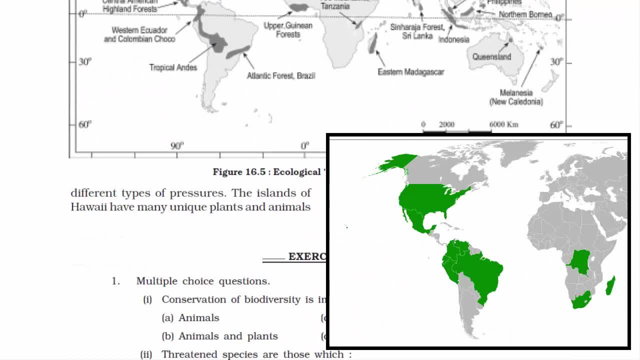 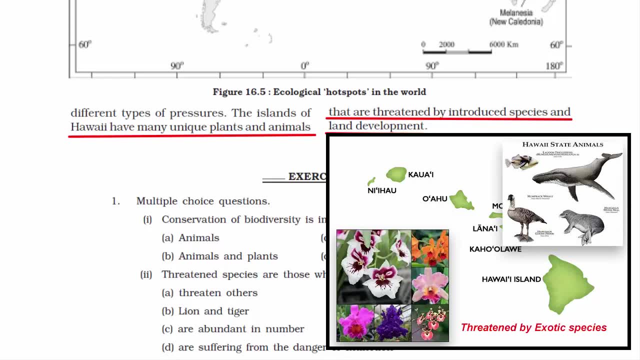 And the third set of problems is in some places, for example the islands of Hawaii. here the native plant and animal species are threatened by foreign or exotic species. These foreign, alien or exotic species of plants and animals and other organisms are a big threat to the Hawaiian ecosystem. 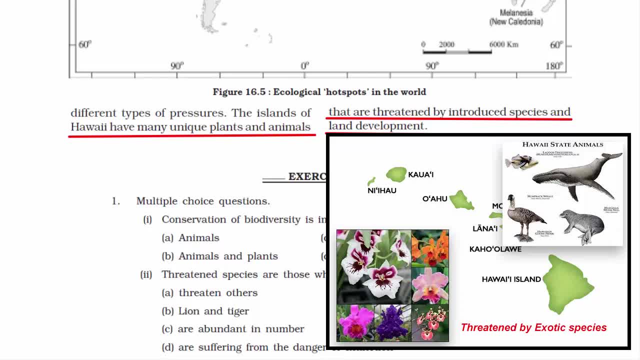 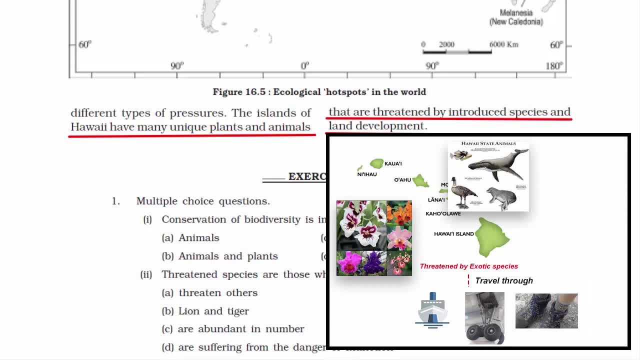 You must be thinking: how did they arrive on the island of Hawaii? It all happened when new forms of plants were introduced. Sometimes it is accidental when foreign insects and animals travel through cargo ship, through the wheel, well, of an aircraft, and there are some other surprising.